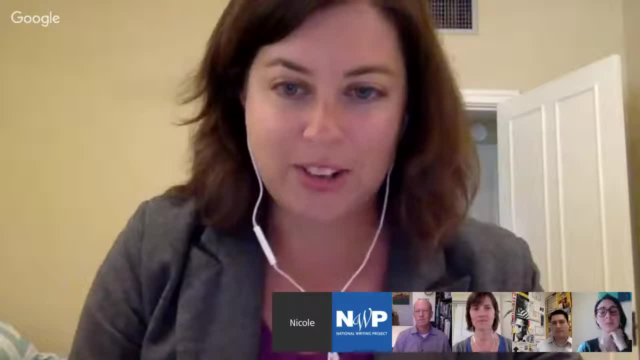 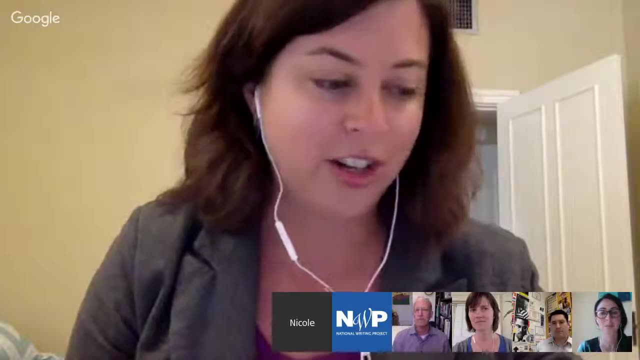 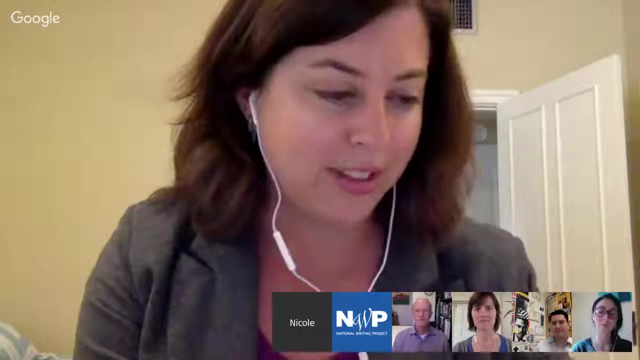 at the University of Texas at El Paso. I earned my PhD in Urban Schooling from the UCLA Graduate School of Education and Information Studies And I'm also a former high school English teacher and coordinator of the UCLA Council of Youth Research. Before we dive into our conversation, let's go over a couple of quick details To those. 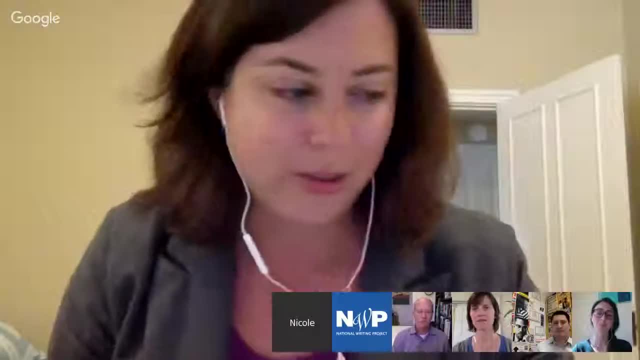 of you watching live right now. we welcome your comments and questions through either the Twitter hashtags- hashtag youth research or on Twitter at youthresearchcom, And. I'm also a former high school English teacher and coordinator of the UCLA Council of Youth Research. 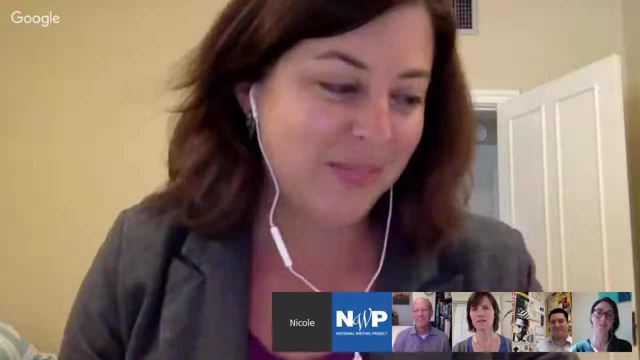 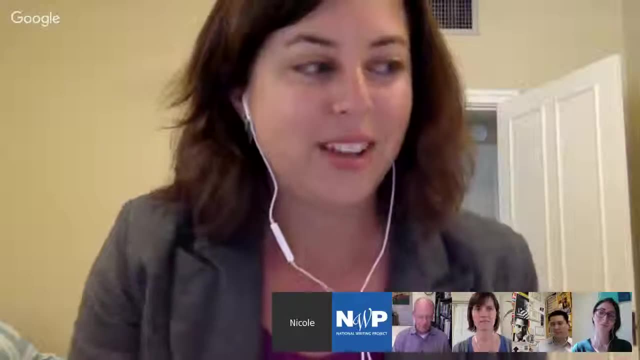 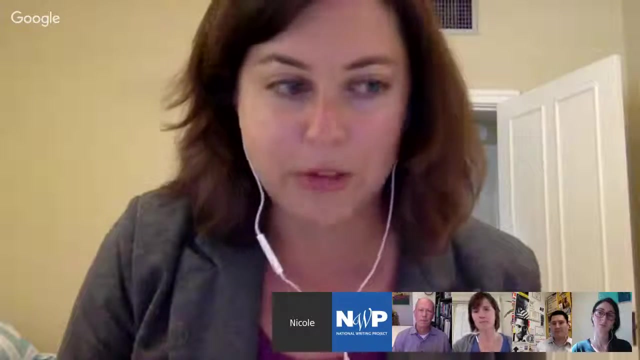 To those of you watching live. do not miss out onists phrase, hashtag connected learning or hashtag digital civics, or the Q&A feature that you should see in your video player. We'll do our best to address your questions here in the Google hangout. 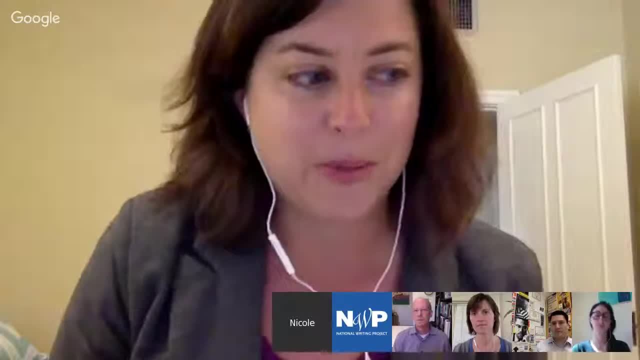 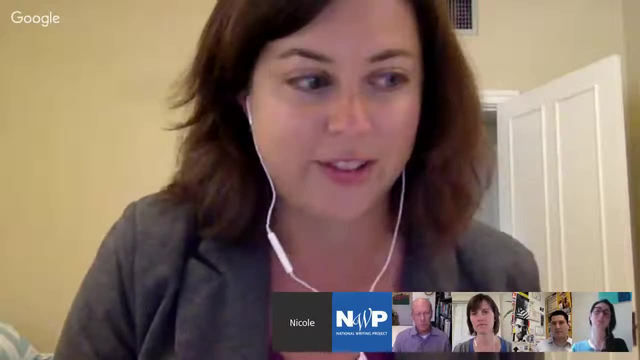 The Webinar is also being costreamed at the National Writing Project's EducatorInnovator org and is part of a series of software related to letters to the next president 2.0, which engages and connects young people ages 13 to 18 as they research, write and make media. 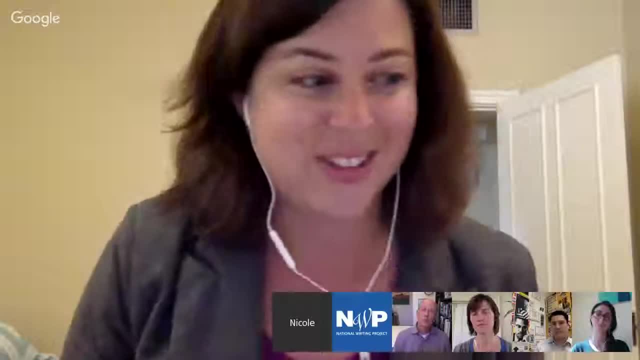 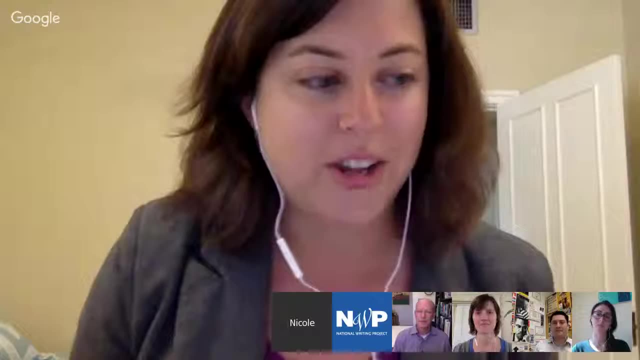 As such. you can also use the hashtag 2nextprez if you'd like to engage that way. This webinar will be available as a resource on letterstopresidentorg, where you can find many other resources and opportunities related to the election, writing and digital literacies. 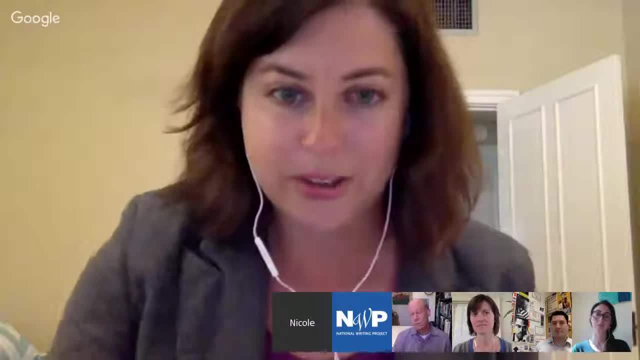 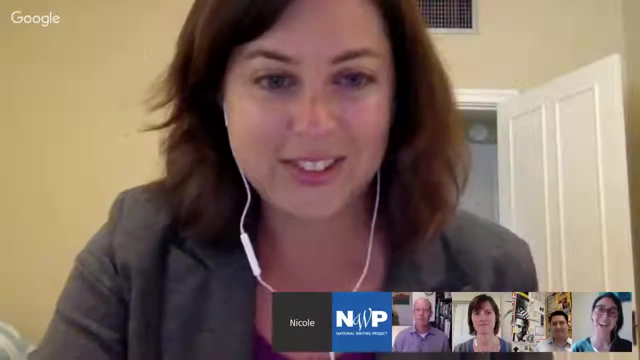 So now, before we get started, let's give everyone a chance to introduce themselves. So I'm just going to go down the line that I see on the bottom of my screen. So, if we can start with Perry Perry, You might want to unmute yourself first. I do that all the time. 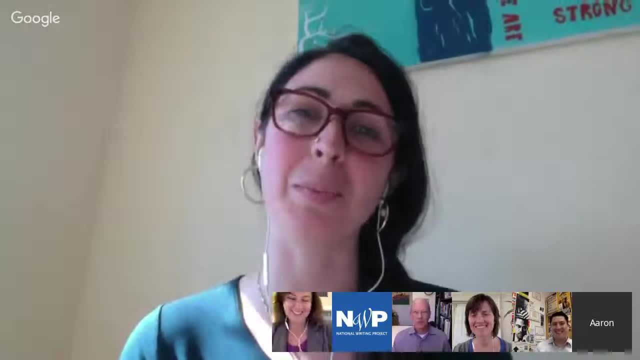 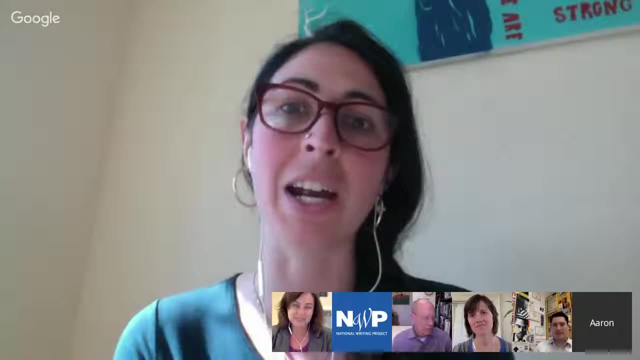 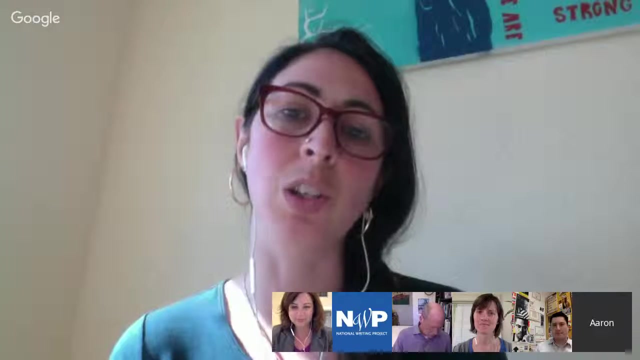 Sorry about that. My name is Perry Bellow-Hanselman. I'm a teacher at Coliseum College Prep Academy. I've been teaching there for five years and eight years in Oakland, Unified in various capacities, And I currently run our social justice pathway at the school and teach ethnic studies and civic engagement. 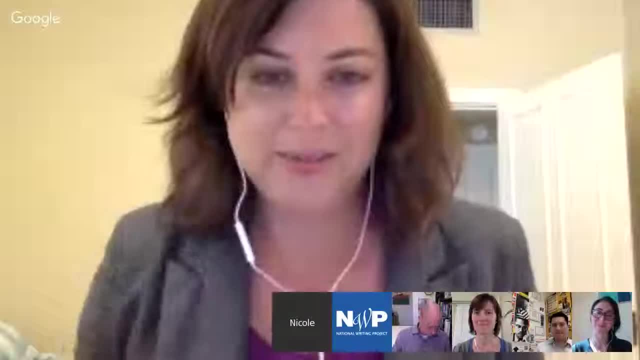 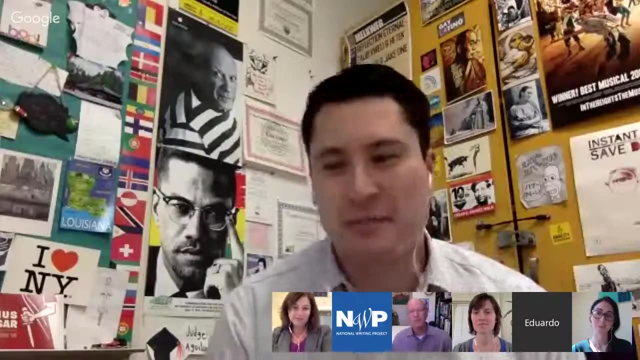 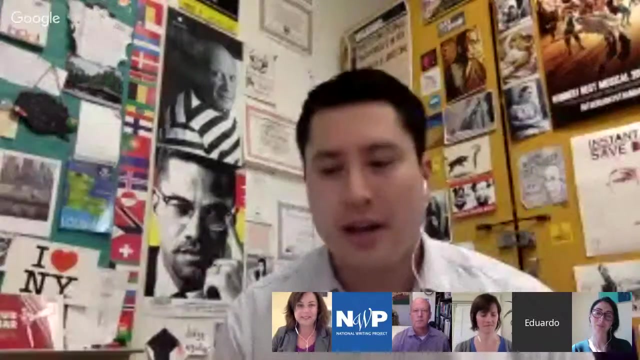 Awesome, Eddie. Hi, My name is Eddie Lopez. I teach at Roosevelt High School, located in Boyle Heights in East Los Angeles. I've been teaching for 11 years. I'm a social studies teacher, So currently I am teaching an ethnic studies course for Latino males. 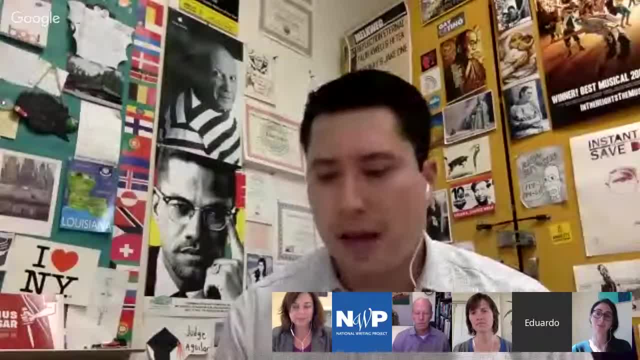 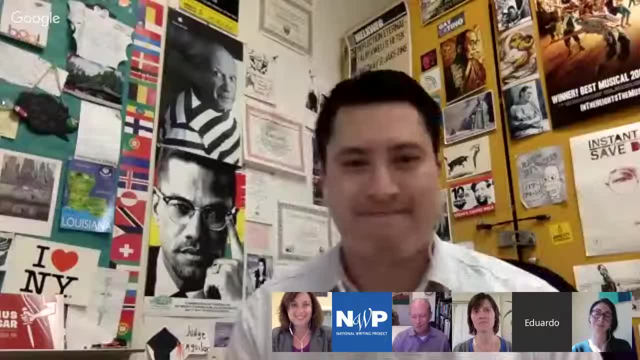 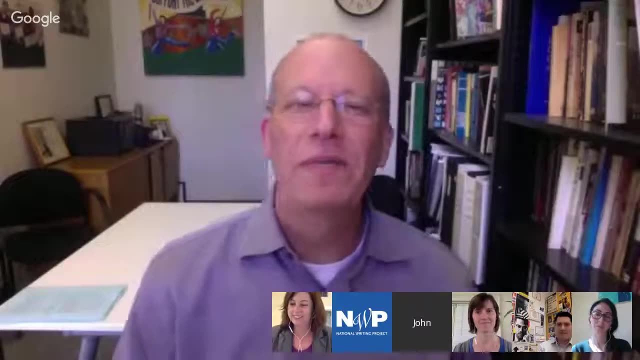 The program is called Urban Scholar Compadres and US History And I've worked with many of the folks on the panel, with the Council of Youth Research And, last but not least, John. Good afternoon everybody. My name is John Rogers. 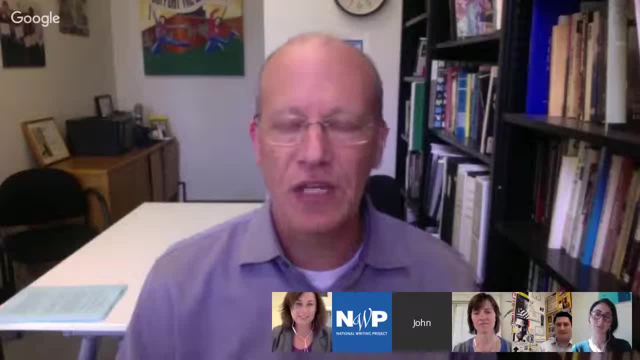 I'm a professor at UCLA in the School of Education and Information Studies. I'm also affiliated with two centers. One is the Institute for Democracy, Education and Access, or IDEA, And the other is Center X. that houses our teacher education program and our principal's program as well. 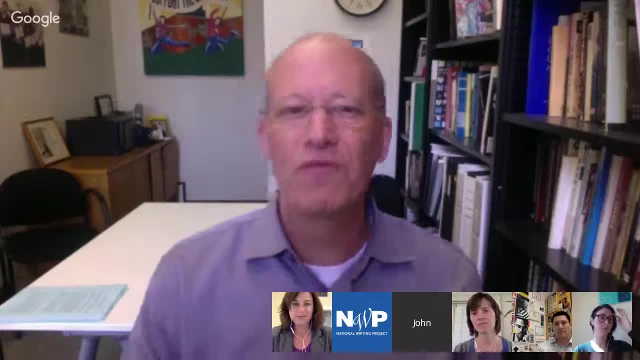 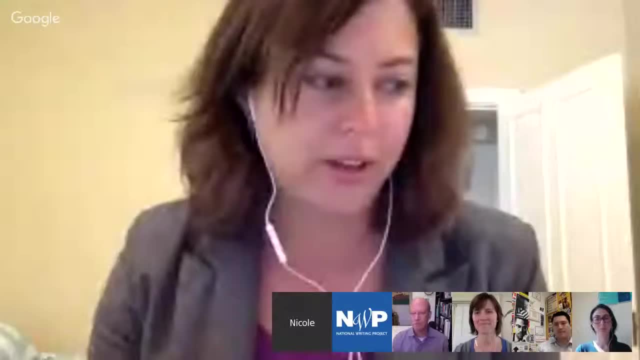 IDEA was the center out of which the Council of Youth Research was founded, And it's the center that I'm currently working on And that's where the Council of Youth Research emerged. Awesome, And I think now we're going to before we start the conversation, in case there's folks that are just coming into the webinar. 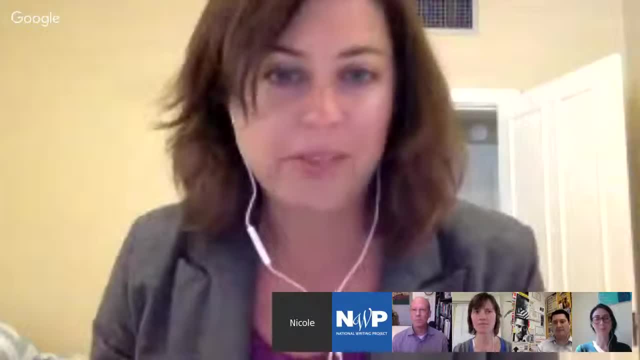 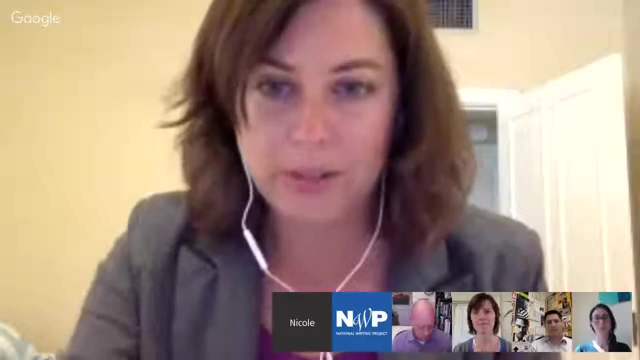 and haven't had a chance to get to see what we've done over the past month. we wanted to talk about the two projects that our groups are coming from. So, Erica, if you want to start off giving us a little description of EPP, 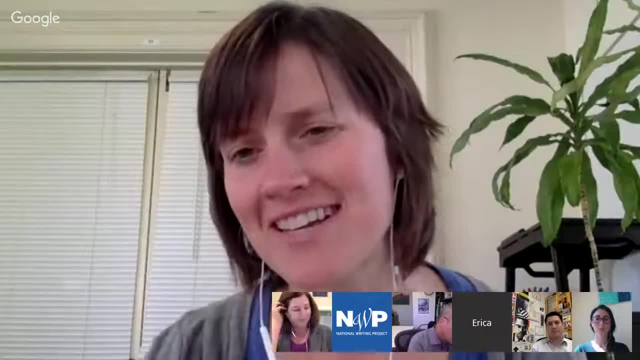 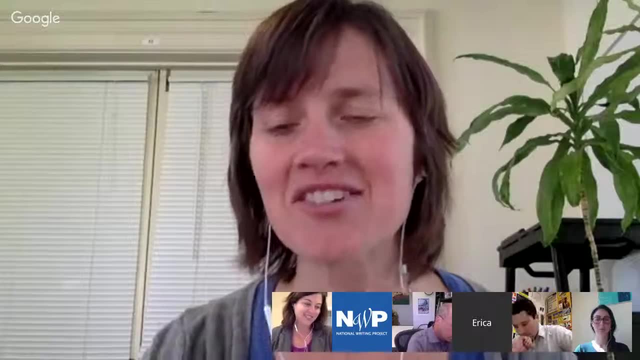 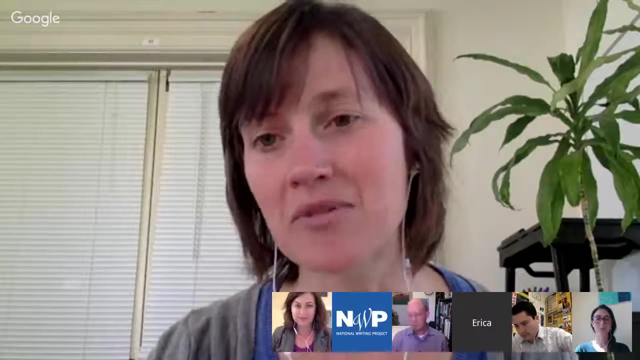 Sounds great. So the EPP project, because I know there are so many acronyms. the EPP project stands for Educating for Participatory Politics, which is actually an action project based out of the MacArthur Research Network on Youth and Participatory Politics. 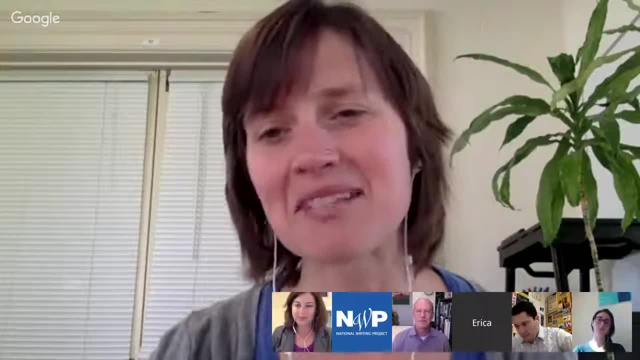 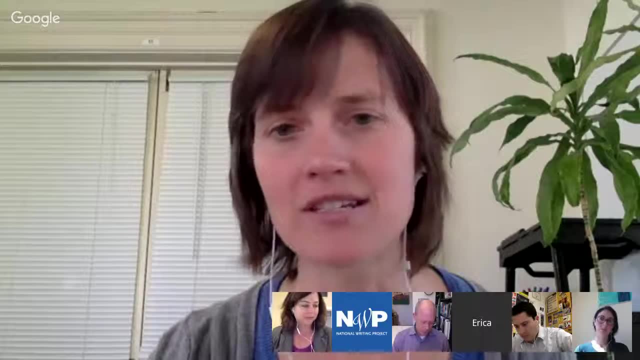 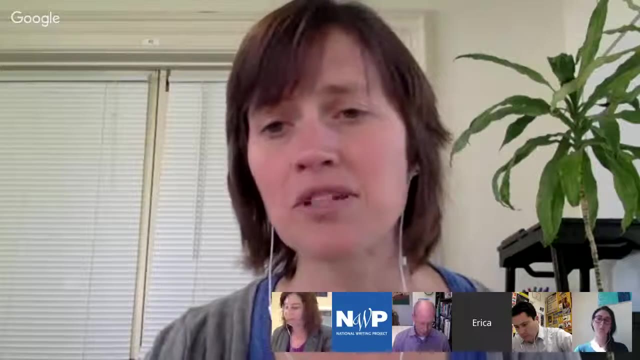 So the YPP- another acronym Research Network- has been studying youth civic and political development and participation in the digital age over the last five or six years through various research studies and research teams across the country, And we've been really focusing on the affordances of digital media. 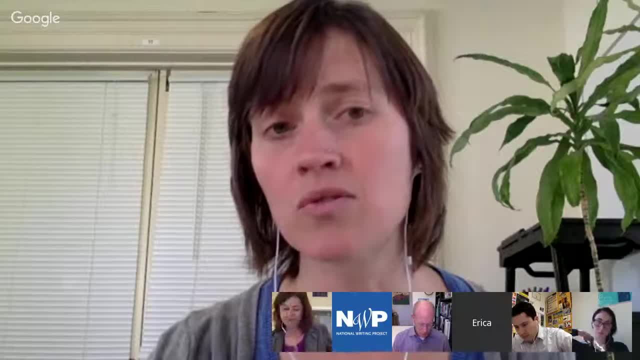 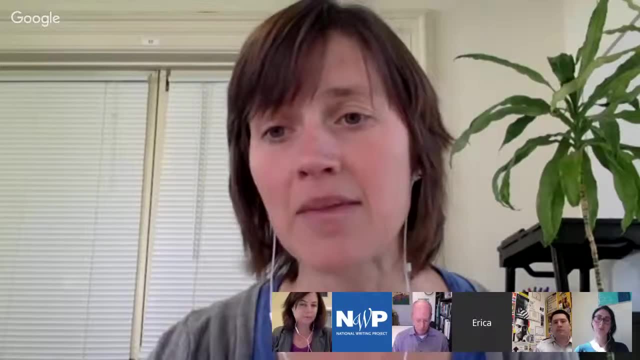 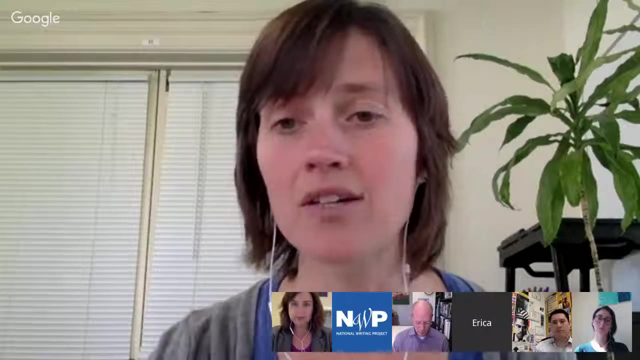 and how those have created more opportunities for youth to engage in what we call participatory politics, which are actions that either individuals or groups take part in to either get their voice out there or to influence issues of public concern. So that could be investigating issues, promoting dialogue or giving feedback. 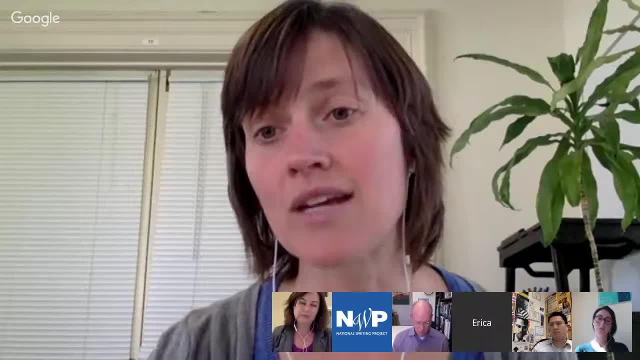 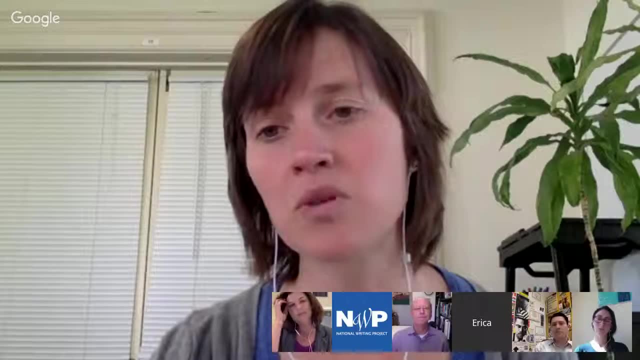 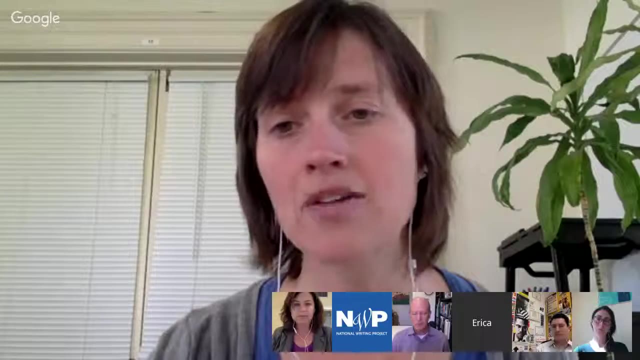 impacting cultural norms or mobilizing others to get involved in issues that matter to young people. So, drawing on this research, the EPP project has been working with educators and youth to develop a framework of core practices of participatory politics and also pilot educational resources that articulate a sort of new vision for civic education. 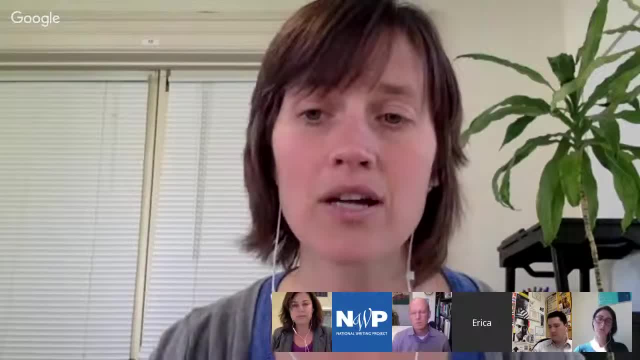 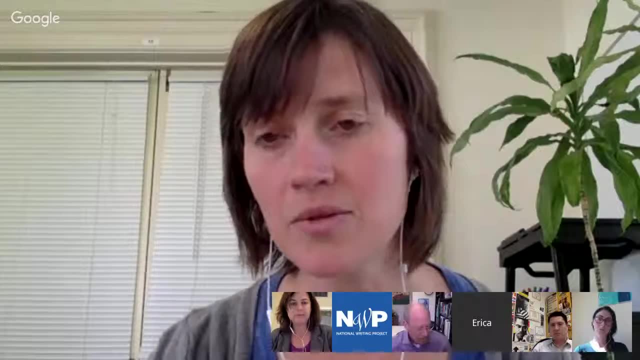 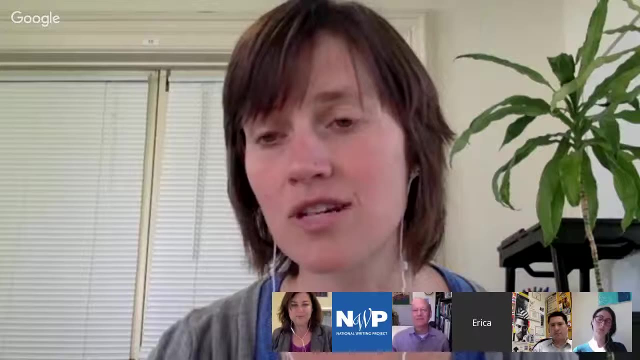 and this changing landscape. So the EPP project is a combination of different teams. We have a team of folks in Los Angeles. We also have two teams that have been working in Chicago through the Black Youth Project and also through Facing History and Ourselves. 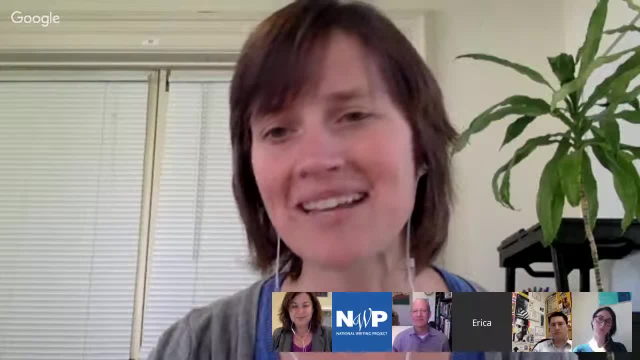 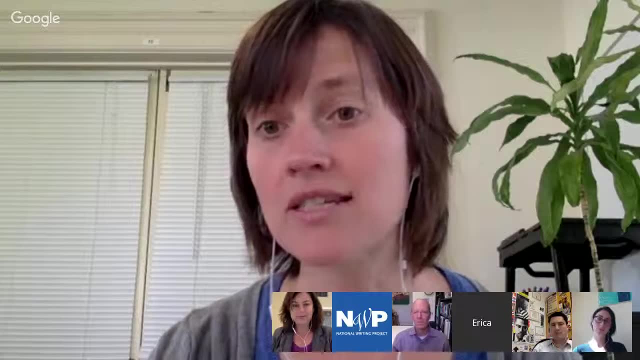 And then we have a team in Oakland. So I'm really excited that Perry can join us from our project in Oakland, And in Oakland the project is called Educating for Democracy in the Digital Age, And this project is taking a little bit of a different approach and working with the entire school district. 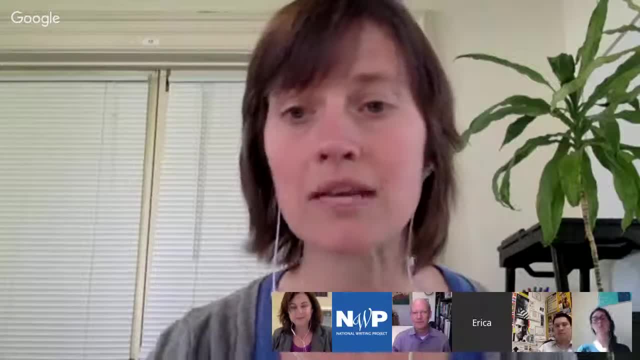 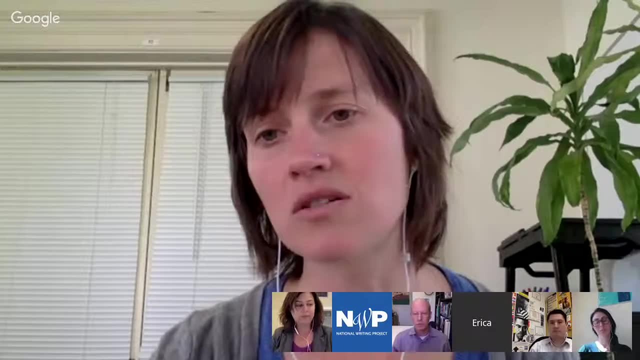 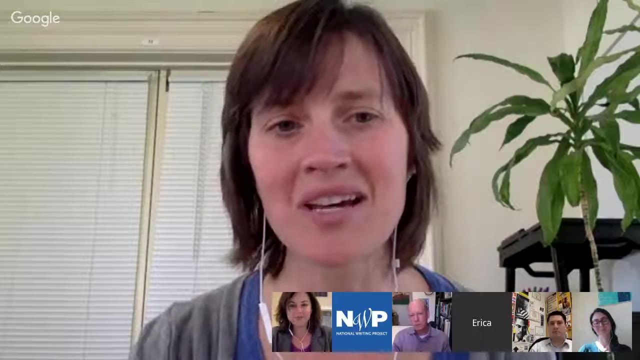 So not only are we working with teacher leaders like Perry, but at the same time, we're also working with the district to try to align civic engagement and also digital literacies alongside of the sort of priorities that the district is focusing on. So I'm excited to talk a little bit more about that project, alongside of the Council of Youth Research. 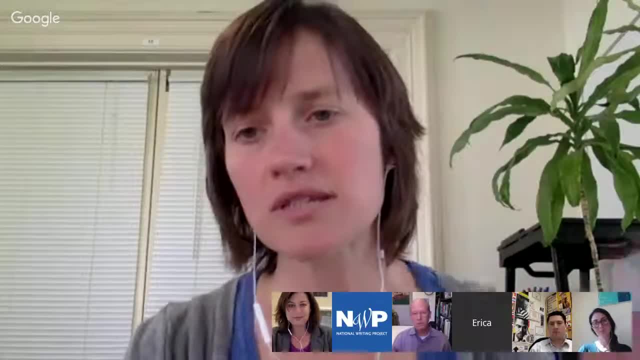 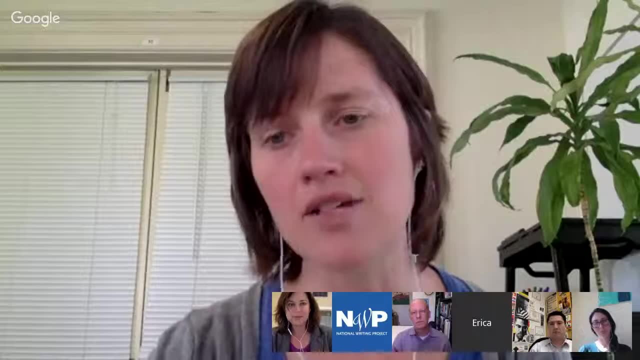 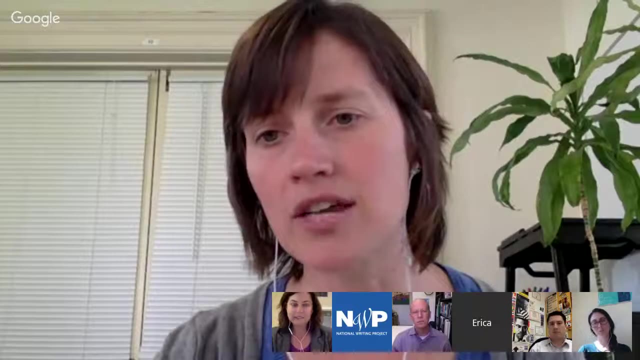 I want to add in one last thing, which is just that these resources that have been developed by the different EPP teams are now available online through a collection, a sort of curated collection of resources. And so if you go to yppdmlcentralnet and click on Educators- at the top of the screen- 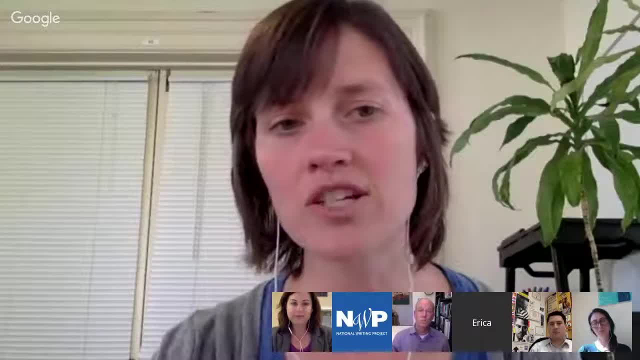 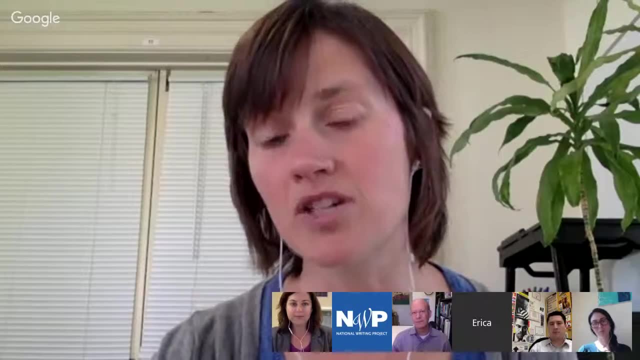 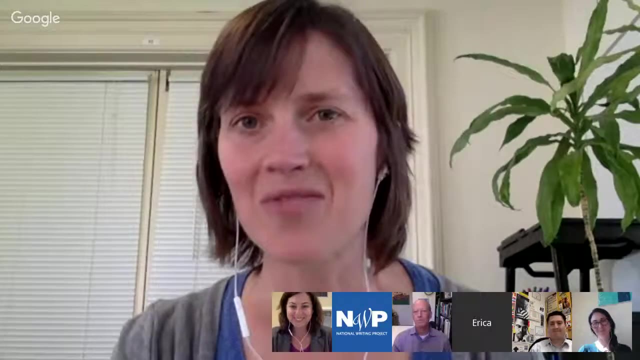 those resources are included there under each project and that's curriculum that's been developed by teachers and also implemented in the field, as well as blog posts by educators and members of the team, sort of reflecting on doing this work. So I'll turn it back over to Nicole to give the overview of your project. 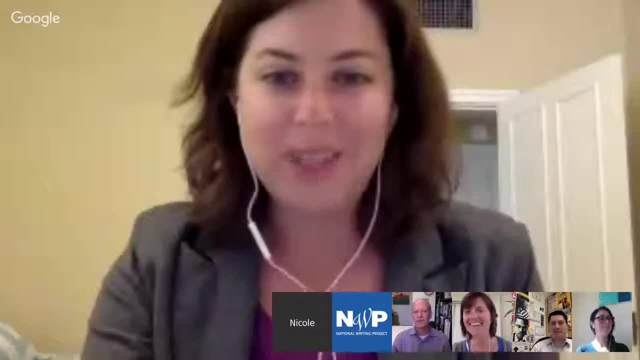 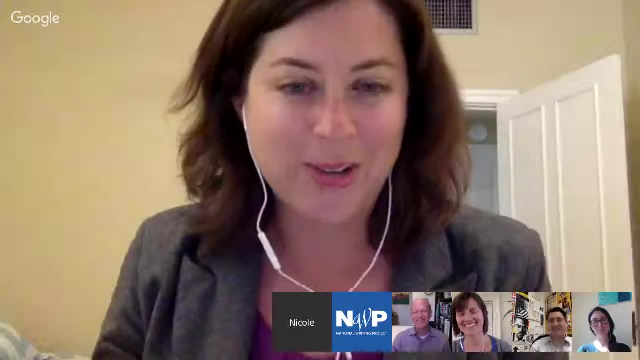 Sure, And just to confuse everyone even more, we are not the Los Angeles team of the EPP network, even though I feel like our work has so many parallels to each other and I think we have a lot of great connections to talk about. 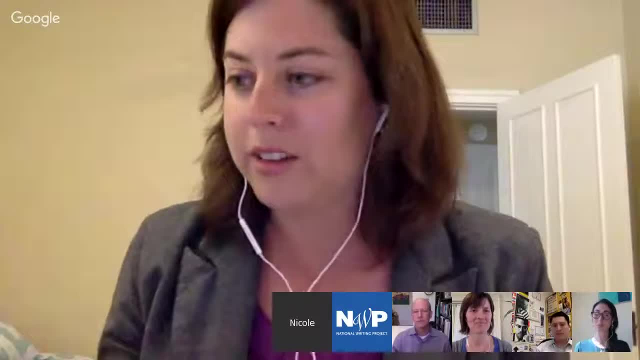 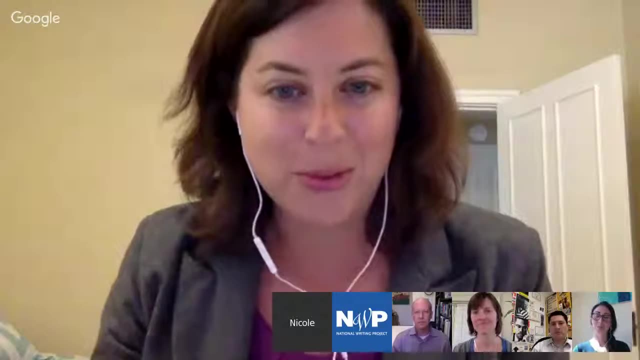 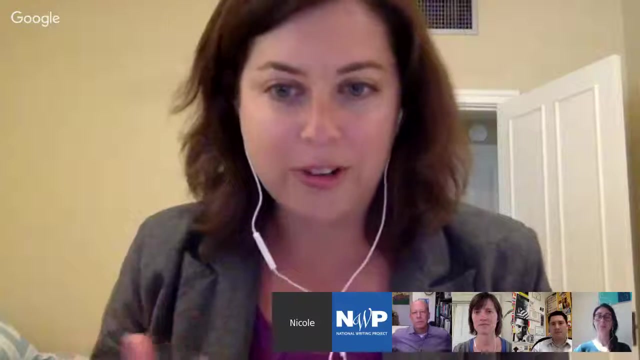 But in a summary, the UCLA Council of Youth Research is a YPAR program, another acronym which stands for Youth Participatory Action, Research At its most basic level, it's about transforming who does research, obviously introducing youth, introducing young people to the project. 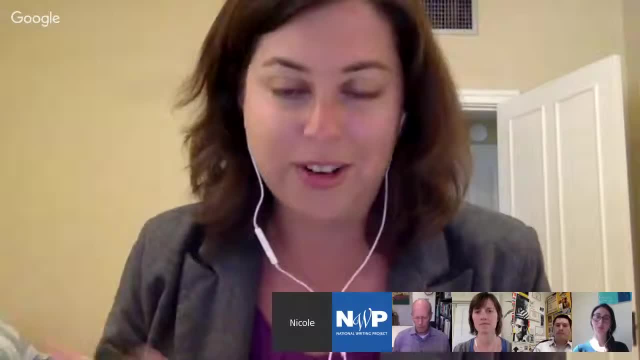 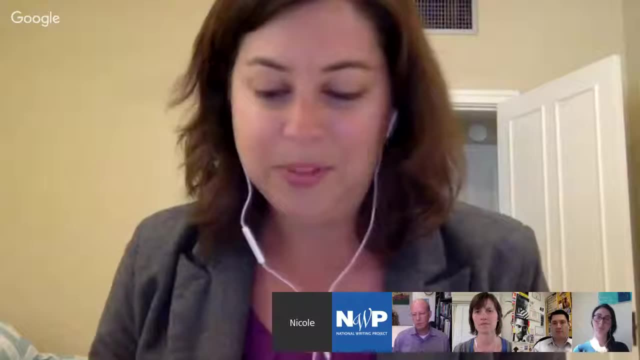 how we do research which is in a participatory, inclusive fashion, and why we do research which is to create social action and fight for social justice, with young people as our leaders. So our project is unique because it is an out-of-school project. 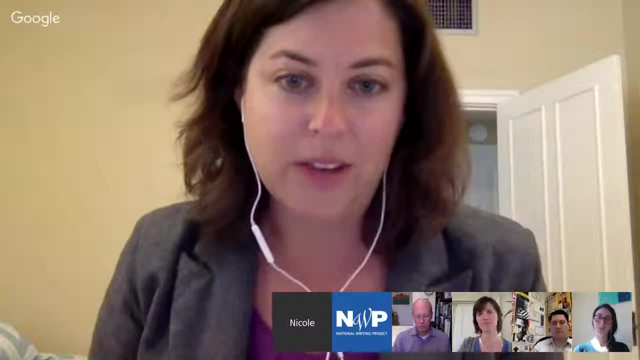 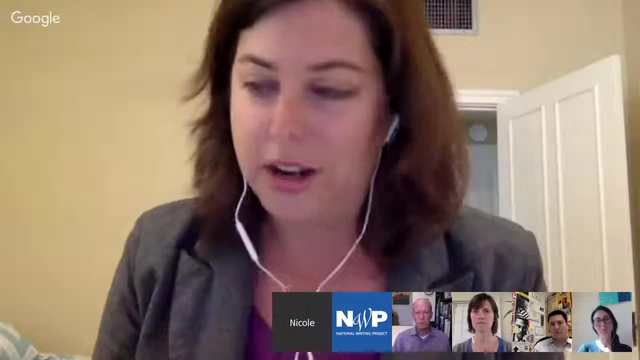 but, as you'll see when we talk to Eddie and many of the folks in our network have actually transformed this work and brought it into the classroom space as well: Dr Rogers, John and Ernest Murrell back in the 1990s- 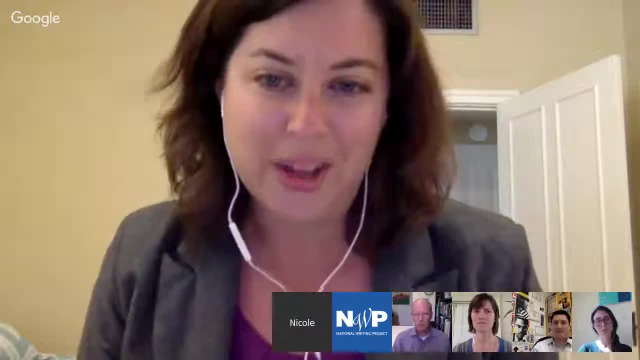 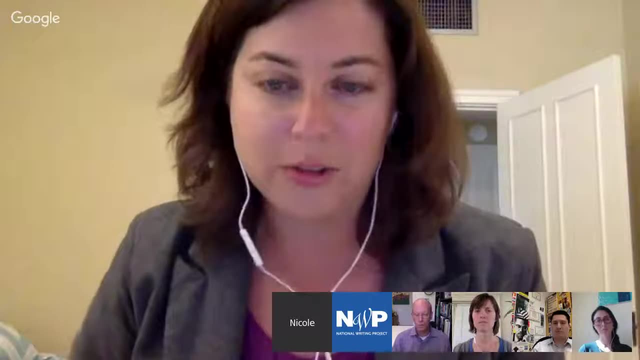 back in 1997, started what became the Council of Youth Research. when they worked with Santa Monica High School, They were asked to come in and do an evaluation of some of the issues the school was facing and they thought that maybe, instead of talking to researchers about it, 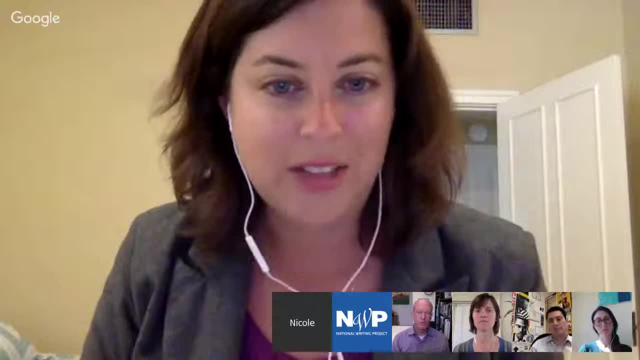 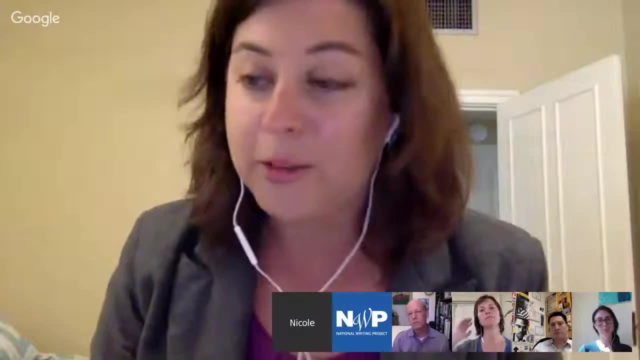 we should talk to the young people who are there every day at the school site. And from that point we kind of expanded to five different high schools in South and East Los Angeles, And now it's been generations of students that have come through our project. 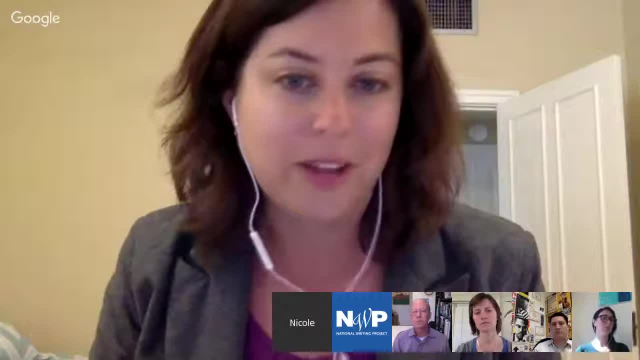 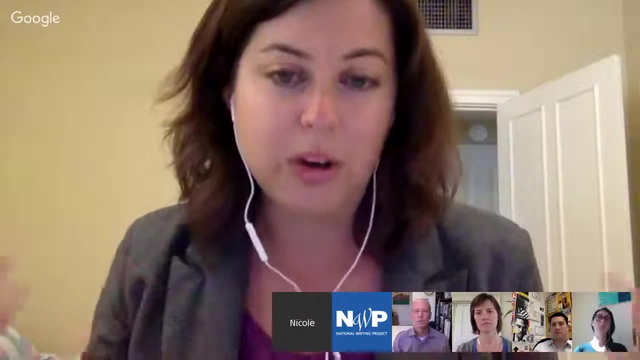 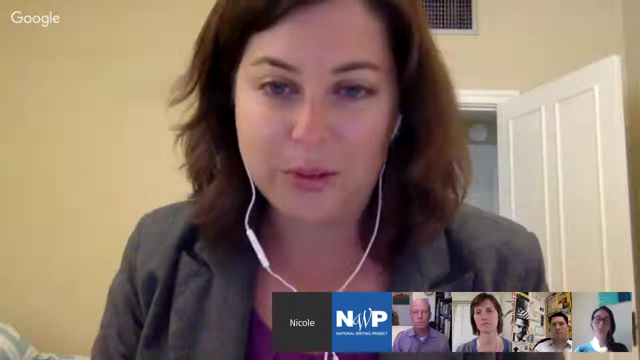 who meet after school and meet once a month at UCLA, And meet over the summer for five-week sessions to create multimedia projects exploring research questions of their own creation about the issues and challenges they see in their schools and communities. We've been lucky enough to bring our youth to academic conferences. 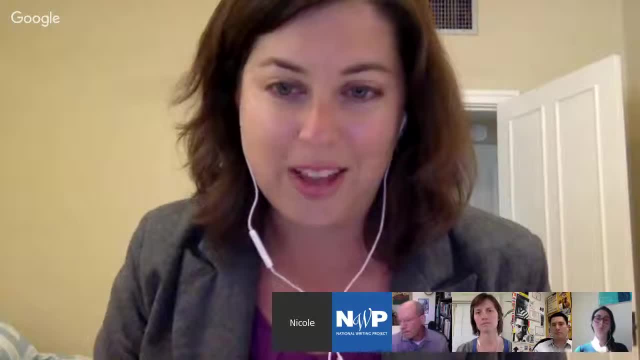 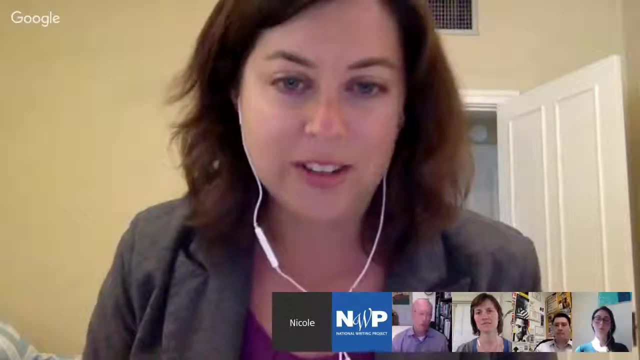 so that they can present to adult researchers, so they can show that they can speak for themselves instead of always having adults speak for them. And their work is available online and we'll be spreading links so that everyone can see some of the multimedia projects that they've been doing. 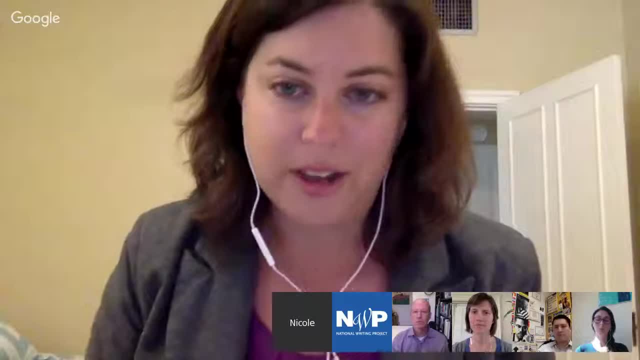 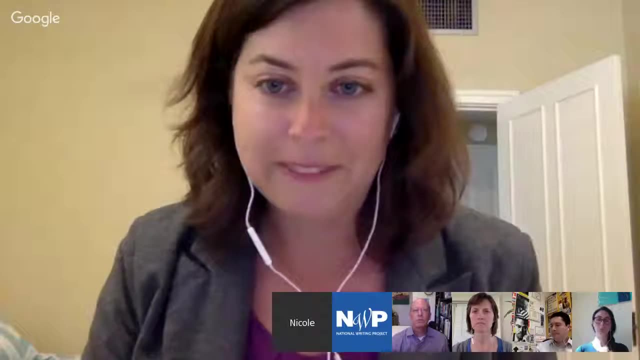 But one of the things that we'll talk about as we move forward is kind of how the in-school and out-of-school environment mesh when we talk about civic education and digital civics. So I'll stop there for now, so that we can jump right into our discussion. 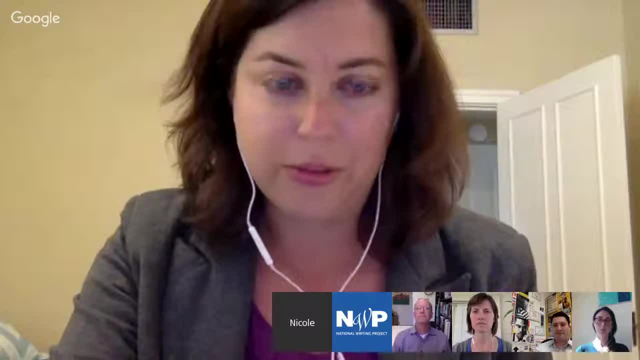 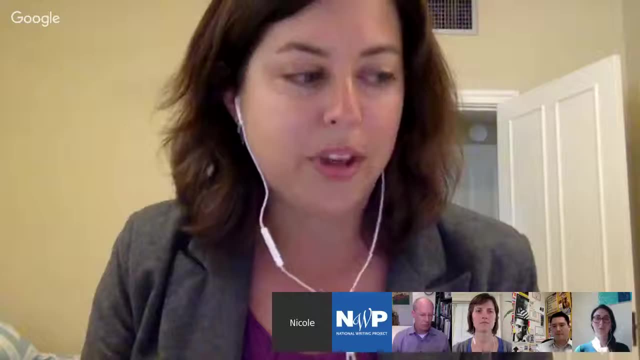 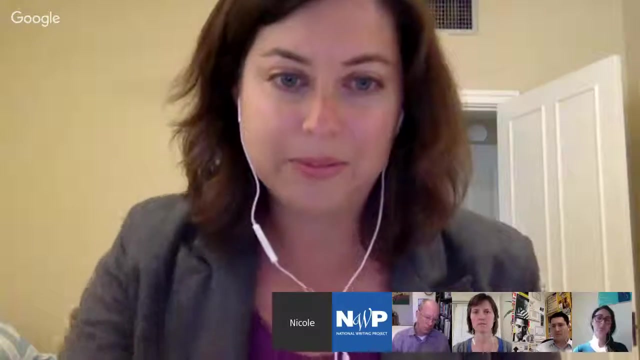 And I want to start with a question for all of our panel. Maybe we can start with our teachers first. I'm wondering if you could speak to how you think educators can use digital tools to connect students to authentic audiences and to civic issues. So maybe we can have Perry and Eddie start us off. 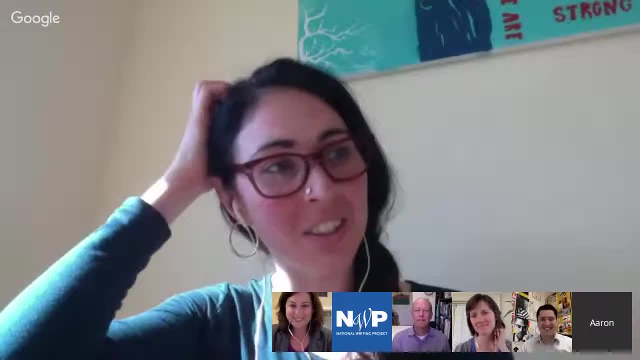 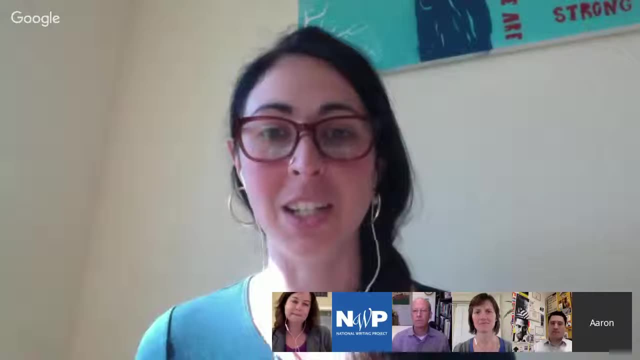 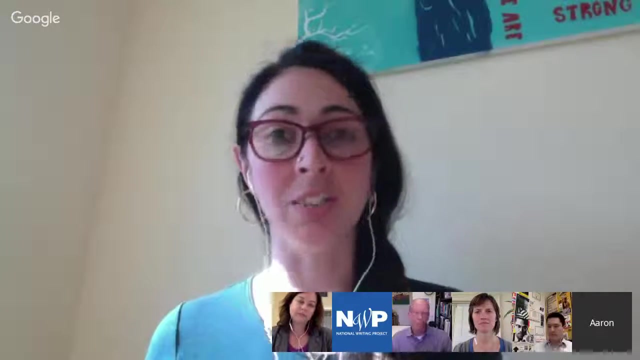 Oh, am I starting? It's an interesting question and I've experimented in different forms with it Because one of the questions is around authenticity. I've had students in the writing that they've done in my class. really look at this year, for example. 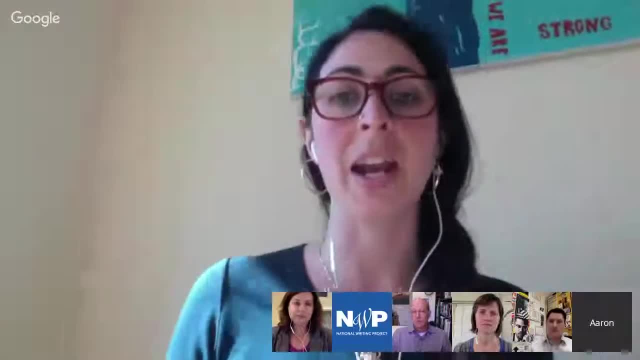 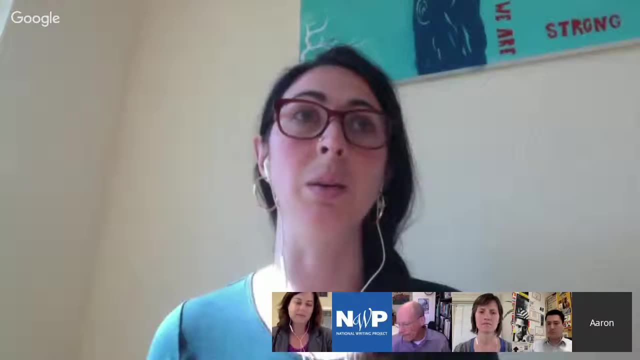 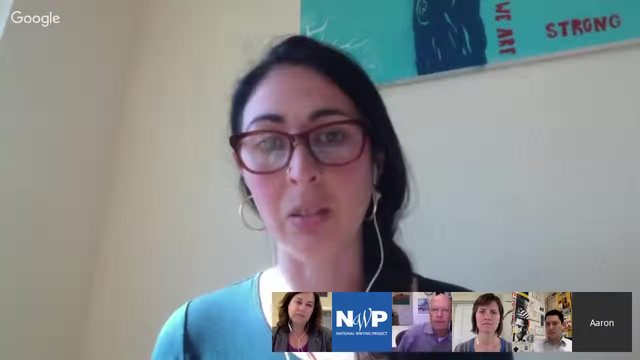 we've been experimenting with putting our writing on blogs and always having an audience in mind when we're writing about the issues that we're exploring in the classroom. So we're talking about systems of oppression, We're talking about the prison industrial complex. We're talking about active movements that are happening right now. 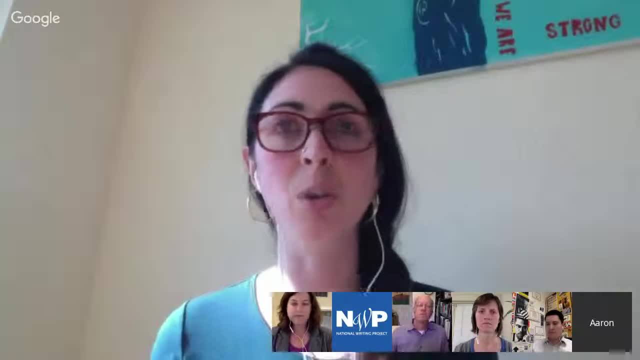 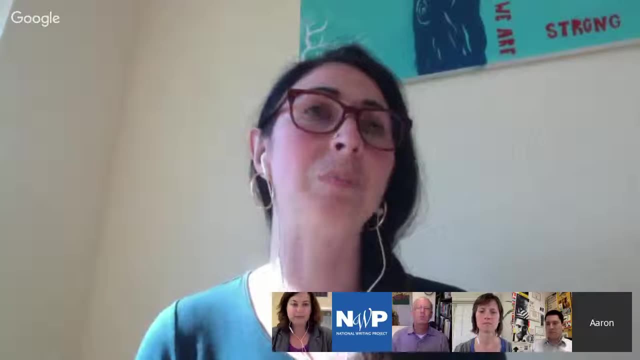 around social justice issues And so, as students are exploring these and writing about these, we're thinking about: okay, how do we write to an audience and then get that work out there? And it's one of the things I struggle with, because I think it is a really valuable tool to put. 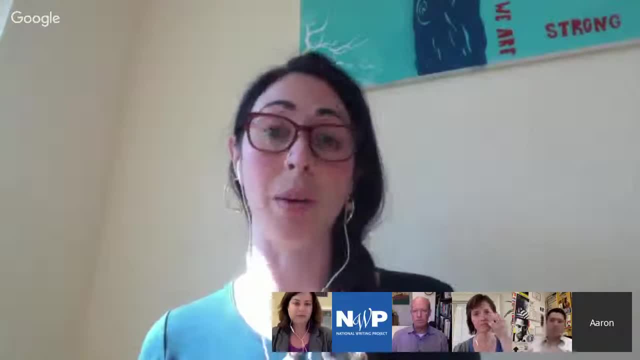 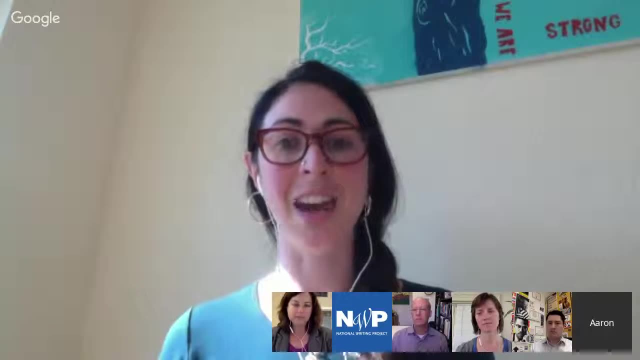 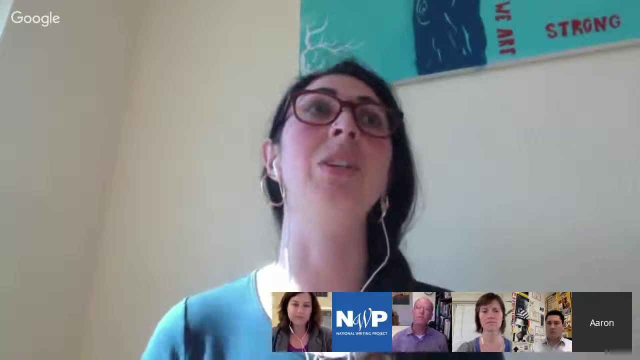 for students to learn how they put their work out publicly and to think about audience engagement, But it's not always authentic in the sense that students' work will be read broadly. Most recently, we decided instead of I had them, instead of putting their work out digitally publicly. 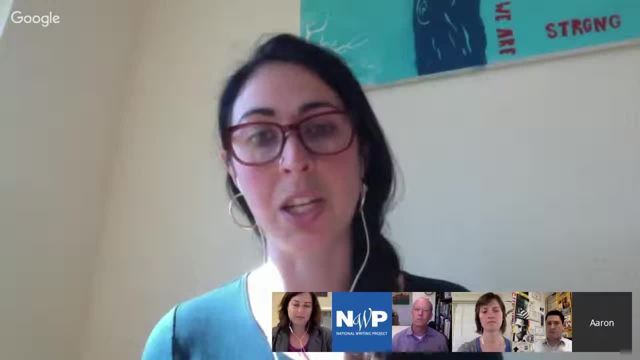 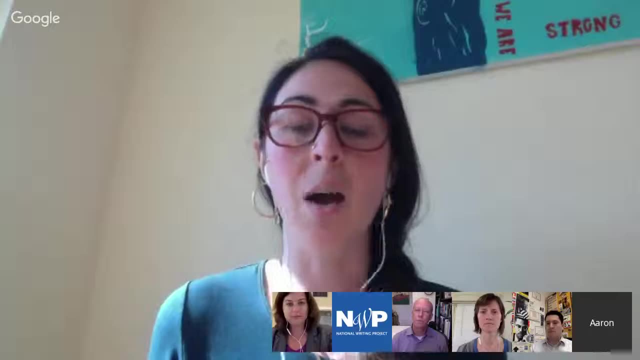 instead to be writing advocacy letters to their local city council member around the issue that we were engaging in, And it took on a level of authenticity that was somewhat deeper than kind of randomly putting their work up digitally on the Internet, And so I don't know if I have the answer to that question. 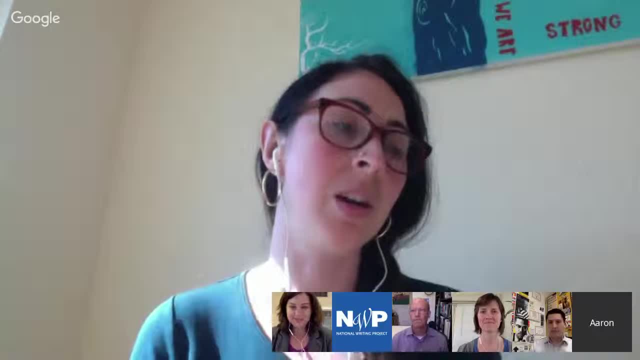 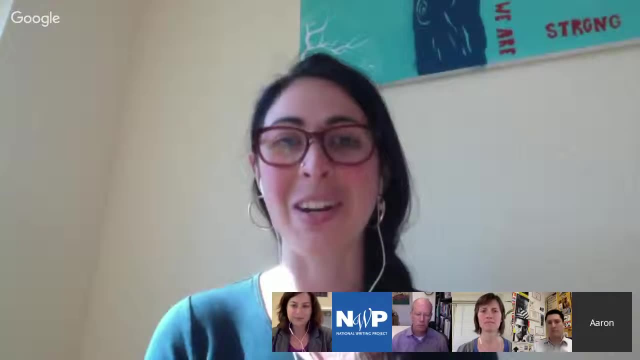 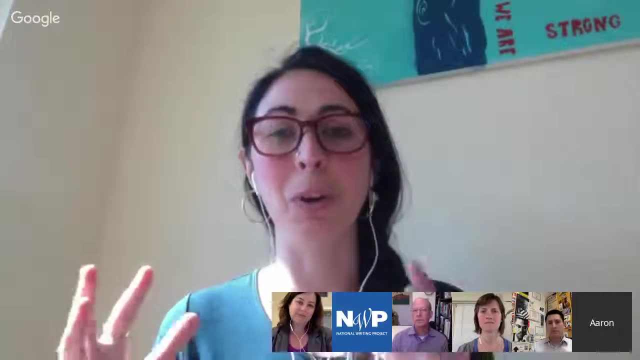 I think one of the things we also have experimented with, not just in my class but in all the history classes, is trying to engage more with social media. And then that's also this funny piece, because it both can be meaningful for students. but then there's this engagement with a very personal area of students' lives. 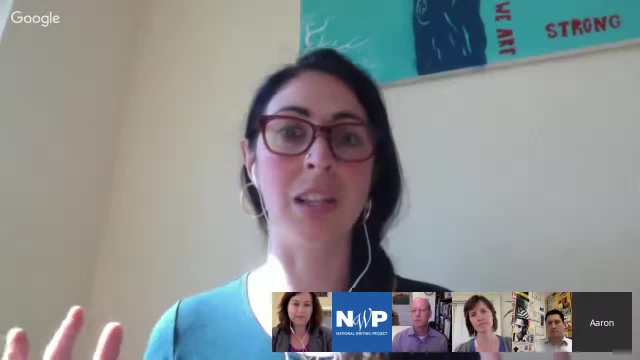 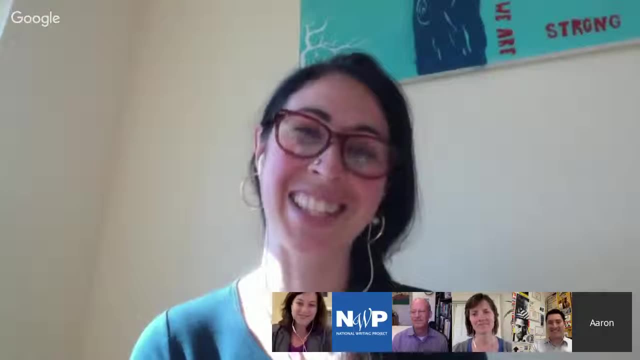 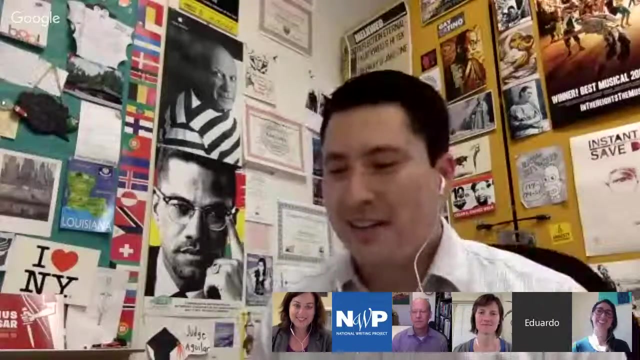 and what is and isn't appropriate to regulate about how students present themselves in that space. Yeah, so lots of questions. Curious what Eddie thinks. Thank you, Perry. I also agree. I think it's extremely challenging as far as having those authentic conversations. 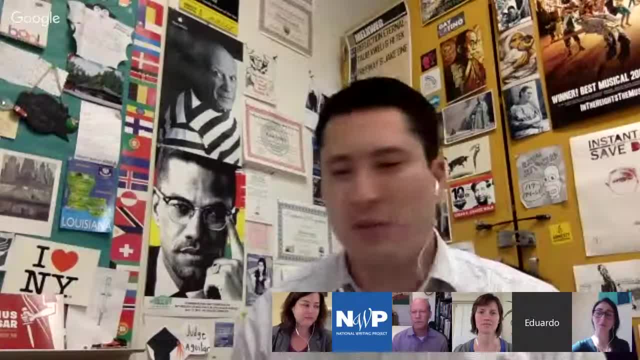 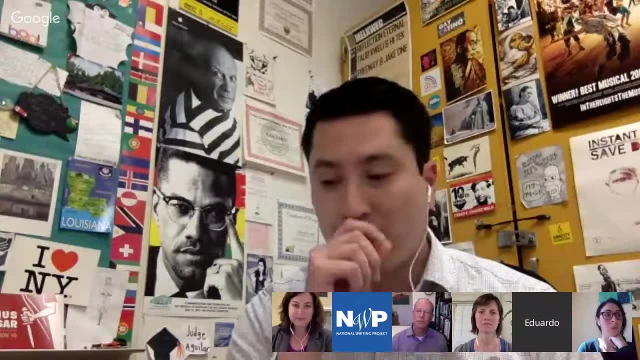 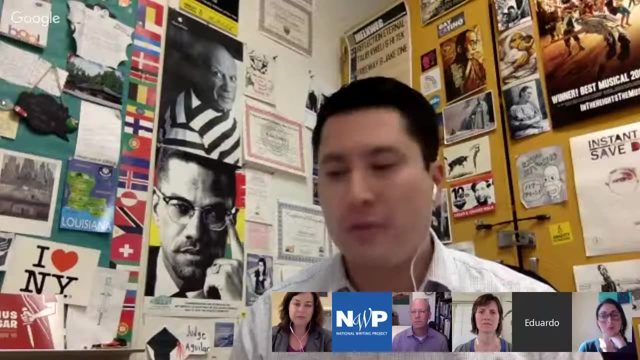 But I guess I'll try to speak more towards like what teachers can possibly do right and use as far as digital tools And, I agree, I think, social media, the use of YouTube. at least in Los Angeles Unified School District we are now being allowed to use YouTube in the classroom. 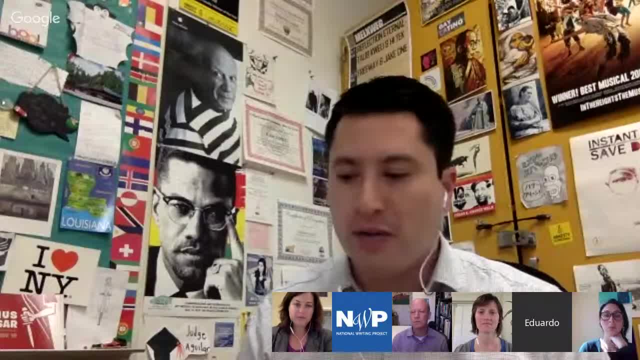 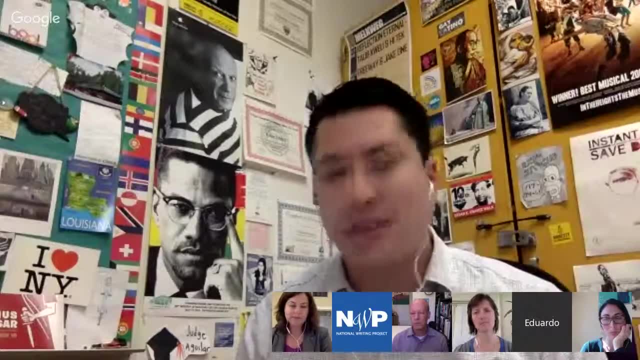 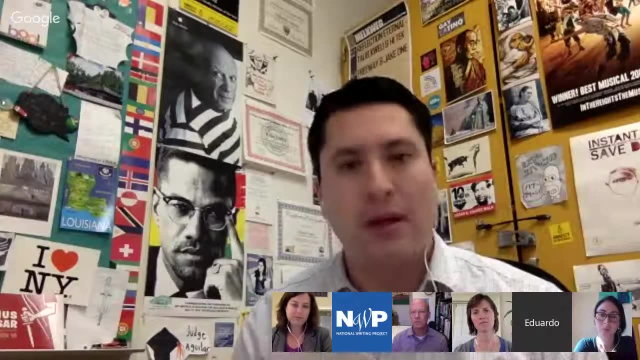 And for my youth, they all have iPads, And so they can actually access the Internet with their iPads, And so that's allowed them and myself to kind of rethink the way I teach and to be able to incorporate technology in the classroom. 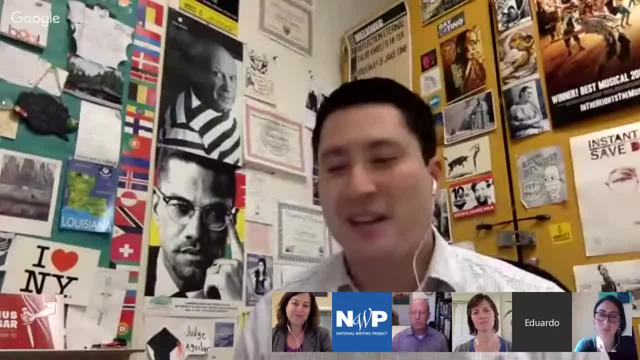 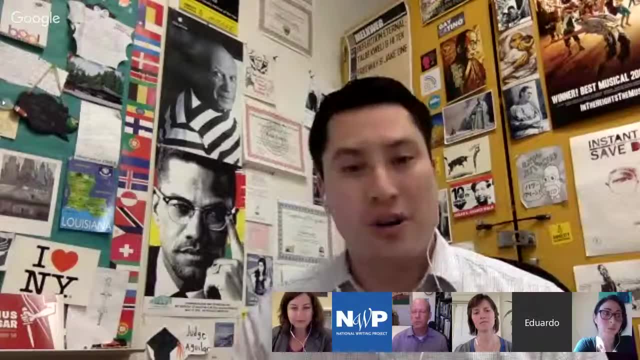 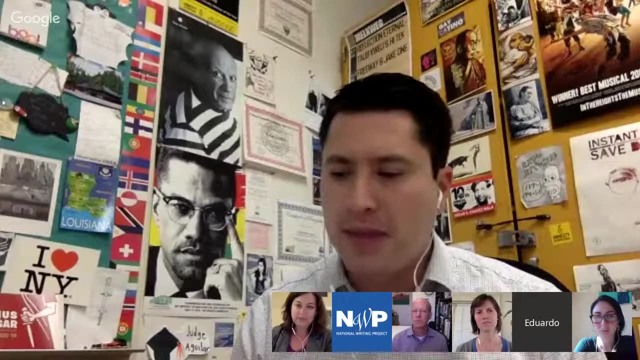 So I feel I'm learning along with my students as far as seeing what's out there, as well as professional development for educators, reaching out to folks like yourself that might have already started on this and having, you know, youth blog, But I guess what I've done is making sure that when we're using technology, 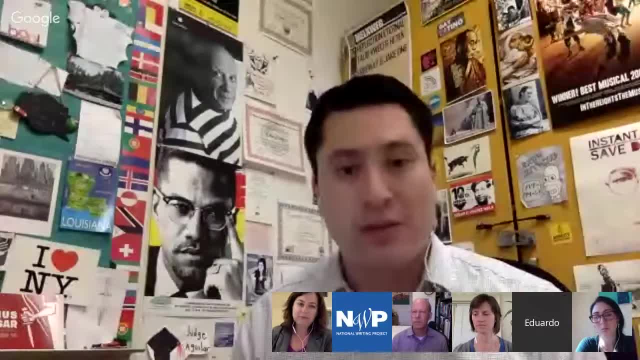 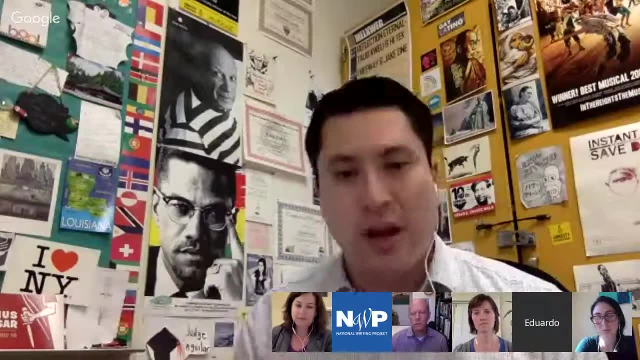 you know how can we use it also in a scholarly way, right? So even when it's filtering even Google searches as a search engine, but you know, going to Google scholars and searching right educational articles that might be linked to the particular topic. 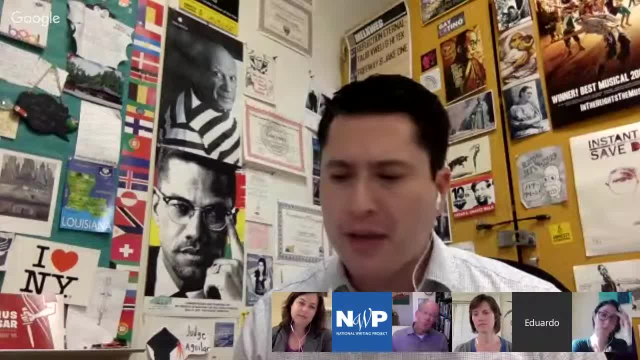 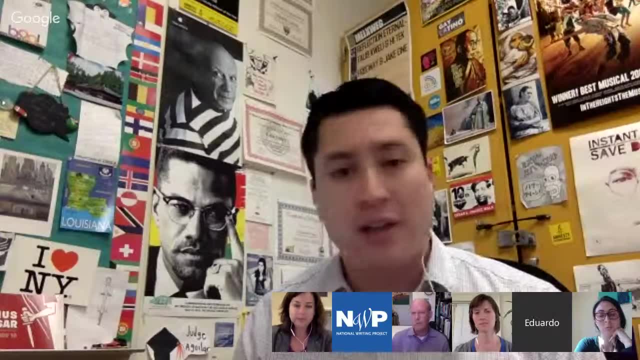 that we're discussing in class. I think of you know documentary footage, you know when we're thinking of you know how do we make this authentic. you know for the students and the audience, And even though it was a different decade or whatever we might be looking at, 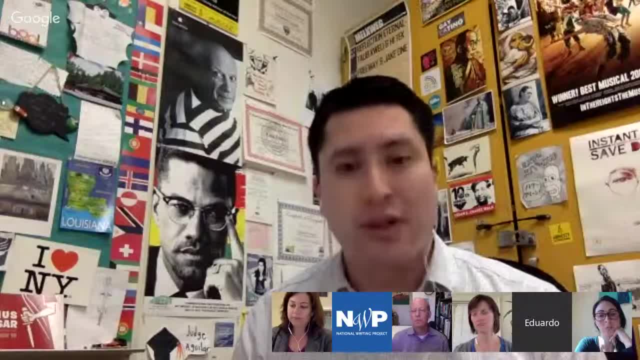 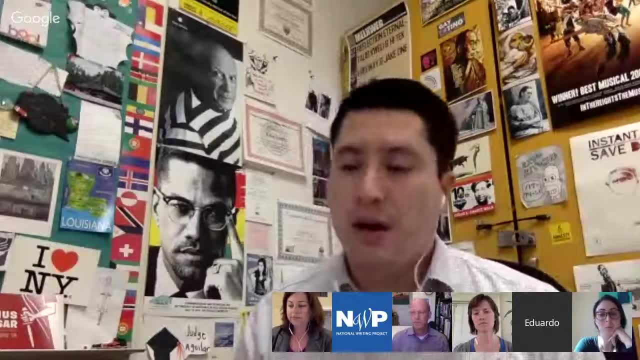 whether it's the civil rights era. I think there's a lot of great footage out there that now I'm able to bring into the classroom where students could hear what youth were feeling at that time and that feeling of empowerment after hearing, specifically with the civil rights era, how so many youth were involved. 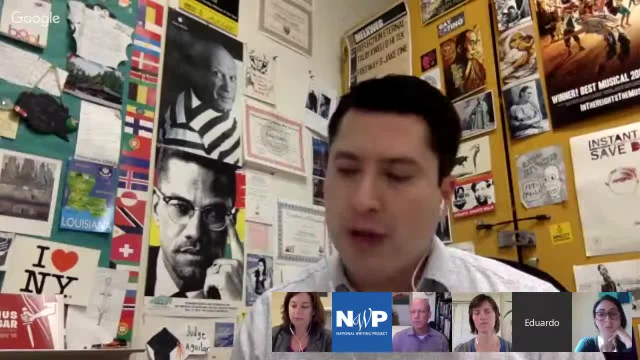 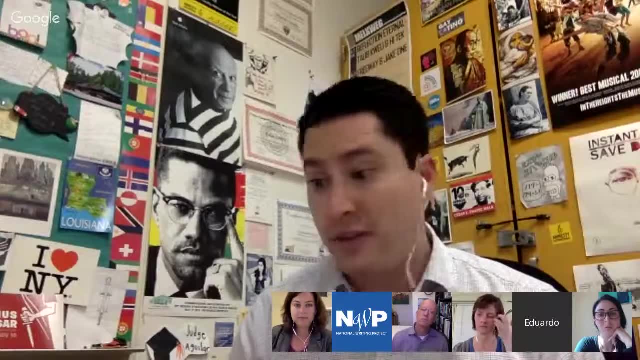 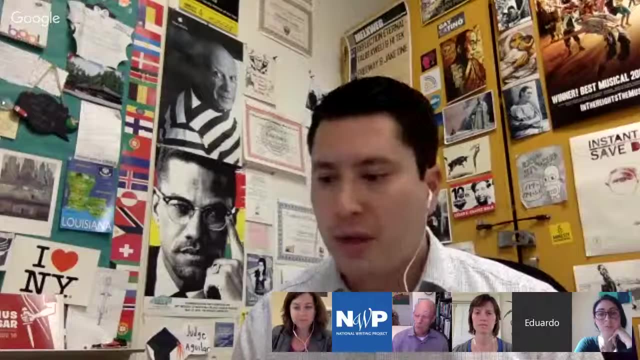 in the movement and in organizing. So I think when I make the link between you know what's happening today, with a lot of the social ills that have continued to plague us and have plagued people of color in the past, it's a great connection that I've been able to bring in into the classroom. 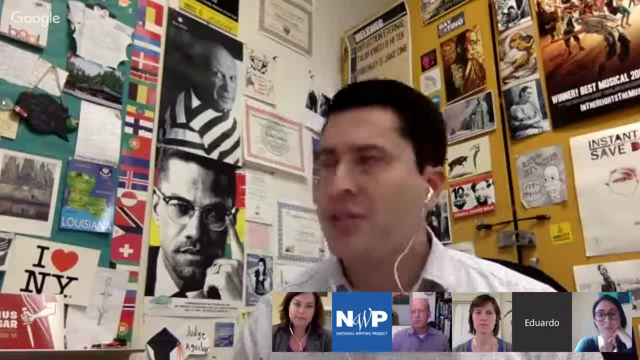 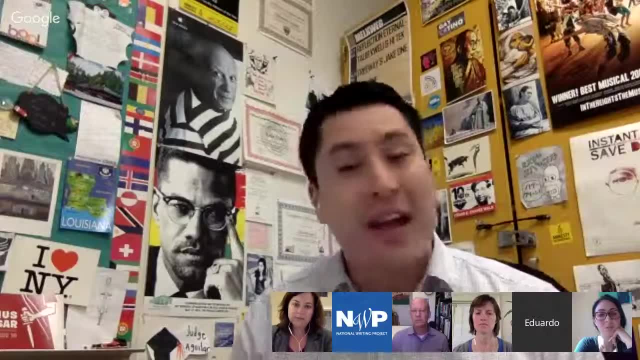 And then you know, even opportunities, like you were saying. you know, I was just thinking of a lesson a little while ago that I did with one, actually with all my US history classes, because I feel with my ethnic studies classes. 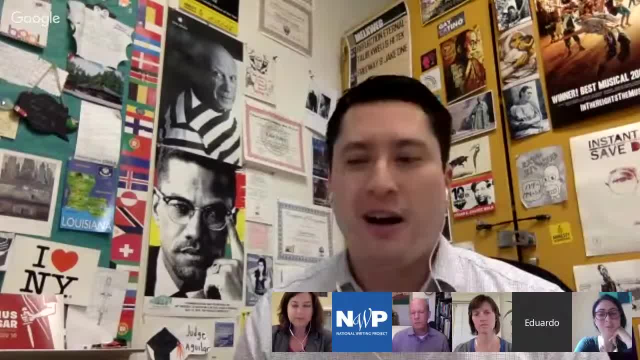 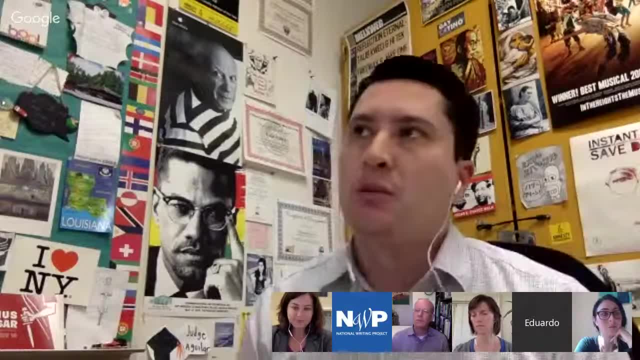 it lends itself more to these opportunities, right, But I guess we're going to be moving on to those type of questions in the next few minutes. but even with my regular US history class I know when we had everything kind of coming together with the, you know. 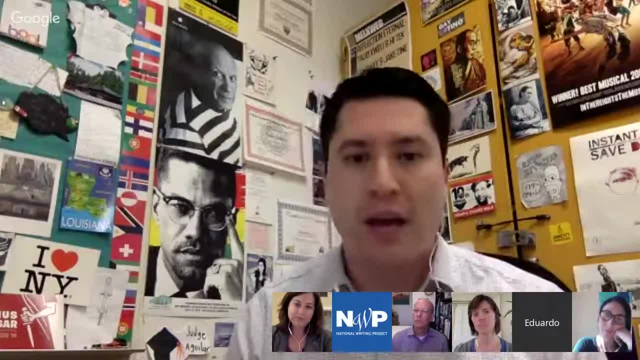 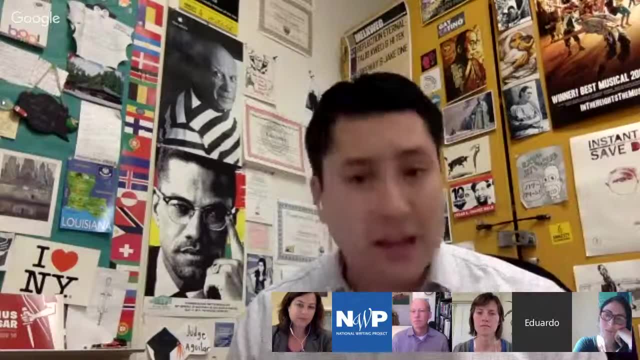 the umbrella uprising in Hong Kong, when we had Ayotzinapa in Mexico, when we had, you know, and still have all of these issues still going on, but with Black Lives Matter being labeled as Black Lives Matter, we were able to pull in a lot of those events in real time. 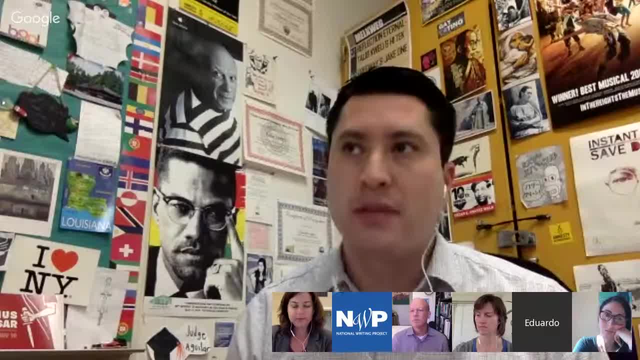 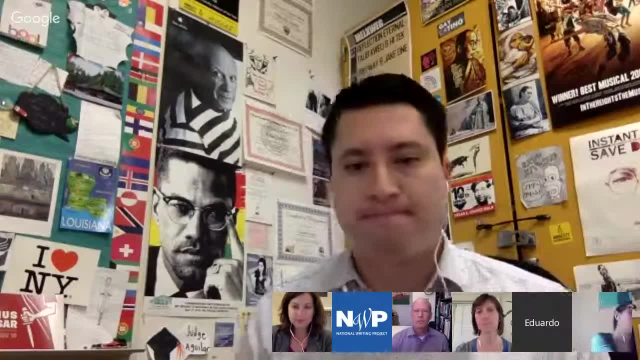 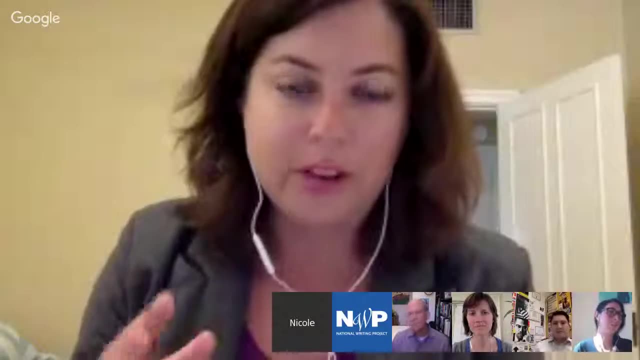 right and we were able to do some really cool activities in the classroom with using their iPads and my access to YouTube. Awesome, And John, I wanted to see if you wanted to jump in. I know you do work with community organizations as well as with teachers. 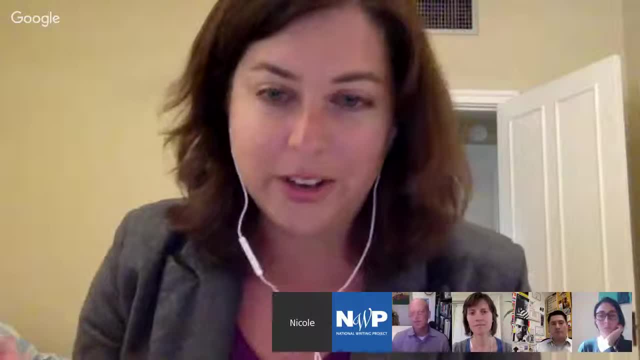 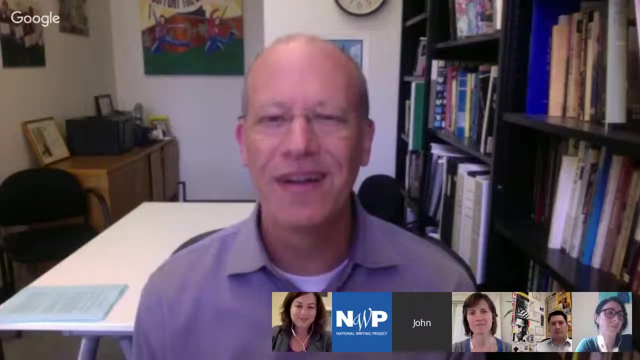 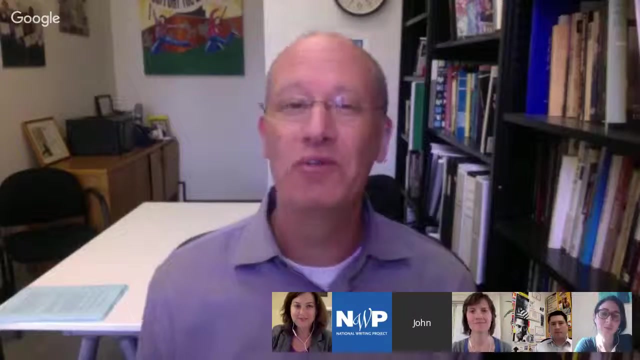 and young people and what you've seen about digital media and authentic audience and how to navigate those challenges. I'm just thinking historically because, Nicole you mentioned, we started doing our youth participatory action research back in the late 90s and when we began we didn't use much digital media. 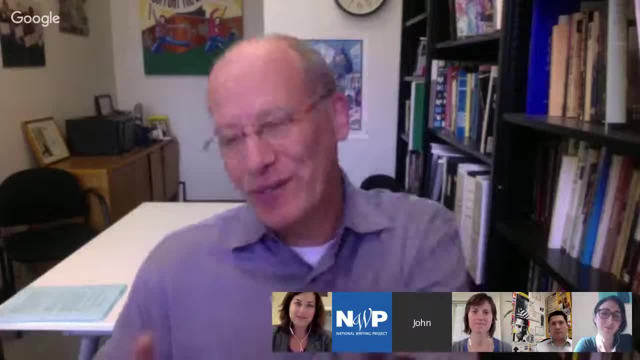 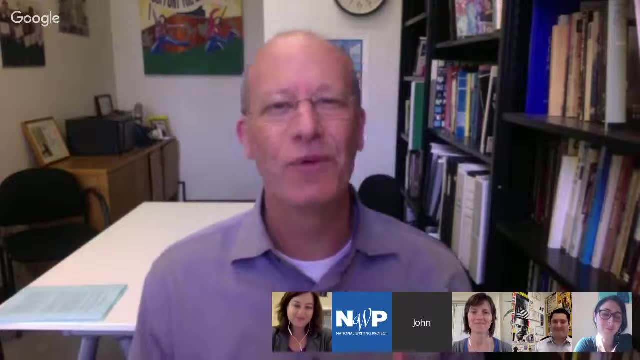 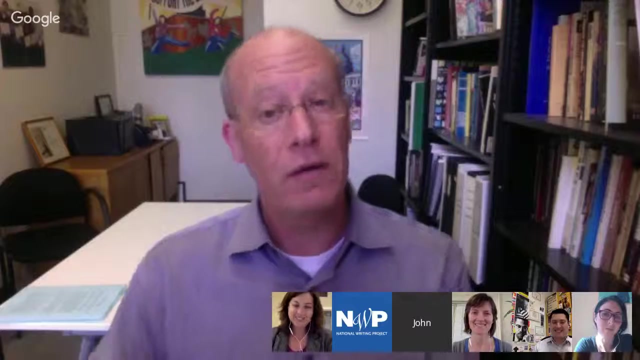 It was young adults or adults in classrooms with young people with notepads, reading Freire, reading Jean Anion, reading other critical sociology very closely with highlighters. That was our technology. And then going out and interviewing other young people, doing surveys with other young people. 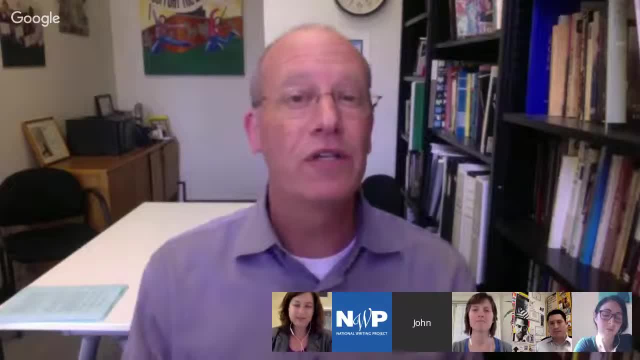 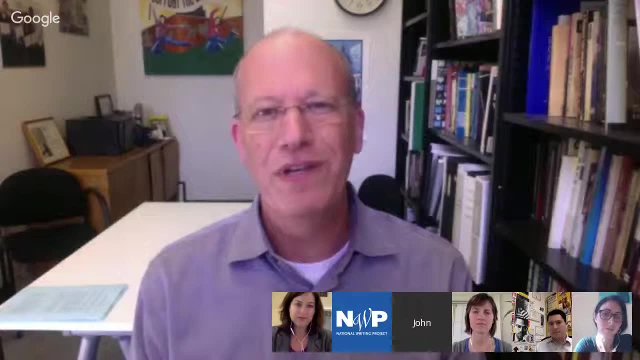 Over time we began to incorporate various different forms of digital media which I think were both engaging for young people, were vehicles for young people to feel a new sense of technical power, but then also became a way to insert the voices and ideas of young people. 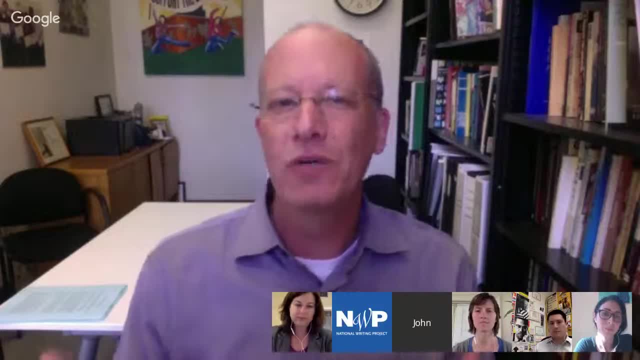 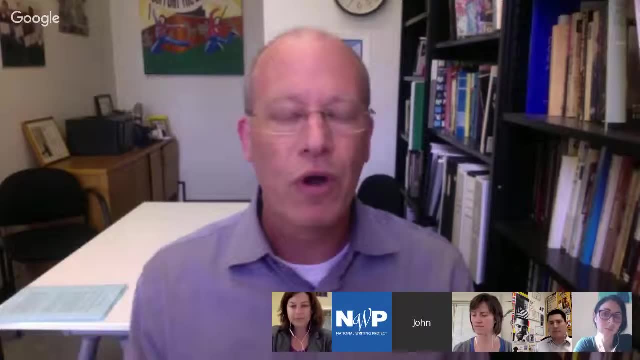 into the broader public sphere, And we did that as young people would present their work, sometimes through GIS maps, sometimes through videos. I recall in particular, in 2002, there was a statewide class action lawsuit in California, Williams versus California- that was challenging the substandard conditions that prevailed. 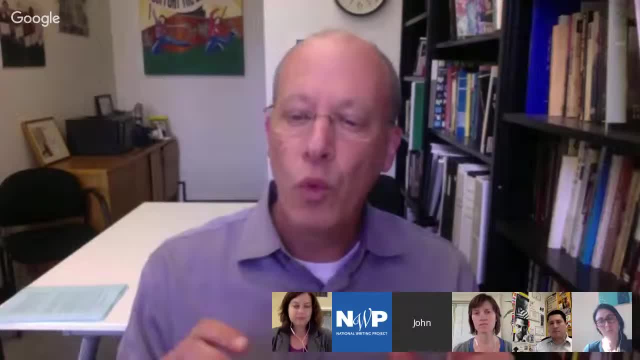 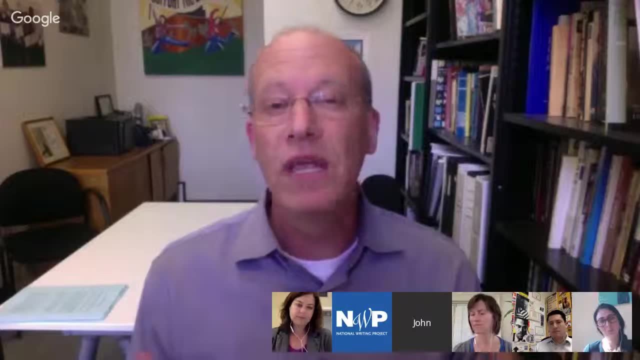 in a lot of schools around the state And one of the groups of students took this amazing video at a couple different schools of these conditions And when they presented this to civil rights attorneys, the civil rights attorneys said: you know, we have all these depositions. 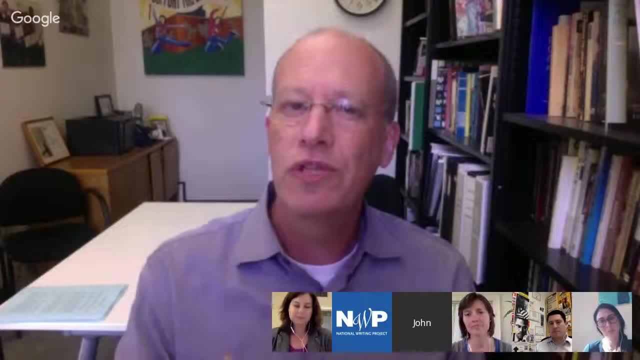 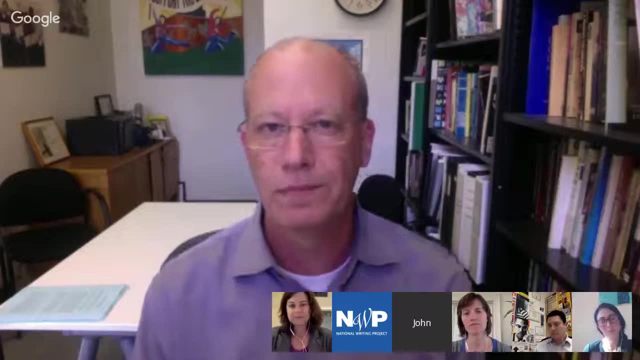 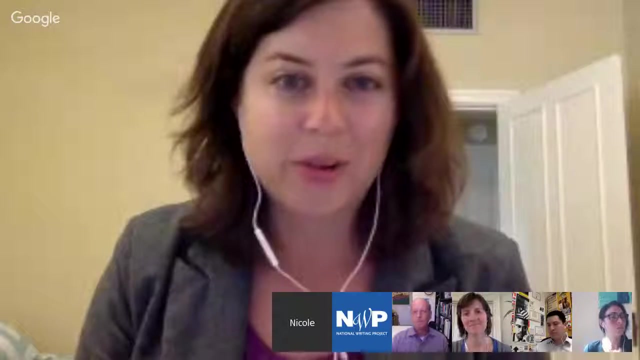 we have all this evidence, but this is some of the most compelling evidence that we have to make the case for the unconstitutionality of prevailing conditions. That's awesome, And I think the power of Twitter today that has that democratizing force so that young people can have their voices out there is also great. 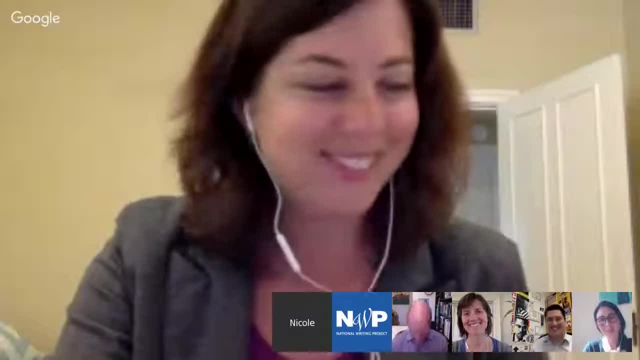 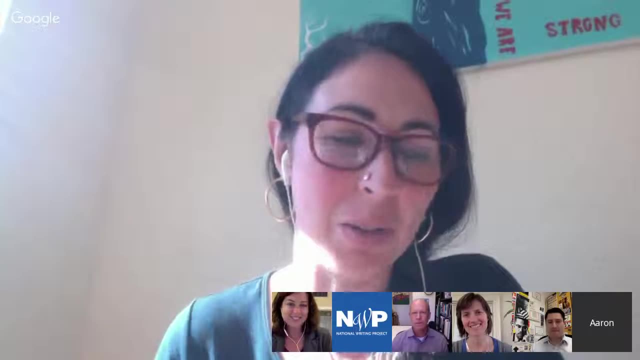 I've been trying to get John to go on Twitter, but he's not doing it yet. Okay, I think if I could jump in. I just feel like I need to speak to some of the work that my students did do And I think thinking about this question. 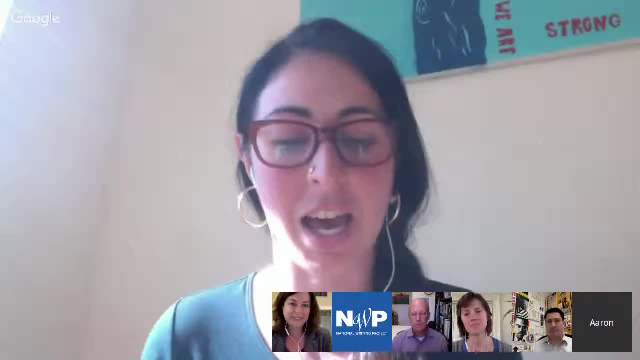 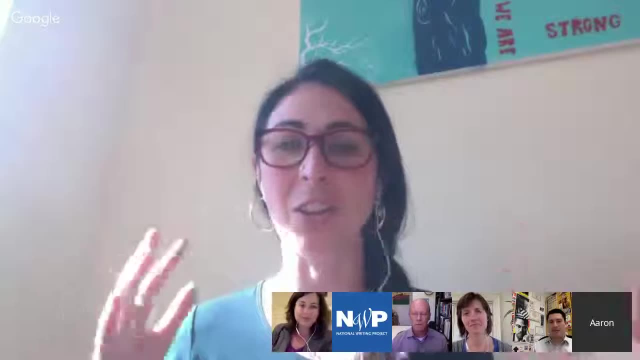 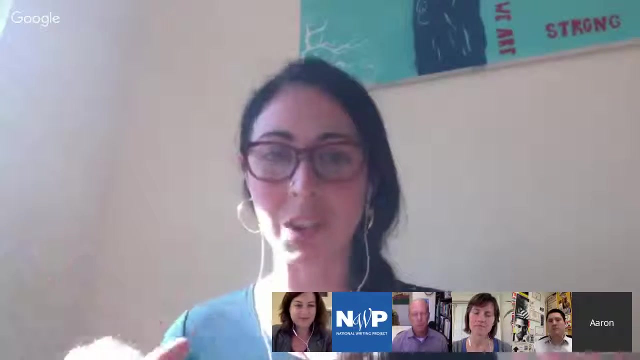 I was thinking more around kind of blocks, block tools such as that that I think are actually pretty useful. as I think more about it, the way that students are able to comment and engage with each other in like these broad conversations, where in the classroom we can create space for deep levels of student conversation. 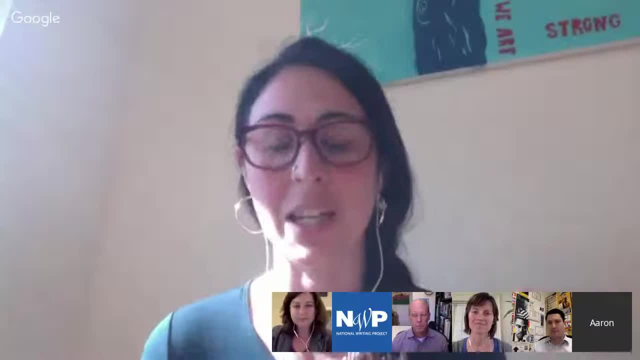 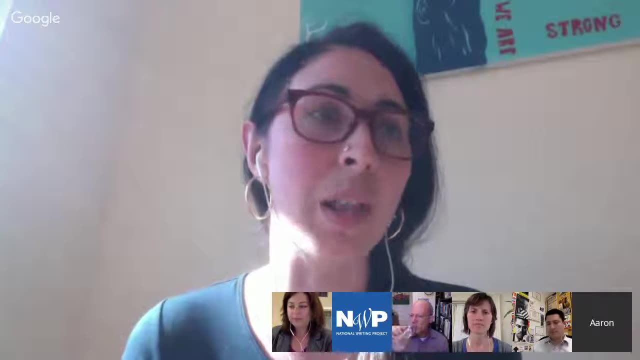 but fundamentally they're not all speaking to each other at once and some of that stuff can happen online And I think that's kind of the richness of it. But last year, around the Black Lives Matter and anti-police brutality organizing, a group of my ninth graders really took on that issue. 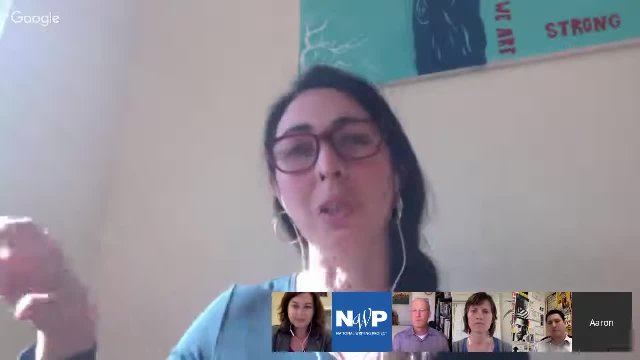 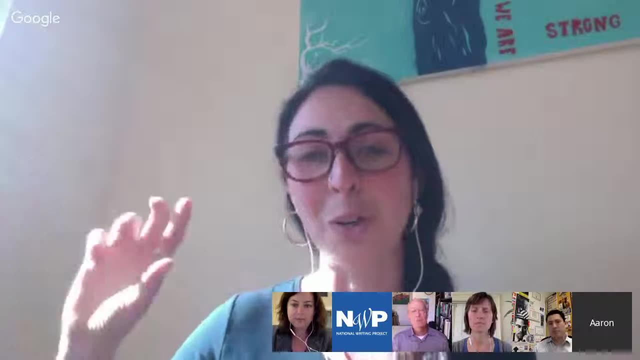 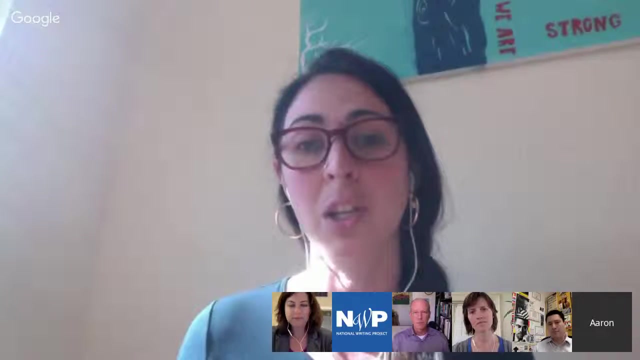 And we started using social media as a way, and they created a hashtag around this movement of high school students. Free Oakland was hashtag. Free Oakland was what they put out- to organize marches and actions by high school students around those issues, And I think that is how they were able to connect with each other. 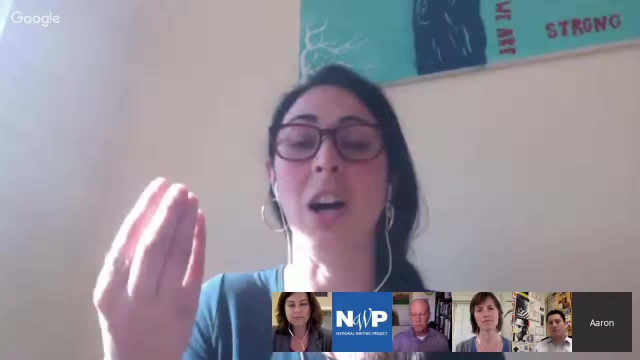 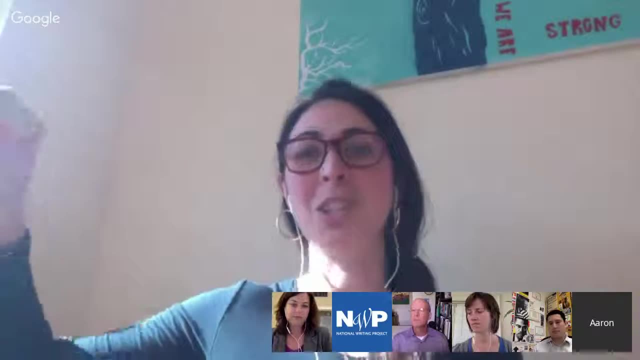 And so what we were doing in the classroom around studying the issues and talking about organizing strategy, they were then translating on their own time, And so I think a lot of the time, like the digital tools aren't necessarily even what we teach, but it's how they're able to translate what they're learning in the classroom. 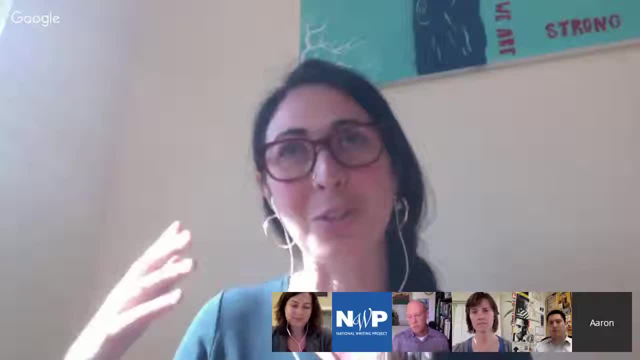 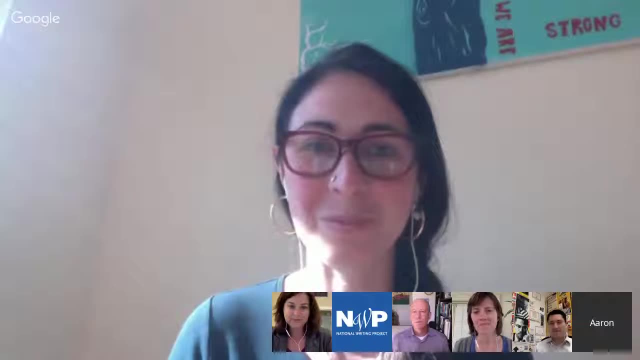 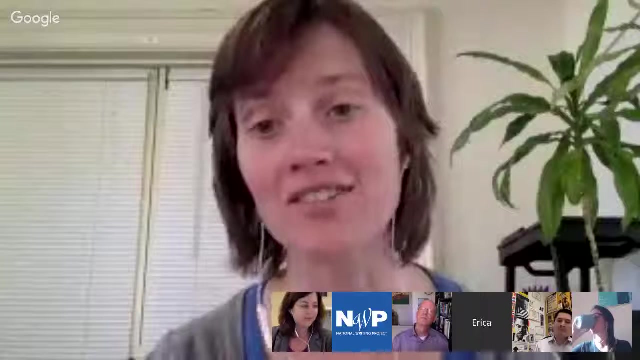 and make it authentic for themselves. So I was just reflecting on that, because I think they did some really powerful work through that. That's great. Well, I think some of you have already touched on a little bit around this organization And I think it's really important to think about. 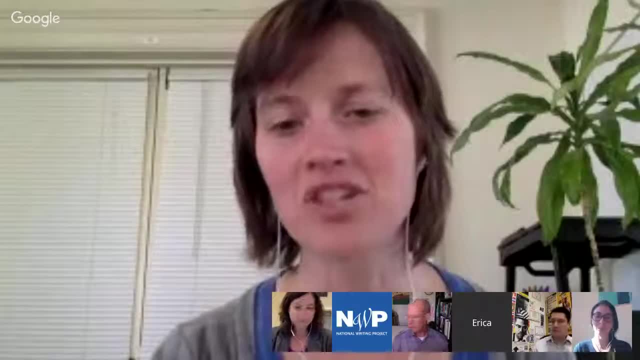 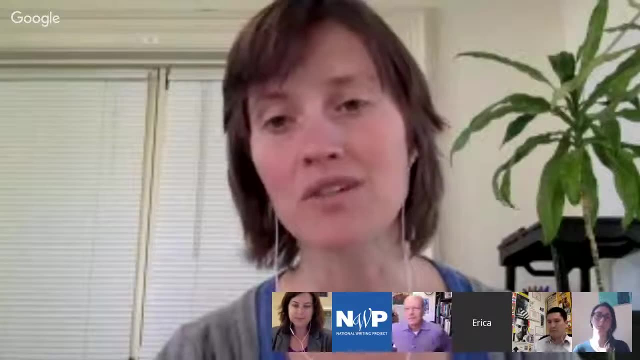 the challenges in the digital age. So of course, as we've all been sharing, there are so many opportunities for young people to get their voices out there, to mobilize other people to investigate or research issues. But of course, we know that with any sort of new genre, 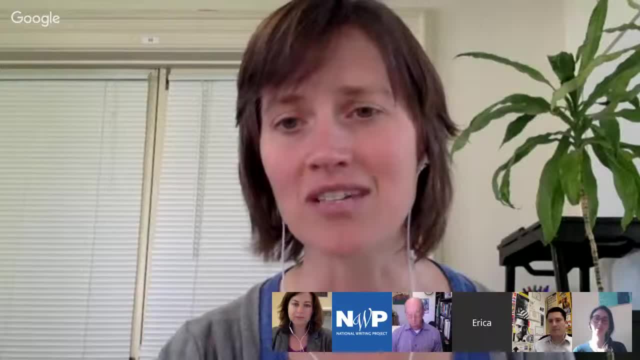 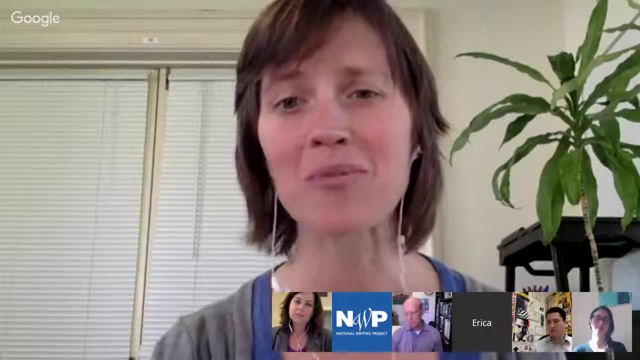 there are also nuances to consider and different things to sort of understand and reflect on. So I know, Perry, you touched a little bit on this idea of like an audience problem. right, I know there's a lot of stuff out there, but do you actually have an authentic audience for it? 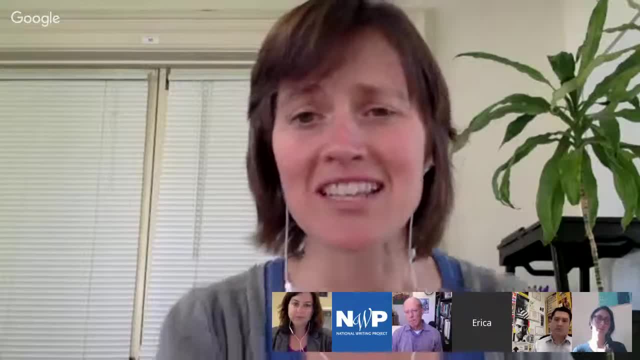 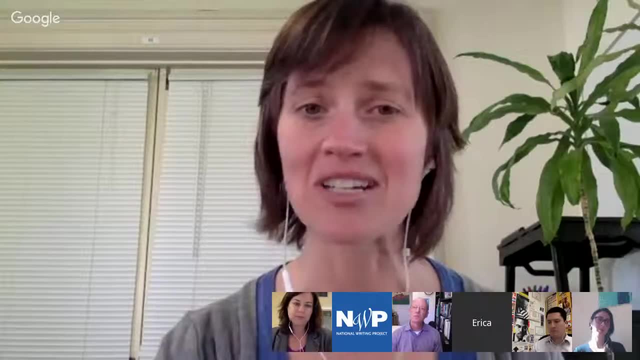 I think, Eddie, in talking about you know research and also John, it's like there's so many sources out there. now If young people go online and do a search, if it's Google or Google Scholar, they're going to get you know a ton of sources. 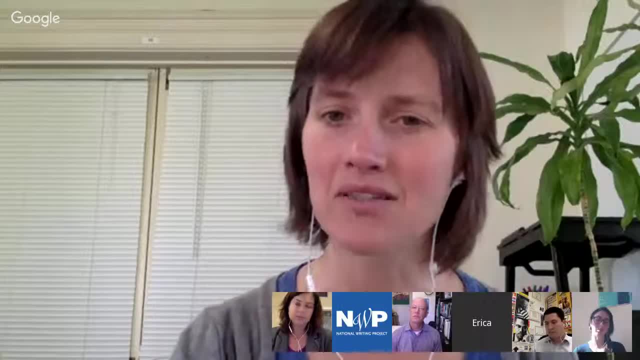 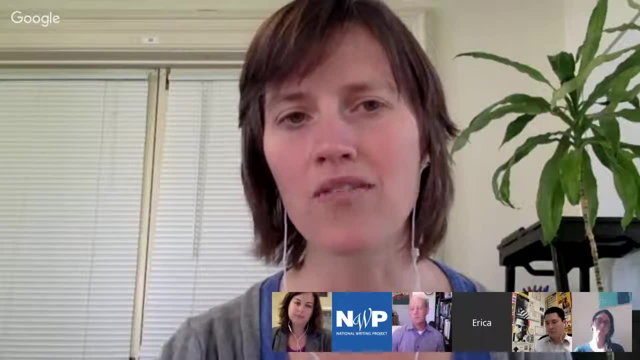 So how do we help young people think about the credibility of those sources that they find? So I'm wondering, I would love to think with you all a little bit about you know, what's the role of educators in helping young people navigate this new landscape? 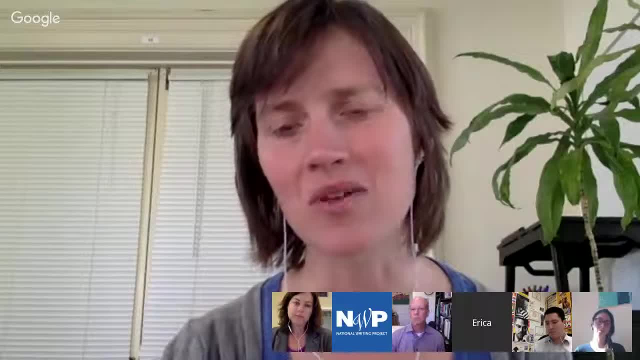 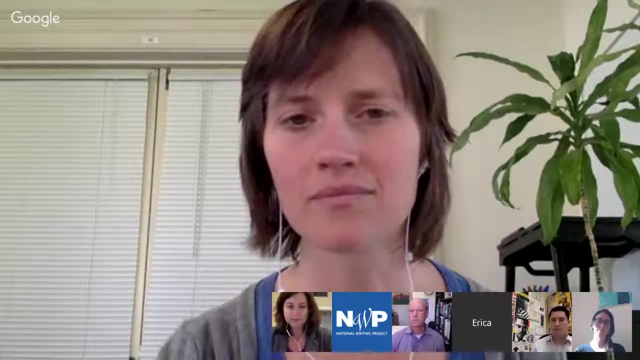 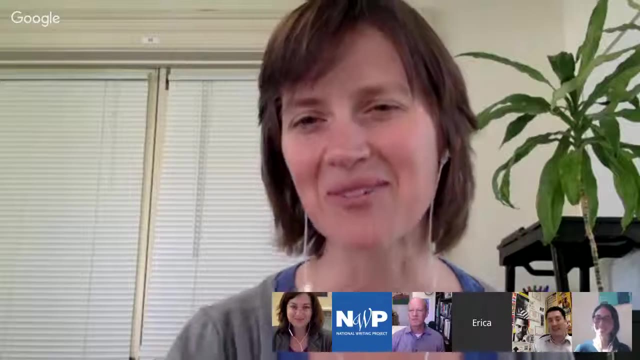 So we've talked a little about the opportunities, but what about these challenges and what are some ways that you all think educators can play a role in that? I hate to put you know, Perry and Eddie on the spot, but I don't know if one of you minds starting us off and 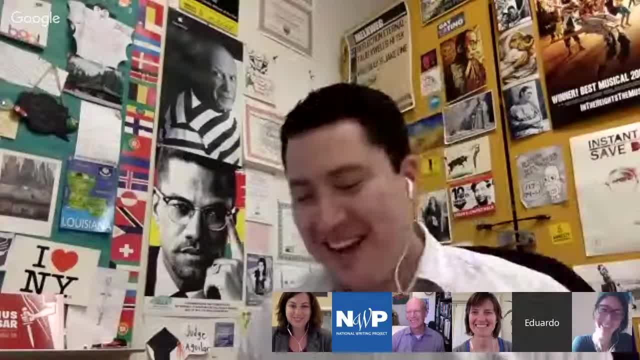 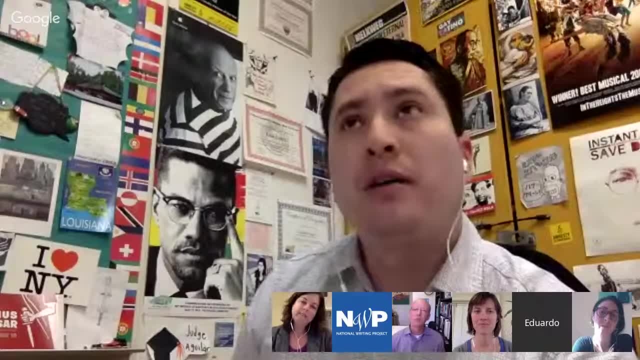 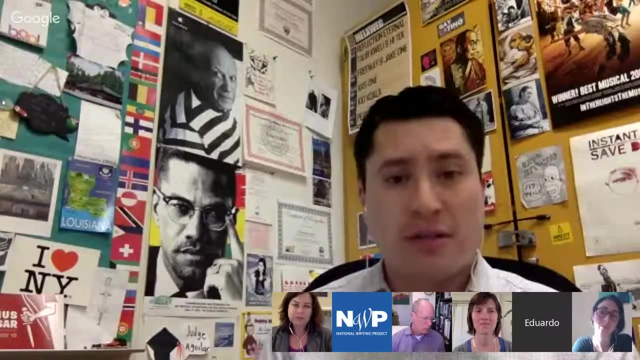 Sure, I'll go first this time. Yeah, when thinking about that, I was just, I was thinking of you know what, When I'm thinking of other teachers here at my school site. right, and the familiarity that we need, even with adults. 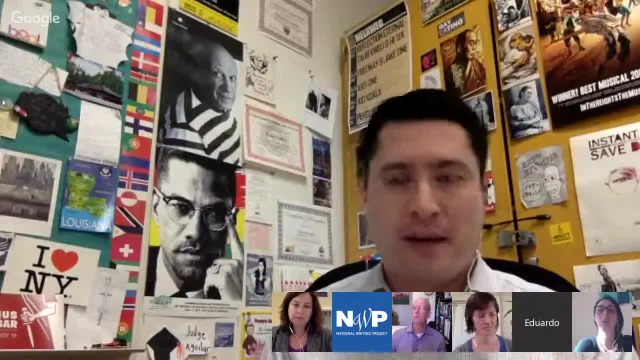 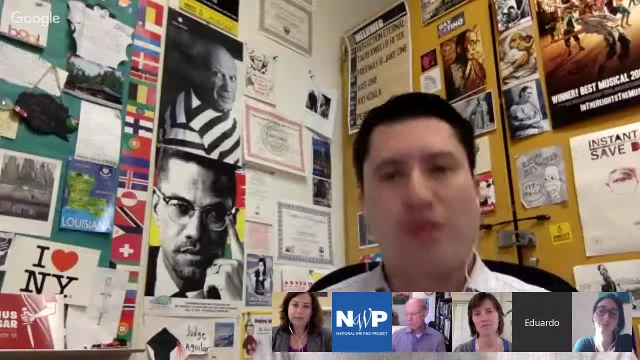 and the use of technology in the classroom. I feel that you know when, Even using, like how John was talking about old, traditional ways of you know, researching or taking notes. right now you have an iPad where you can use notes. 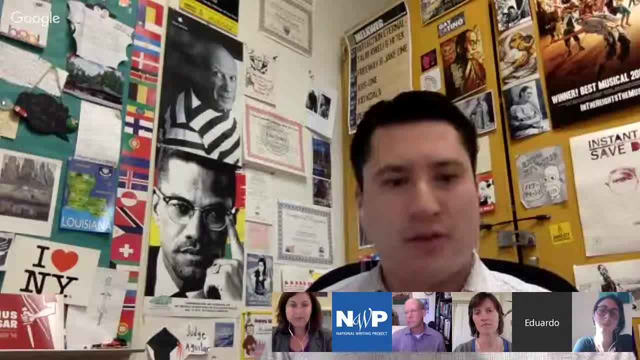 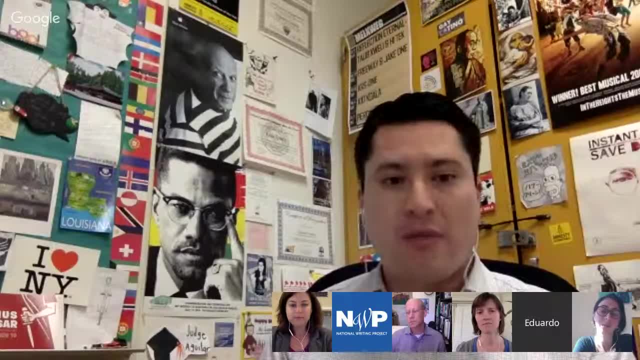 you know you can. You can use notability and other things right to take down notes, But I think some of the fundamentals obviously are always crucial, such as like sourcing right. We very much do that with the sources that we're filtering. 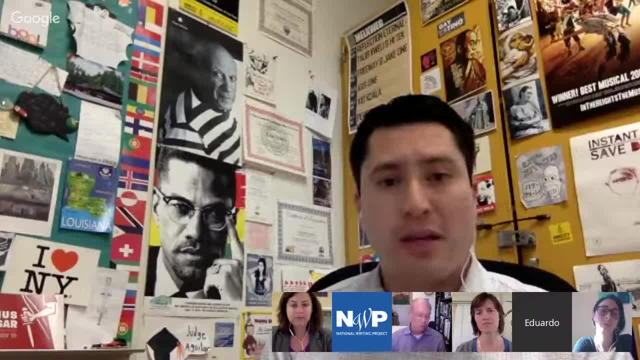 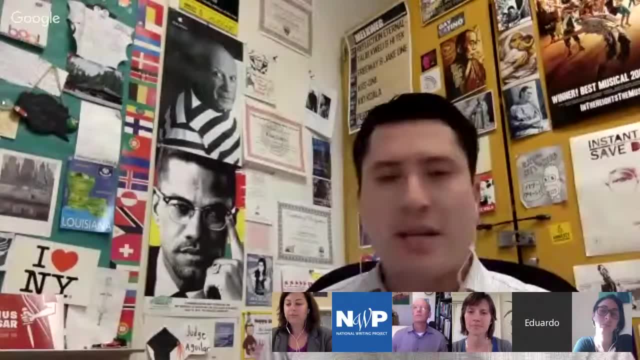 and receiving, because we're just so bombarded with so many things. when you plug in any type of right word on any search engine, you'll get a lot of results. So always asking of you: know who is the author? who is the audience? is the source credible? 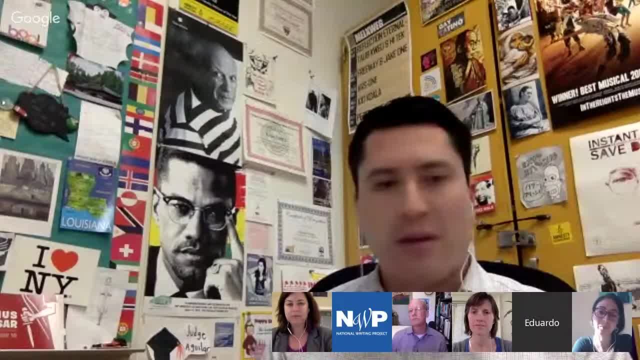 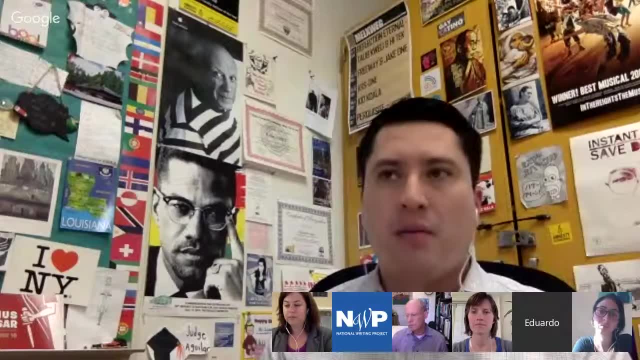 how do we know if it's credible, right? Those kind of fundamental things that we do when we look at biases and when we're looking at, you know, primary documents and secondary sources with text it's the same way. It's, you know, just now looking at it digitally. 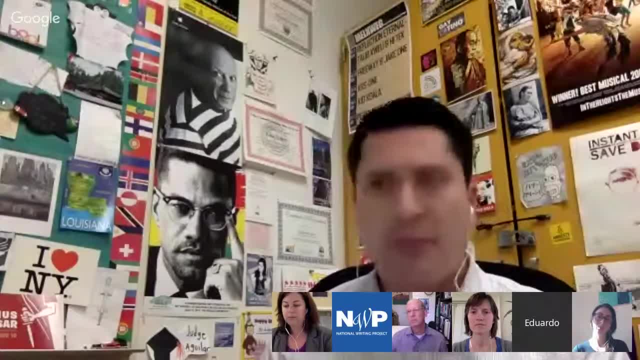 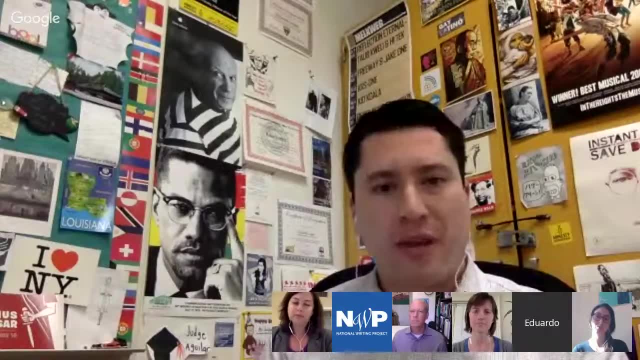 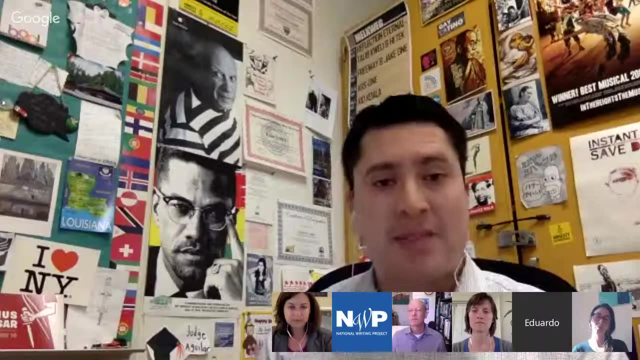 But also even learning myself right with assigning projects on Google Docs, assigning projects on Keynote really pushes me to learn, and the students, And so together, I feel we grow together in these opportunities And these assignments and these projects, But I, for me, I think that the thing that holds back 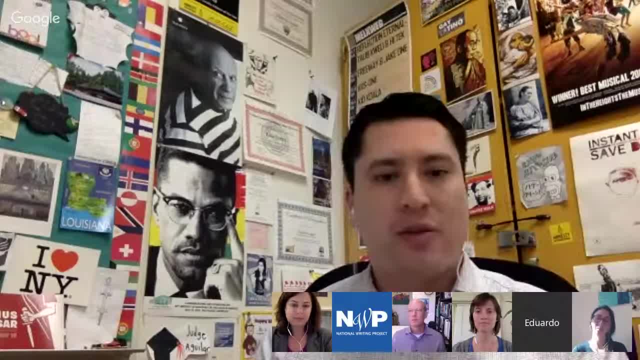 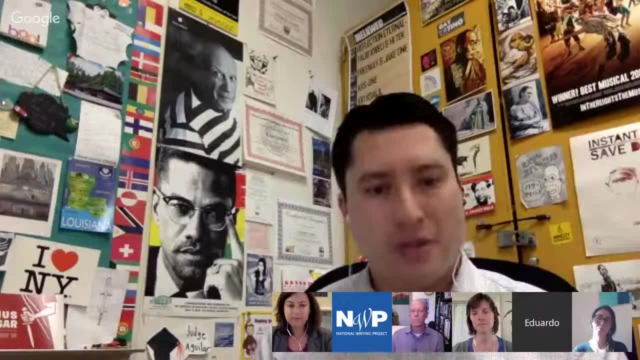 a lot of teachers is just that: not knowing how to navigate through it, not feeling comfortable with it. But I think there's a lot of value in being vulnerable and allowing yourself to be seen that way by your students, because it is a new age. 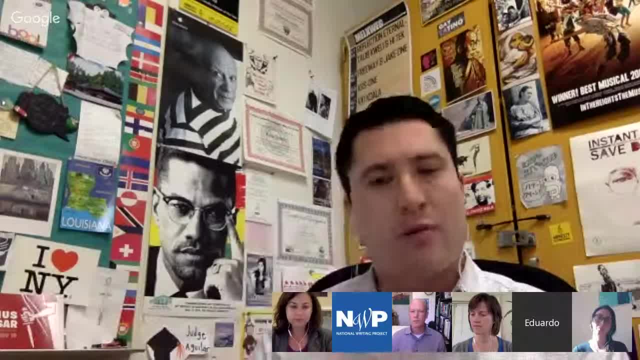 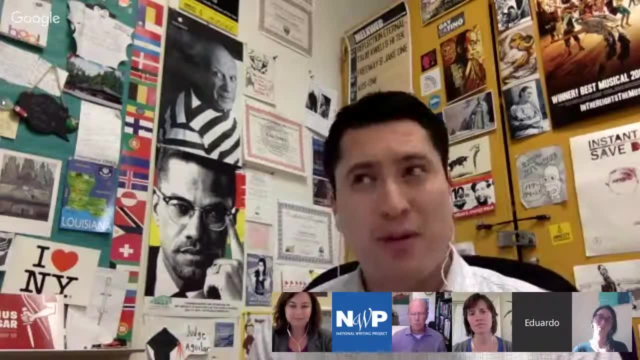 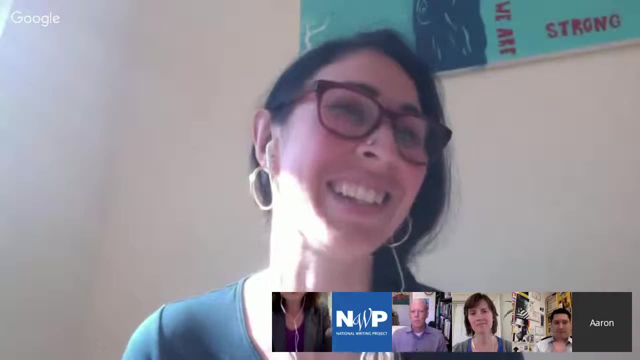 And I think that together, right, we progress and we grow to you know, and that way we navigate through these challenges together, Because the same questions that they come up with are usually the same questions that I have as well. Thanks, That gets some thoughts flowing. 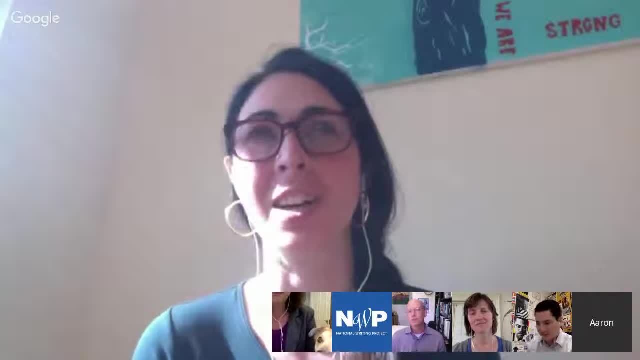 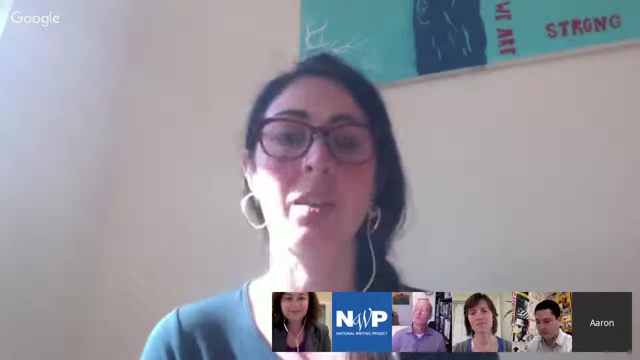 In terms of challenges. I mean, one of the first things I thought about was just how we teach students and talk to students around privacy issues. That has to do with the work that they produce for us, For example, when I ask students to write their about pages. 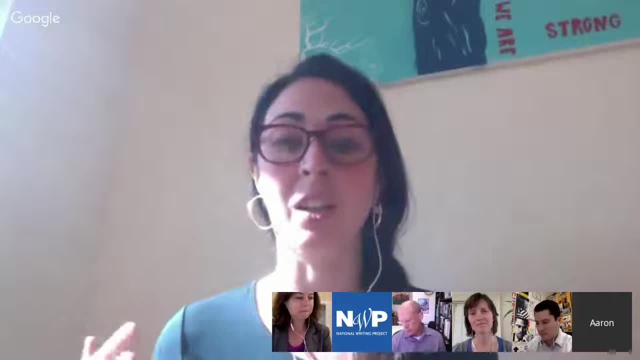 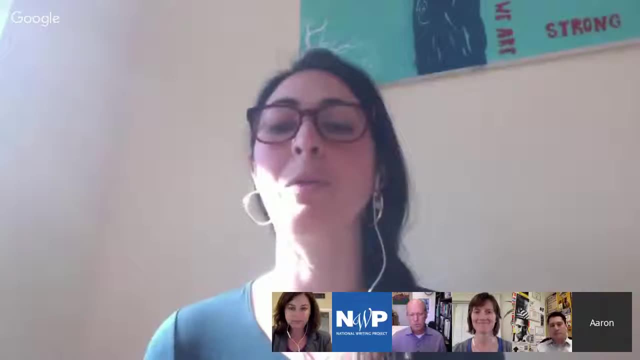 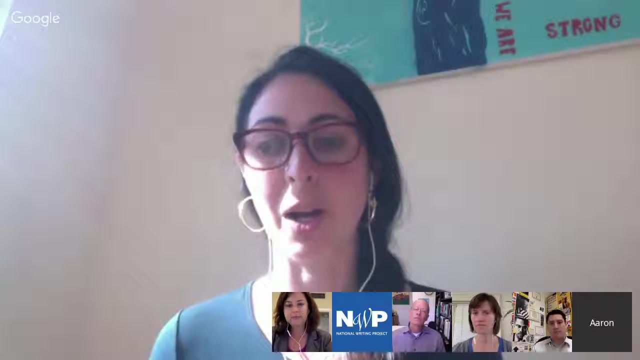 for their blog, the level of comfort that they feel revealing deeply personal stories about their own lives publicly on the internet. Like what is my role as an educator? to support them in a certain level of self-censorship around what we put out publicly. 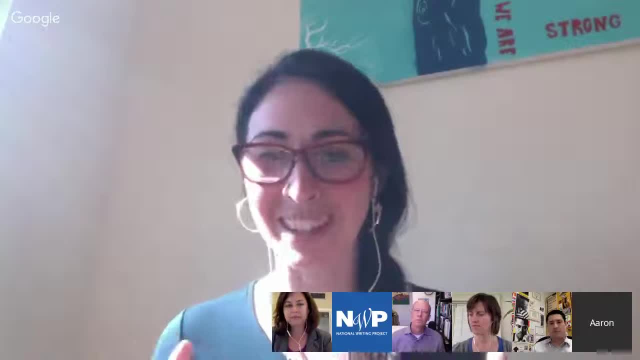 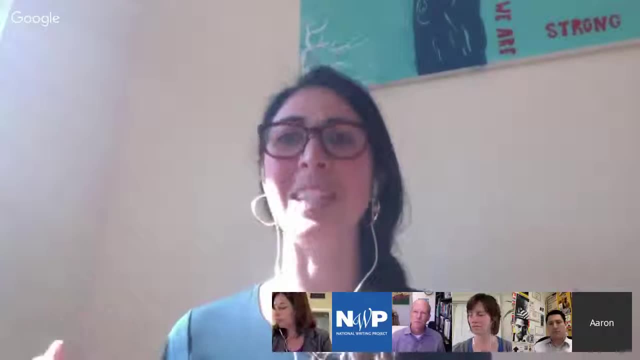 And what are the norms of their generation, as opposed to mine, around what is appropriate and how do they think about their own safety and security in that process? Like those are really deep conversations to be having with 14-year-olds and really critical. But that, I think, is something that comes up and it comes up. 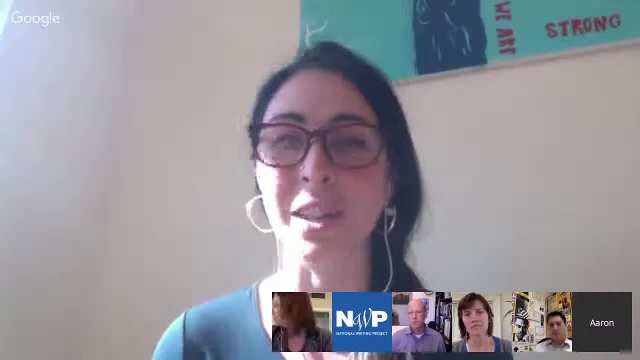 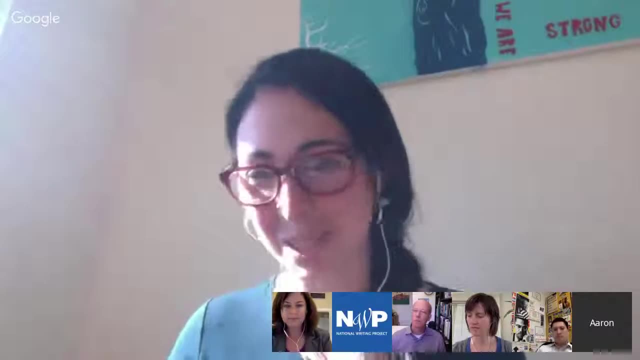 both in the context of the writing they do academically and also how they interface with the school, when all of their personal life is available to administration, right that sees them on Facebook And really needing to be like aware of those things. 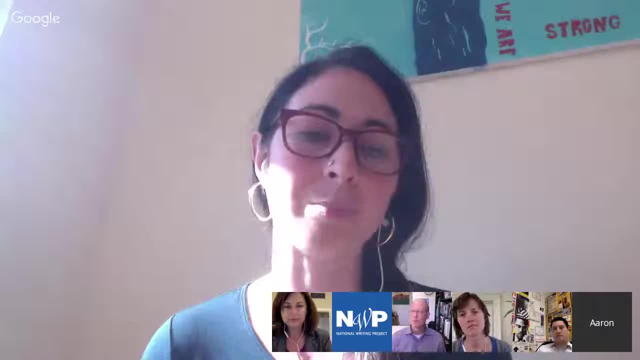 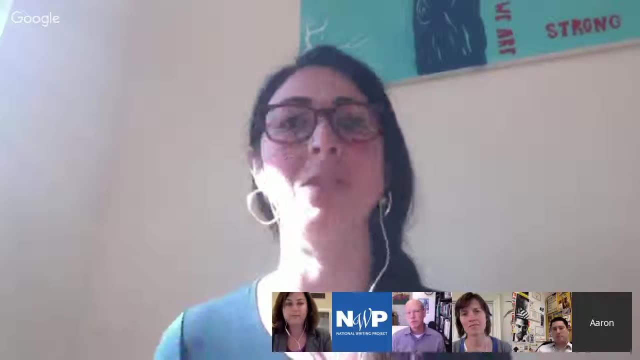 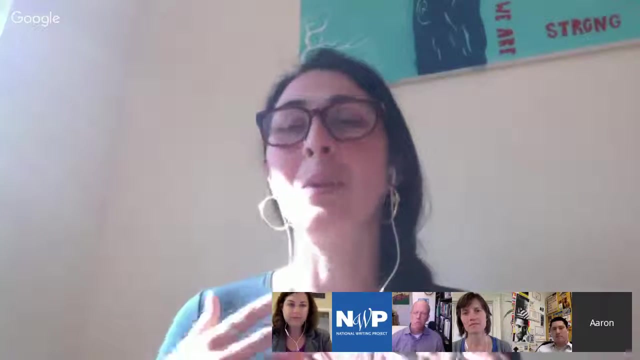 When you were talking about evaluating bias in sources. I mean, I think that there's such a wealth. there's so many sources. If you ask students to research a particular issue or historical moment, or whatever the content might be, there is an enormity of sources that they might look at. 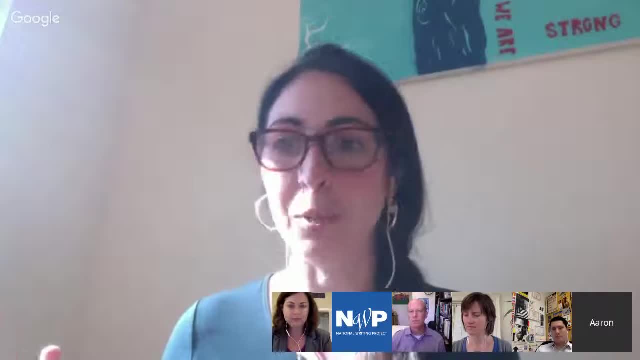 and they're really still developing and probably won't develop until they're 19,, 20,, 21, the lens that they need to really be able to identify the political differences and ideological differences between sources, To be able to say, okay, I'm hearing a certain perspective. 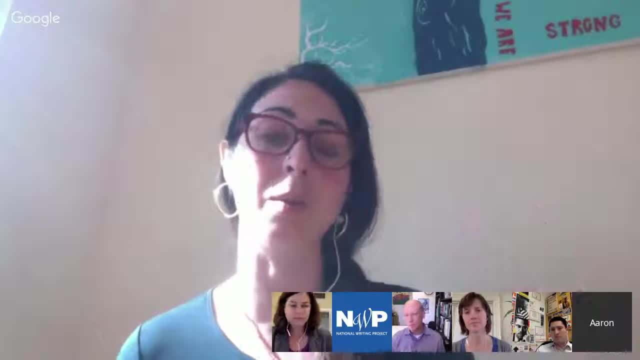 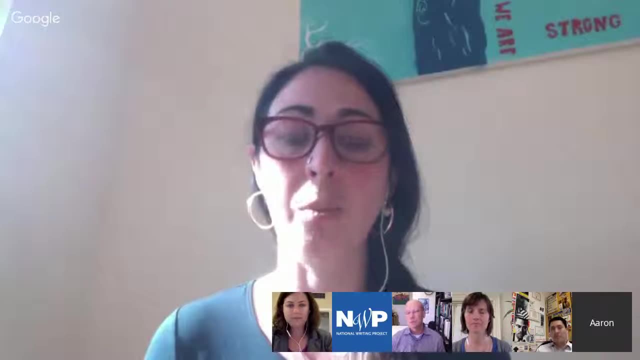 and I can guess or make assumptions about where this is coming from and what it's being informed by. that's really hard for young people to do, especially young people who may not have been exposed to like the large variety of different political perspectives. 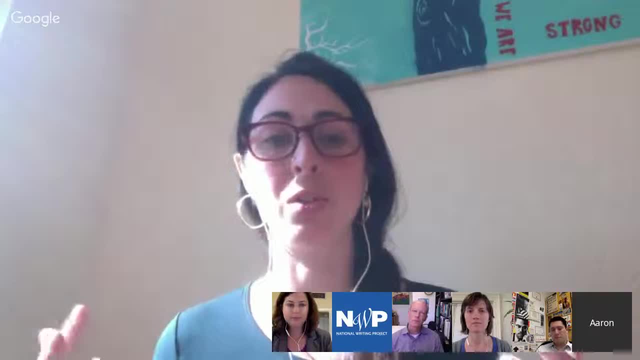 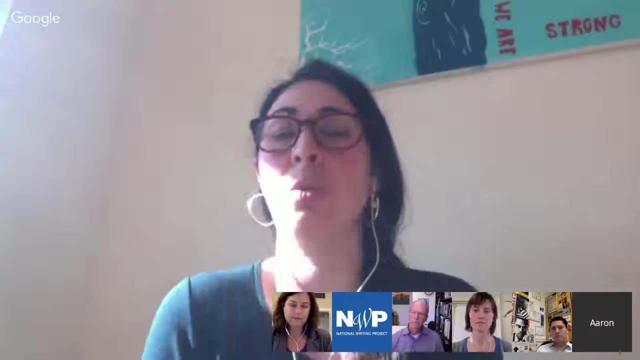 I think a lot of my students haven't been exposed to some of the more conservative perspectives in their own personal lives that they might see in the media and their day-to-day lives and so don't really know how to translate it or make sense of it. 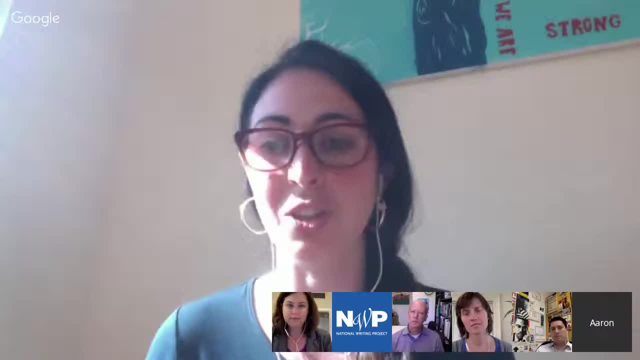 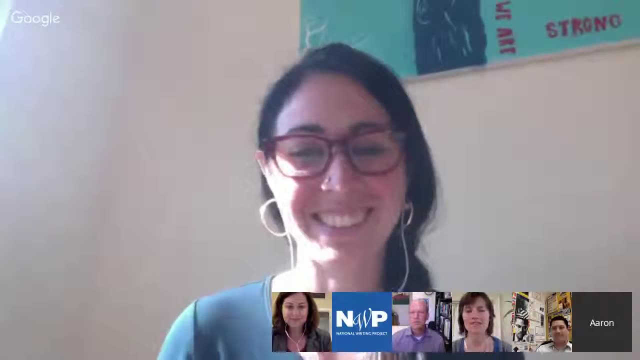 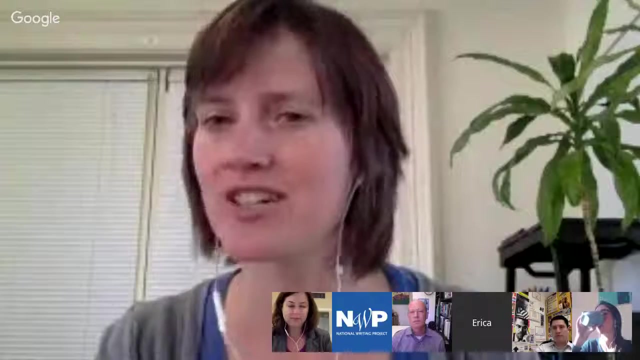 And so I think that can be really challenging for them to engage with. Yeah, so those are some places to start. That's great. Thank you both. I feel like you're both touching on really key considerations for educators and I'm wondering, John or Nicole. 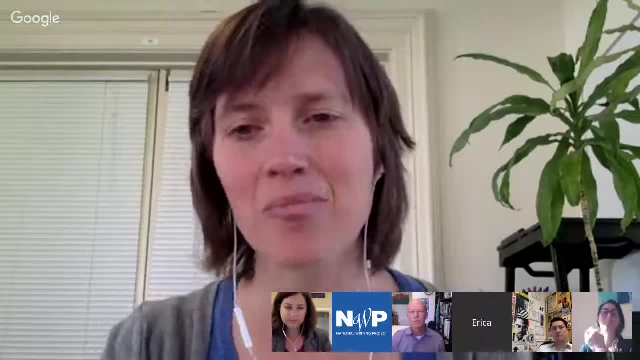 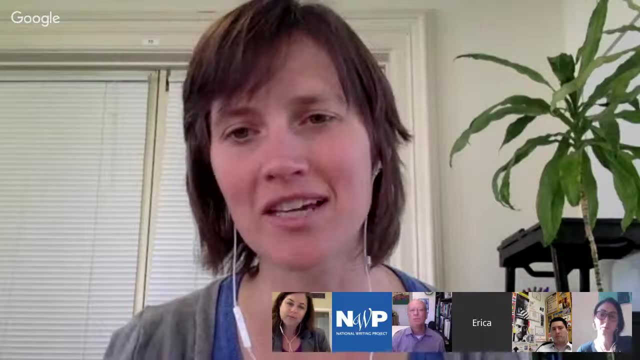 if there's anything you'd want to add to that broadly. but also it just makes me think about how different it is for young people to think about developing their civic and political identity in this day and age when it is so public. I mean, I think there are considerations. 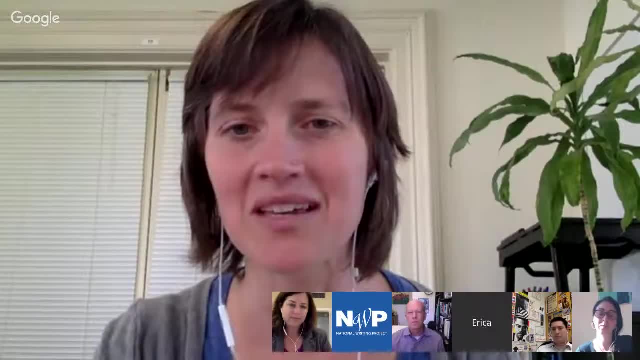 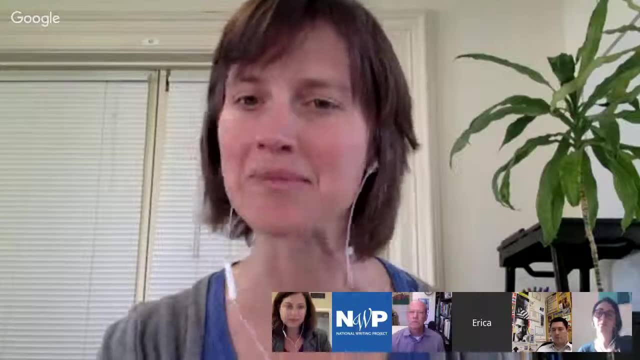 about that pre-digital age, but I also think it is very different in terms of thinking about the sort of afterlife of things that are put online, in terms of young people putting themselves out there in the way that they may see an issue today and what would that mean in 10 years, when it's still there? 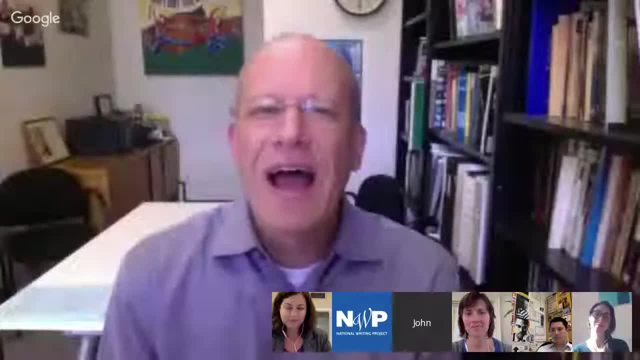 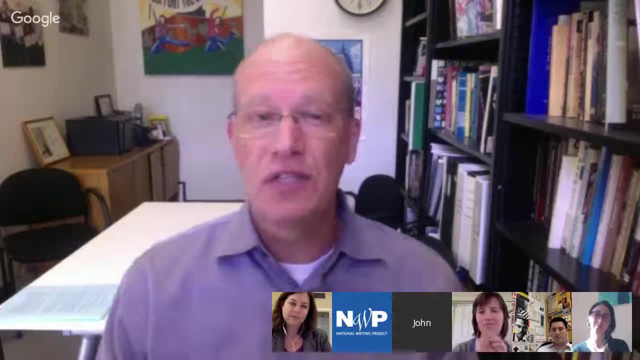 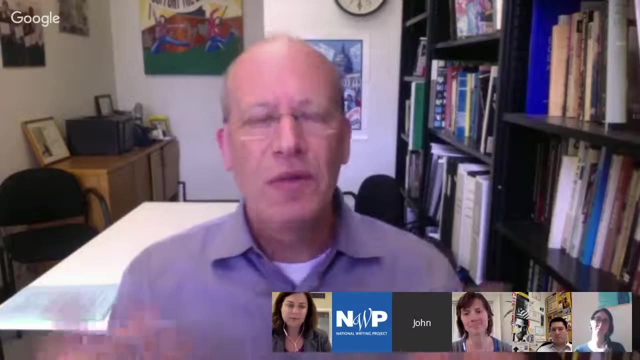 Yeah, I also. it strikes me that the young person, the young person's digital identity, much like the teacher's digital identity, needs to be understood in relationship to civics right. So young people and adults have identities digitally as consumers, as social beings. 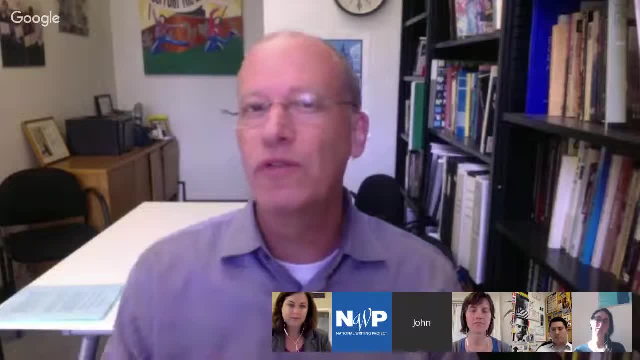 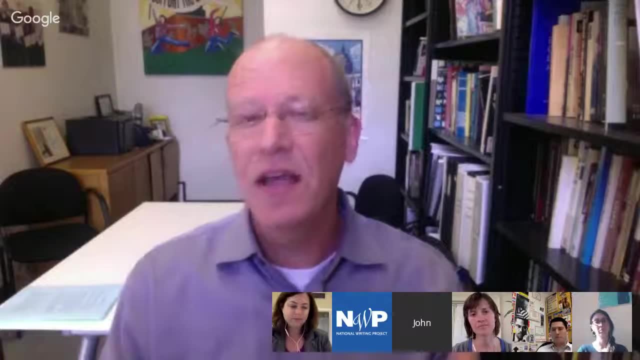 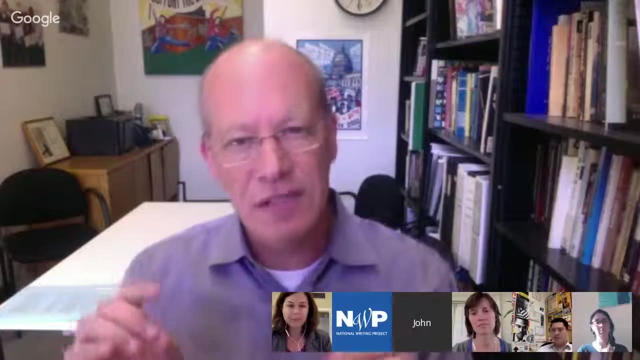 but they don't necessarily have well-developed identities as civic agents And it's really important for teachers themselves to have that identity and then to help young people to reflect upon their emerging identities as civic agents, because I do think that that's distinctive from their identity, say, as a consumer. 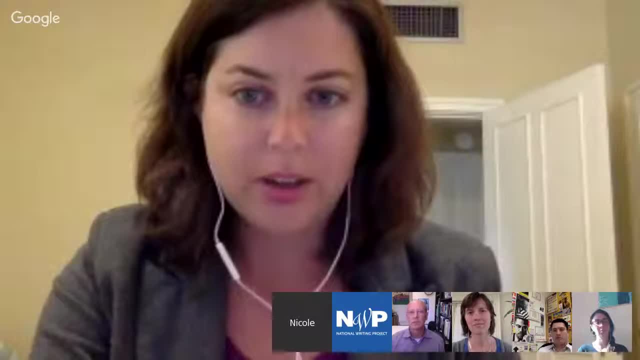 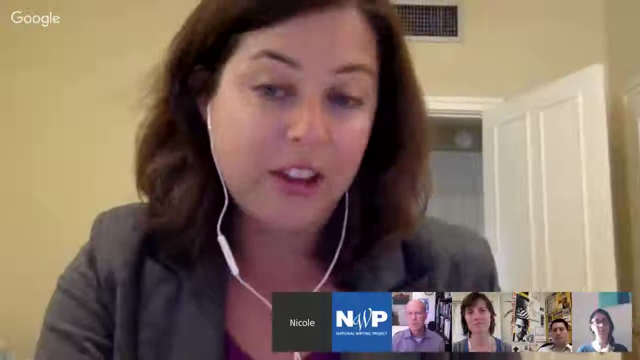 Yeah, and I would add that I think that all of us here are thinking about digital citizenship. I really think there's a lot more that has to be theorized about what that means being a digital civic agent online, because I get frustrated when I go online. 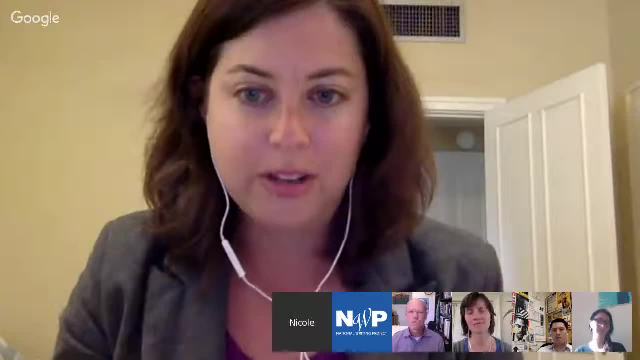 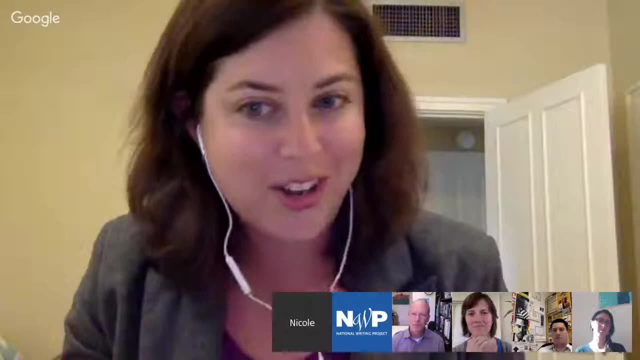 and see that much of what you find about digital citizenship tends to be very much about, you know, not sharing too much. It's kind of like it reminds me, if you're familiar with the Westheimer and Kahn piece that a lot of us talk about, about civic engagement. 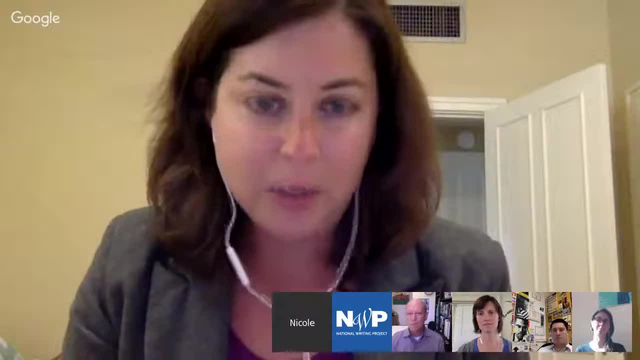 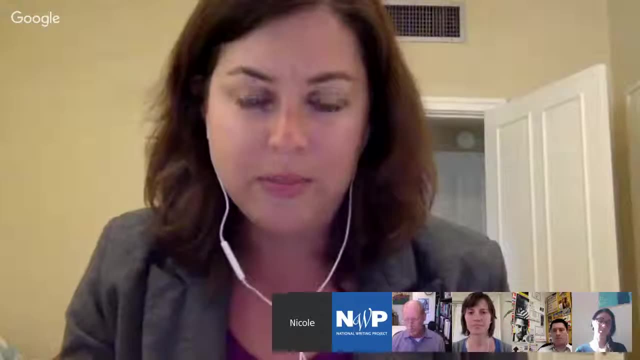 it's more like being a personally responsible citizen online, not bullying, protecting yourself. but it stops there And I think that, Eddie and Perry, what you guys are talking about is that those issues definitely come up, but you're talking about them within an authentic project where it's not just saying: 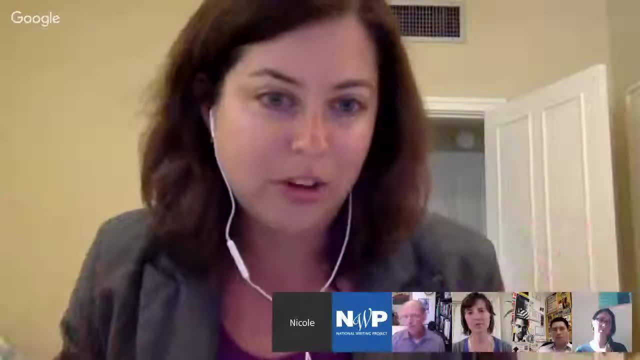 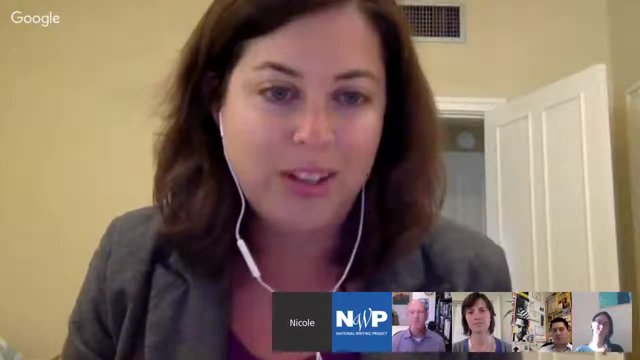 hey, be careful online. it's dangerous out there. don't share about yourself. You're doing it in the context of an authentic project, where there's a reason to have that conversation and have that teachable moment, And I think that's a lot. it makes what you're doing. 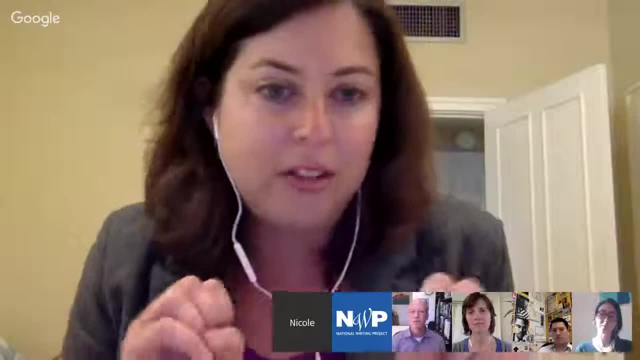 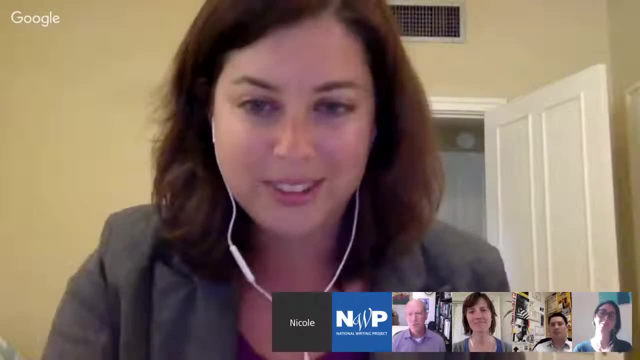 a lot more powerful than just saying: you know those badges you can get online of, just like digital citizen, I'm safe online. I just think that's not the level that we need to get to to get to that civic conversation. Perry, I saw you. did you want to add something? 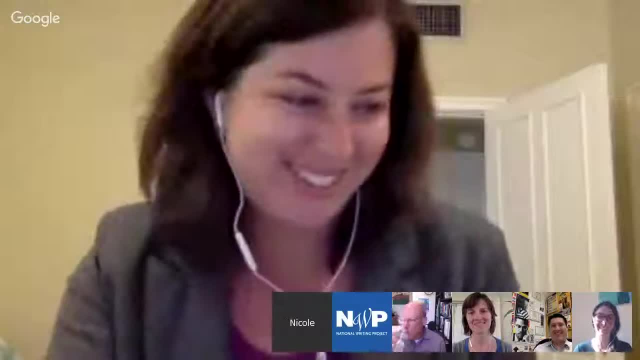 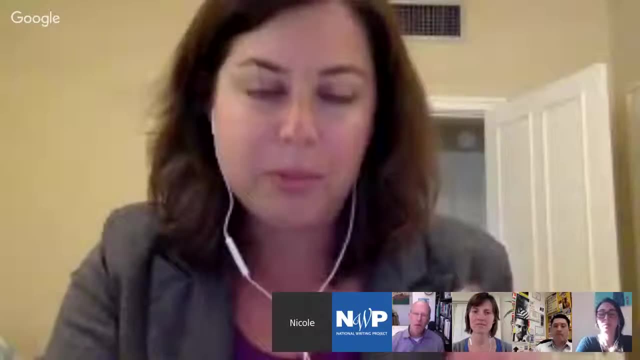 I saw you were on mute, Oh no, But I do want to know. so we do know that we do have the opportunity to connect young people, like Eddie, what you were saying and Perry about connecting to community movements, either far and wide. so I guess I'd want to ask. 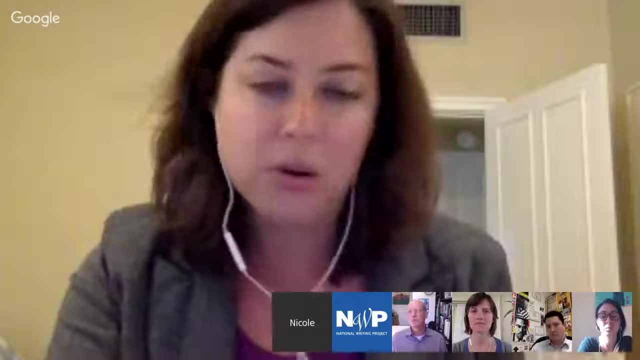 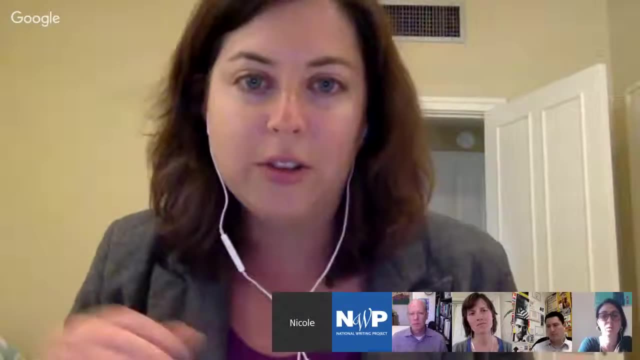 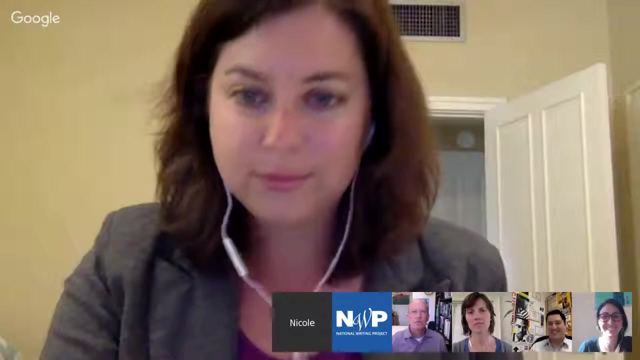 about the ways that you've used digital media or even just used the resources around you in your community to connect with families, to connect with community organizations, and how you manage those partnerships with your instruction in the classroom. Now it's Perry's turn to go first. 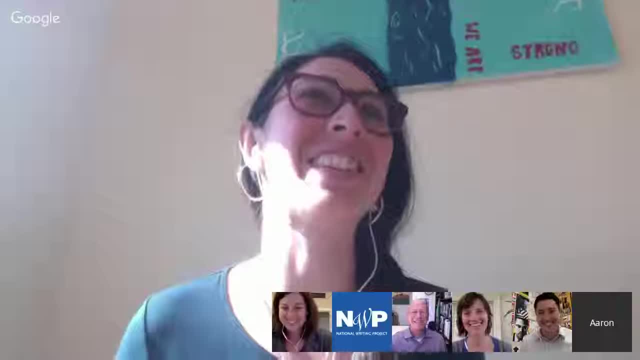 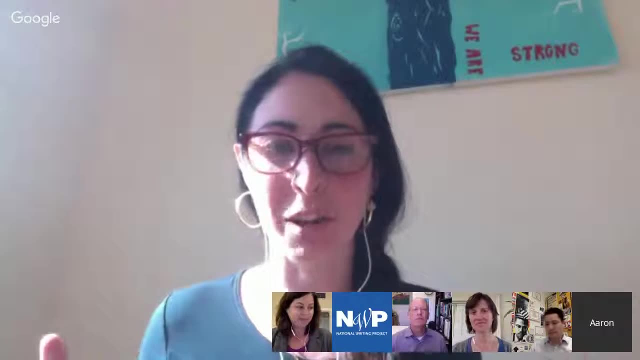 Okay, I'll go. So there's a variety of ways we do that Because I have the privilege of teaching in the context of the social justice pathway, community partnerships. that's built into the curriculum and I have time built in with students in the day. 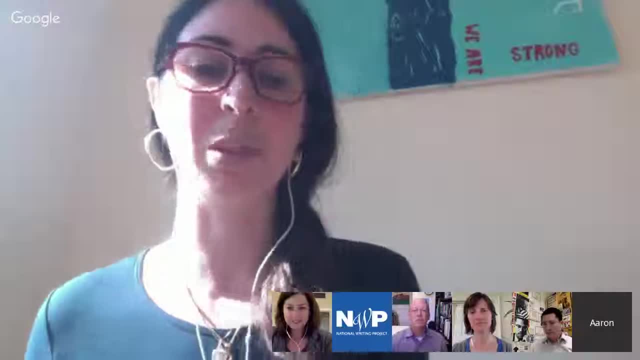 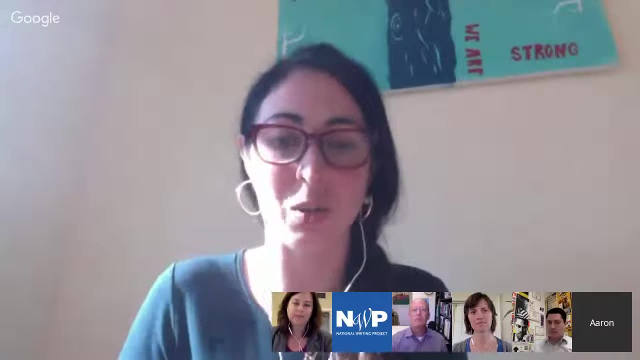 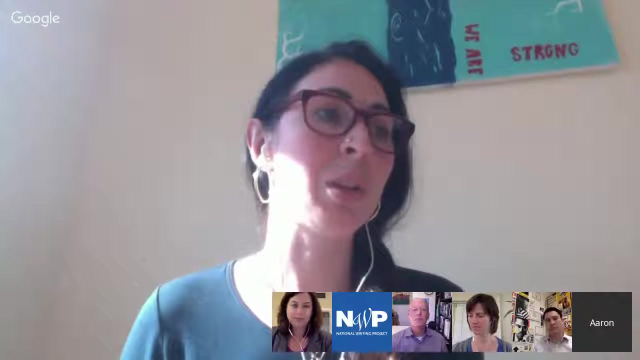 to go out and do work in the field. So it's not always the challenge of having to pull community organizing and that type of work into the classroom environment. We can actually leave the school together to do that work, I think with my ninth graders. 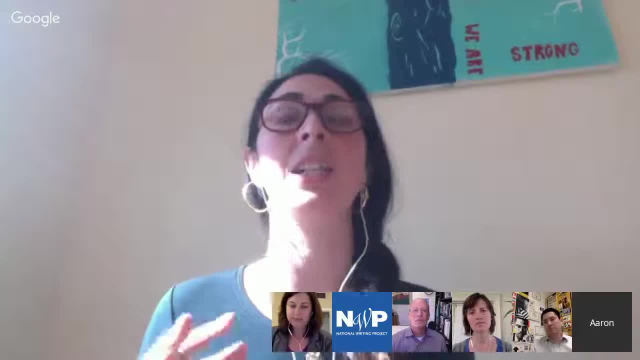 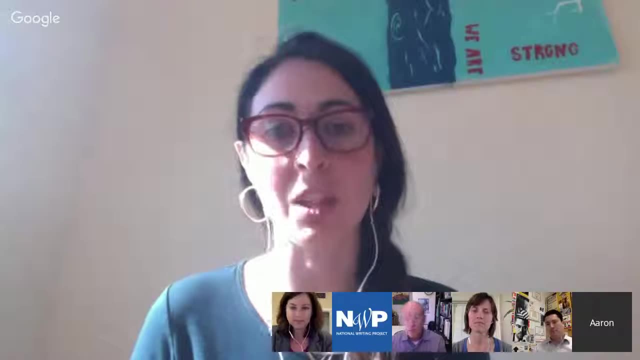 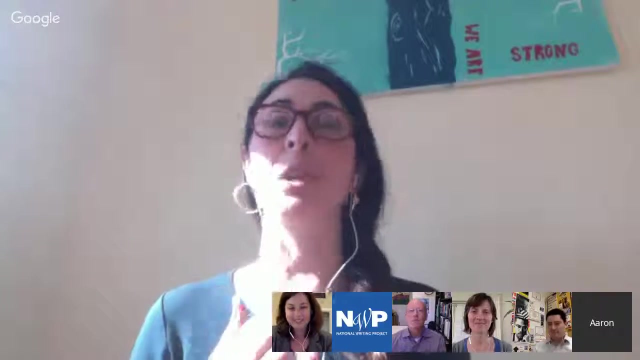 that process looks at different points in the year. We take on issues, and so that tends to look more like having guest speakers come into the classroom, students doing Skype sessions- I forgot about that. That's a digital thing. So if I had students Skype when they were researching? 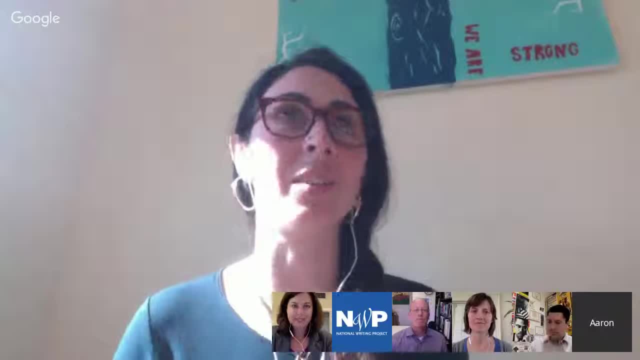 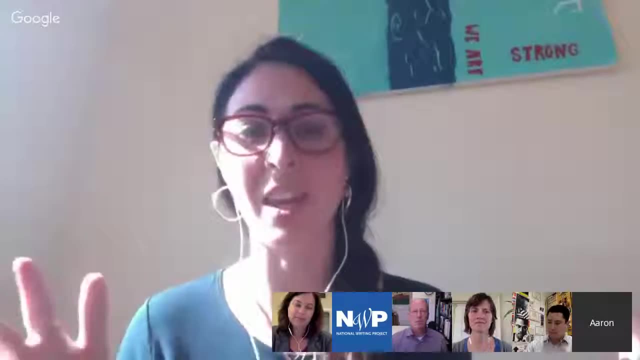 Black Lives Matter, or were researching the Alliance of Californians for Community Empowerment or different community organizations. that they looked at, Communities for a Better Environment and Open right that they decided to look at and research where they were then able to Skype and engage. 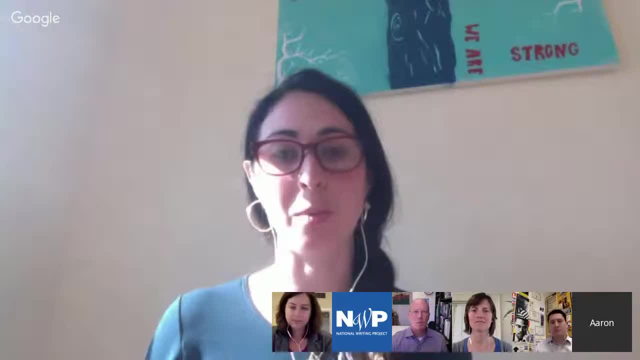 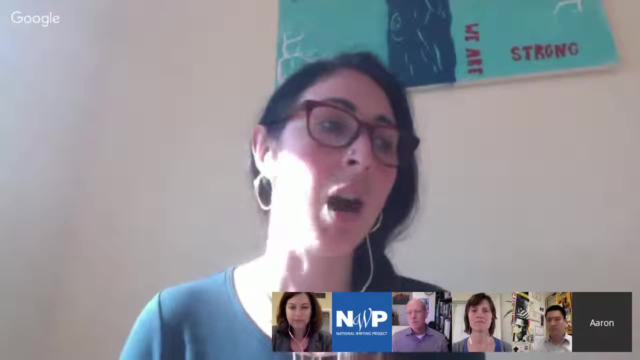 with the organizers and interview them to learn more about the work that they're doing. So that was one way of being able to connect them in. In 10th grade my students go out and do an organizing fellowship. They're working with an organization called 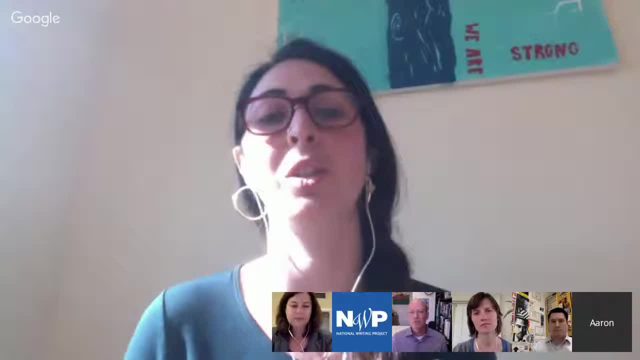 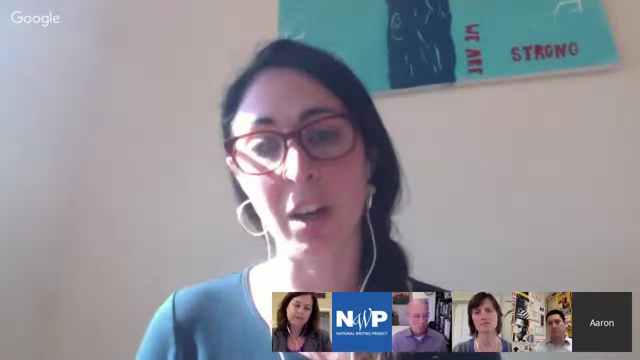 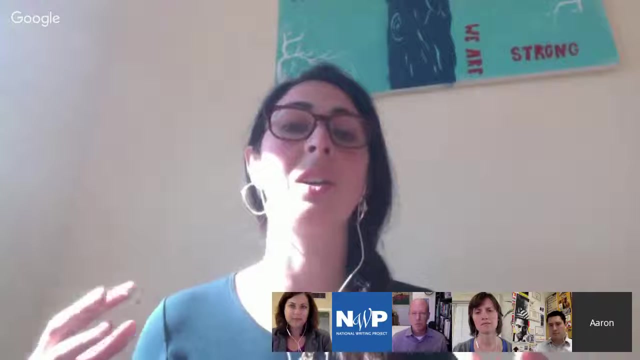 Casa Just Cause and the Alliance of Californians for Community Empowerment working on issues around gentrification, Reentry services for formerly incarcerated people and transportation issues for youth, And so they're going out as part of their school day and door knocking phone banking. 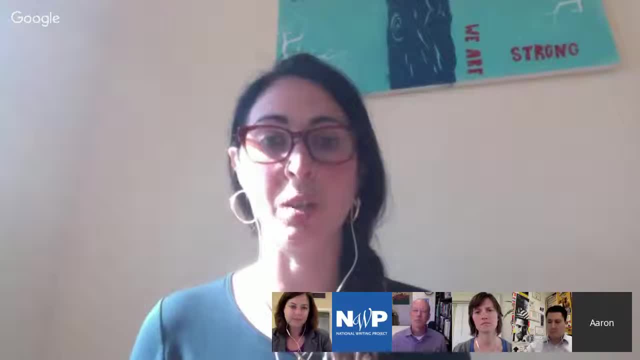 working one-on-one with organizers, helping to organize community meetings and so really learning, kind of this hands-on approach of what does it look like to apply the theory that we learn in the classroom Like we do a whole series where we watch all these films, kind of like Eddie was talking about? 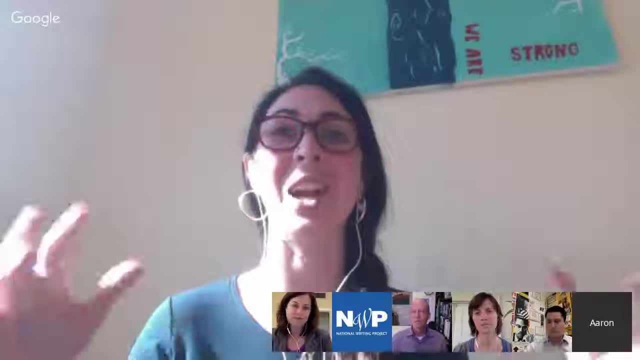 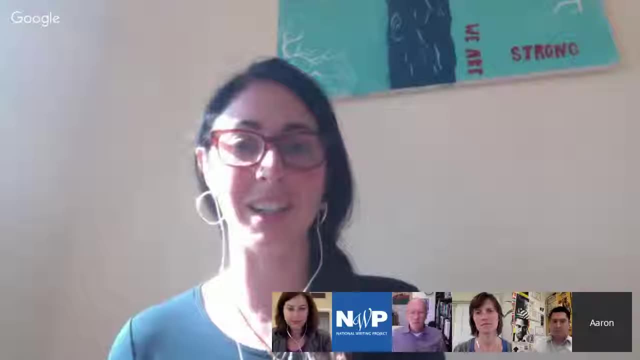 of youth-led movements historically and they analyze the tactics and the strategy of those movements and then now they're applying it and saying, okay, this is the issue we're trying to solve. How do we use these tactics that we've seen? 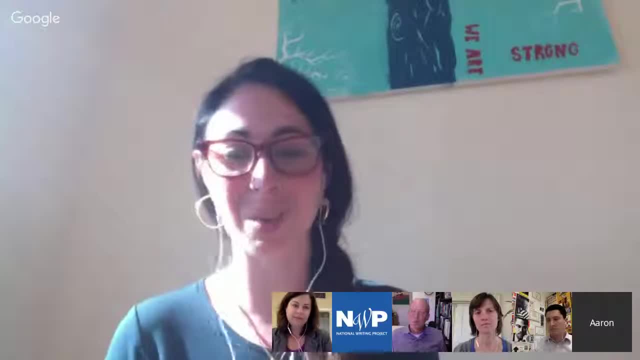 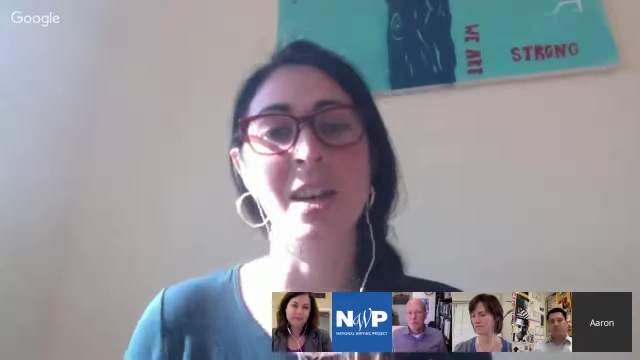 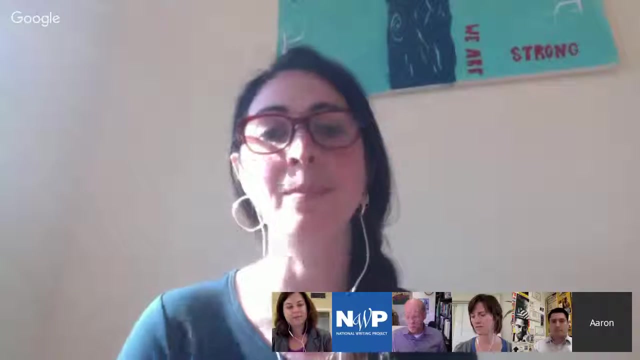 in our film study, or these activists that we've interviewed in the past to get laws passed in Oakland to protect tenant rights, And so that's one way. So there's kind of that applied aspect to it that, I think, is what makes it meaningful to them. 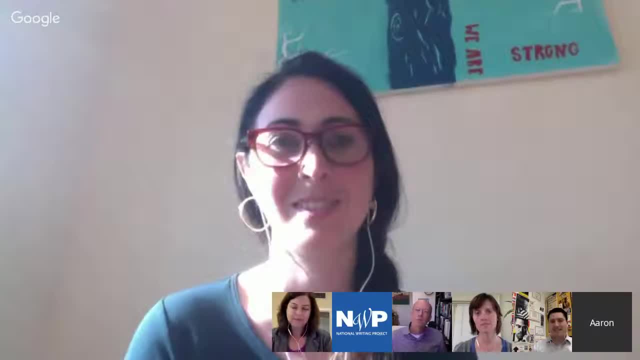 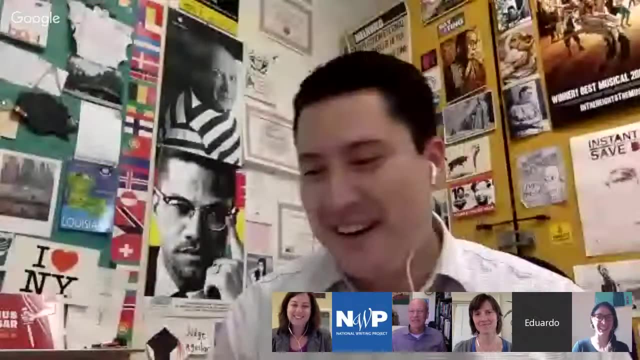 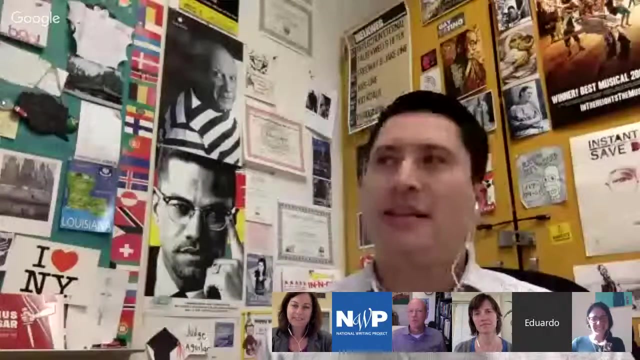 not just academic coursework. That's all right, Eddie. Thank you. Yeah, there's just so much right, I guess, when thinking about creating partnerships- advice that I would give teachers- it very much has to align. I would say: 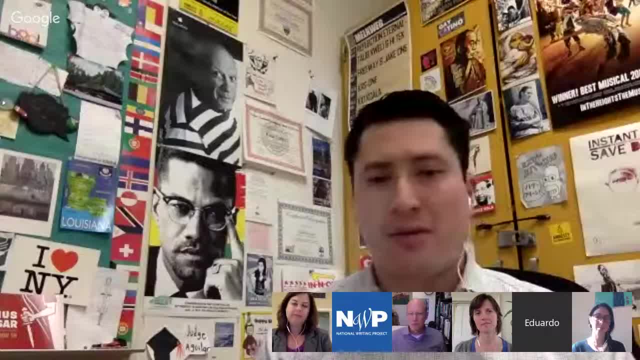 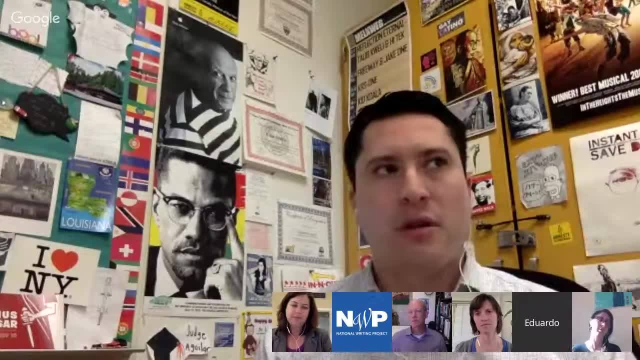 with what the focus is and whatever project, like Perry was referring to, because there's so much sometimes that we have our students involved in, As a teacher, just finding those allies within the campus, within the community, with parents, and establishing these relationships. 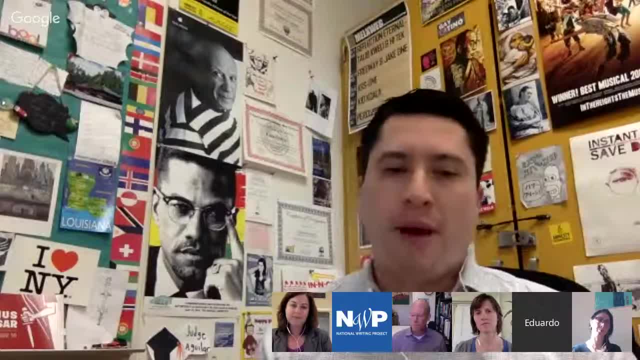 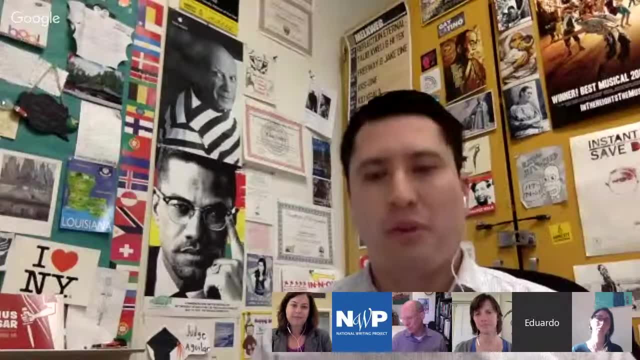 and making sure that you're nurturing them. so they're ongoing. I think oftentimes at schools we have folks that come in and it's a one-and-done deal, and so you don't build community with those folks, You don't build longevity. 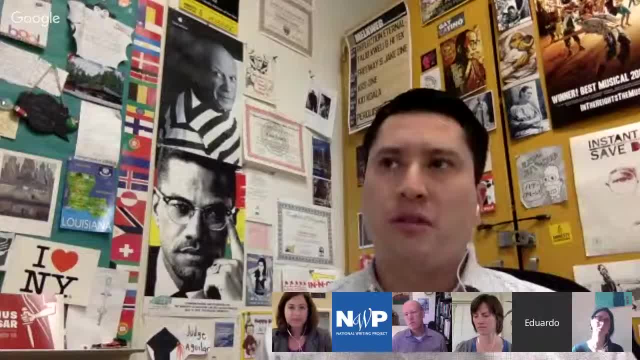 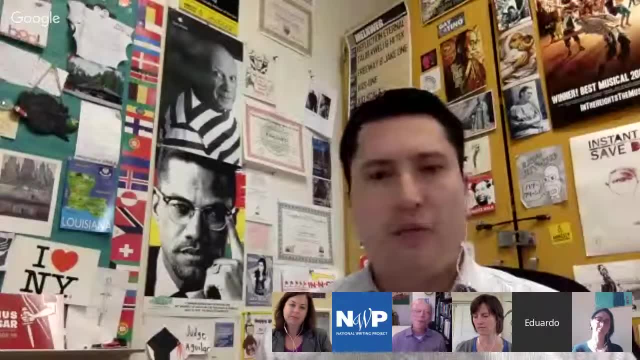 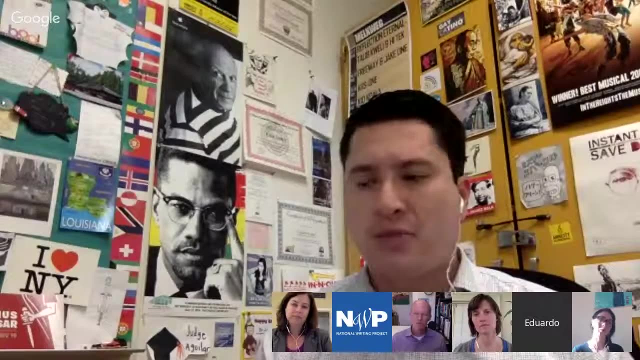 You build longevity and continuity, and so I think students are very observant to know those type of organizations, and so I think, in terms of creating meaningful partnerships, there's got to be some real stakes and accountability on all ends, right? I think a lot of times we put so much of the onus. 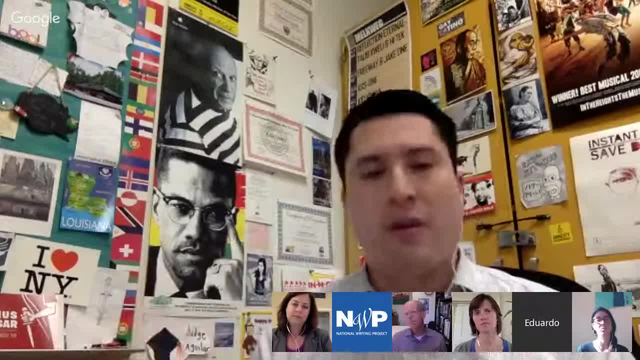 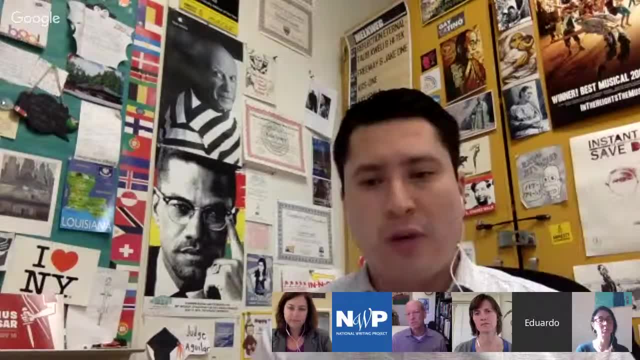 on the young folks, but I think it very much has to go back on whoever we're creating those partnerships with. For myself, for one example, so with I run a program called the Urban Scholar Compadres. It's a 9th grade. 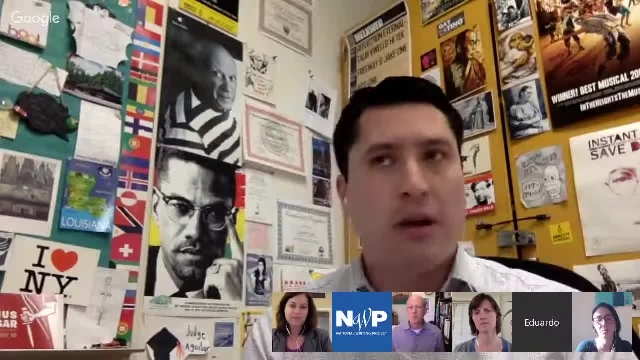 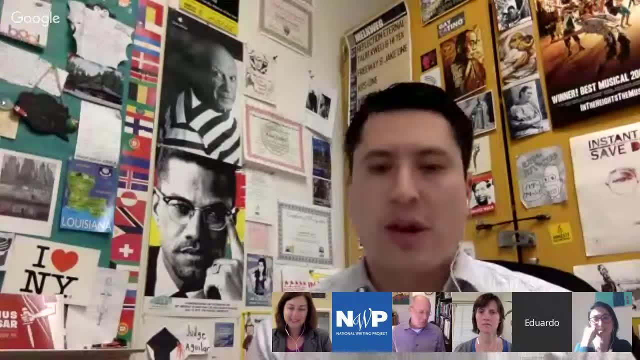 I mean 9th through 12th grade. young males, young male ethnic studies focus curriculum with a YPAR component, which Nicole was referring to, the Youth Participatory Action, Research. And so I got my schooling working with Nicole, with John Rogers and other folks. 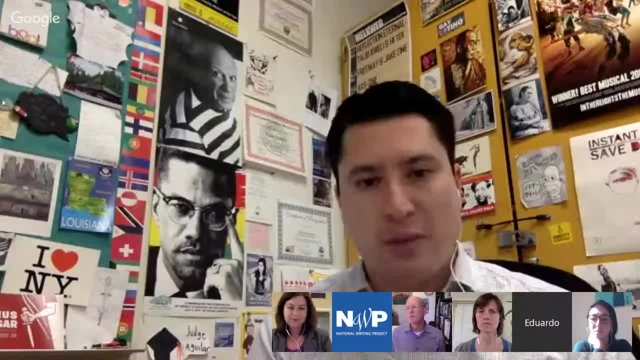 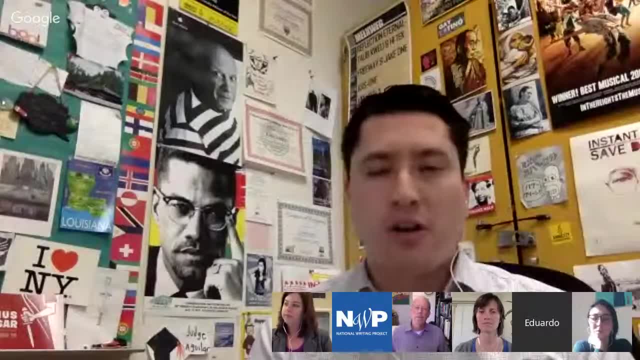 and so I've found ways to incorporate YPAR into my classroom And so, for one example, with my young men. every year we started. well, now it's going into our fifth year, We have an event called the Bowtie Event, and the idea behind it is having the young men 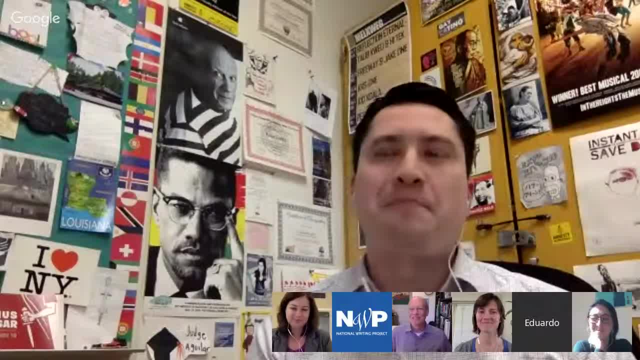 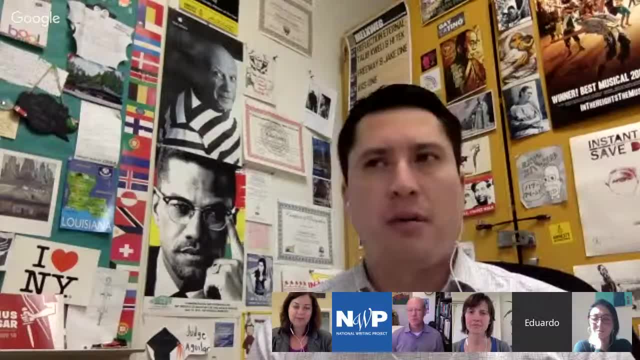 wear bowties right, so dress up that day and we have a motivational speaker come and speak to them, We have them invite their mentor and a lot of times, especially in our communities, we never really formalize, you know. 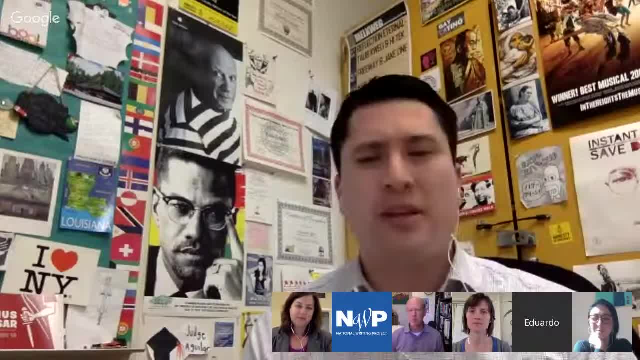 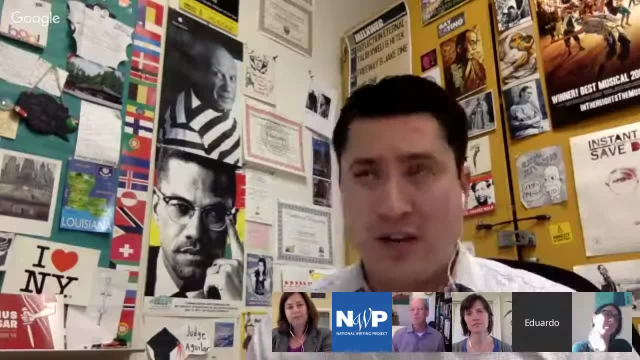 like: you're my mentor, I'm your mentee. It's just more informally, and so it's kind of recognizing that and trying to nurture that relationship And so whoever it may be, it doesn't matter in terms of gender. 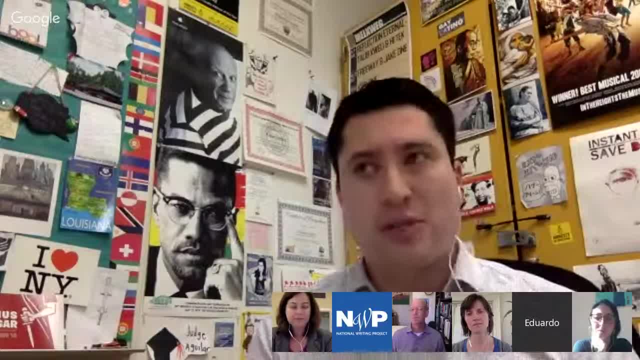 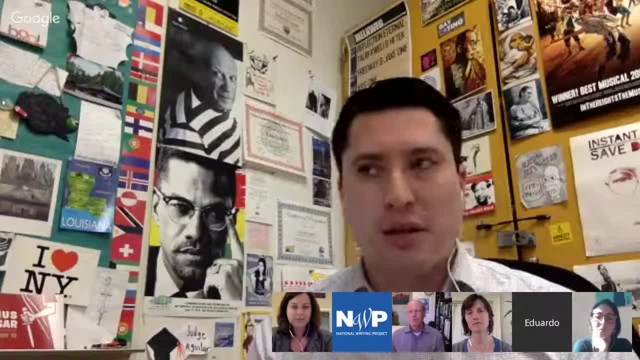 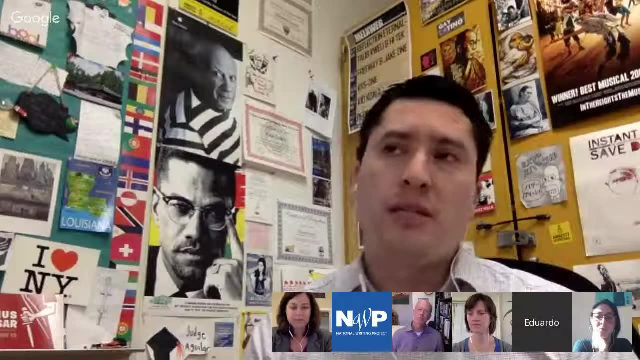 we invite these folks, But in the process of doing this, we've created a great partnership with the Parent Center at our school and so who typically tend to be a lot of the moms on campus of students who their students are on campus. So these parents now look forward. 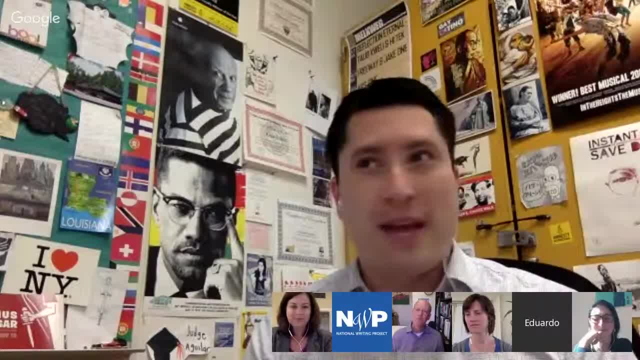 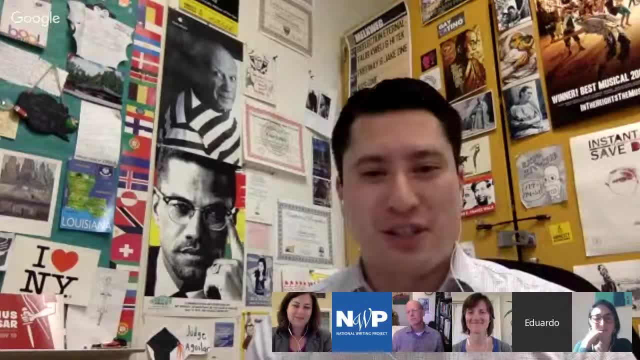 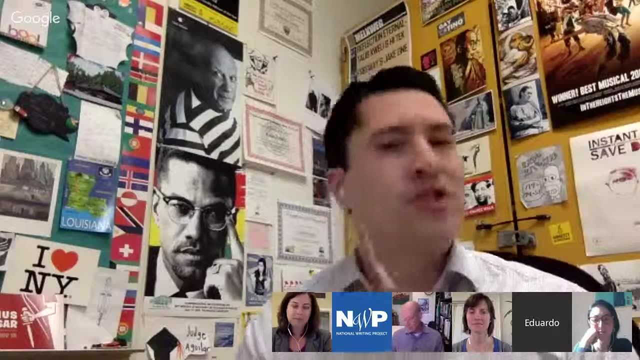 to this event every year. If it wasn't for them, a lot of it would not be done as far as just making logistically the location look beautiful, in addition to kind of, you know, working on bringing the food, the beverages, making it just work right. 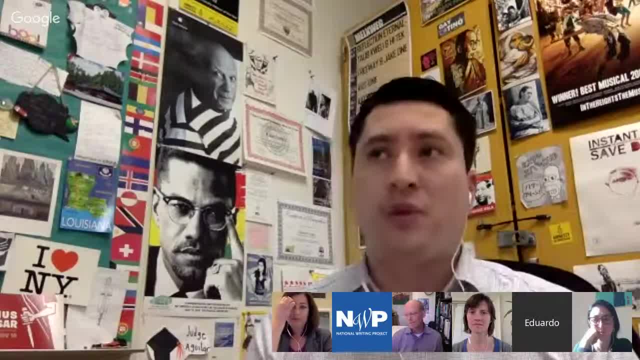 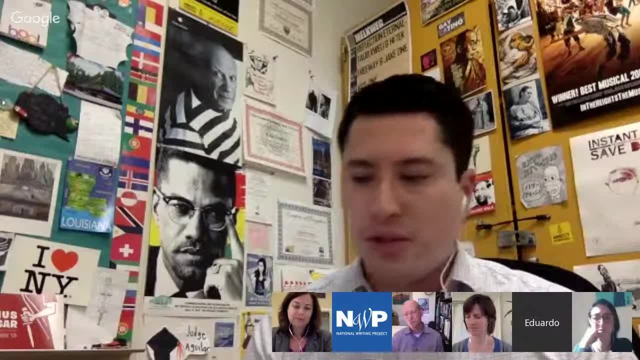 And so, even starting off there now, we've had opportunities where we bring in some of these parents to come and speak to our young men, especially when we get into feminism and we get into issues of, you know, family and the role of young Latino male. 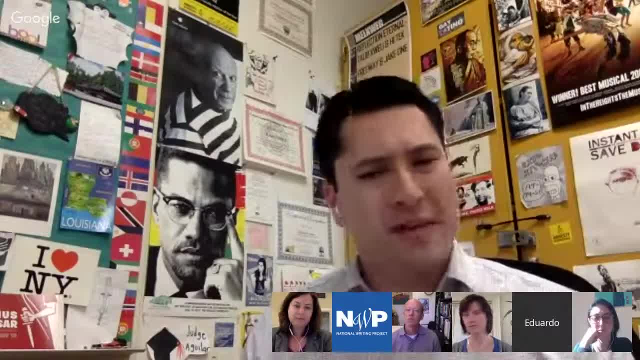 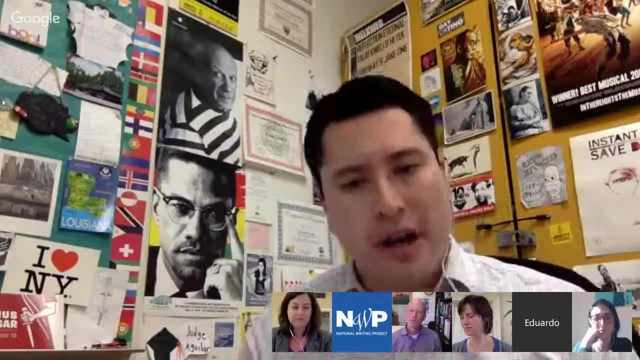 in our community, And so that's just kind of an example of how we started off with one event, the Bowtie event, but now it's grown to mean something else, where the mothers are now connected to what we're doing in the classroom. 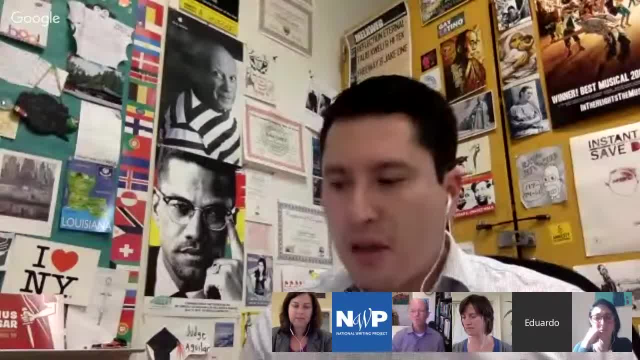 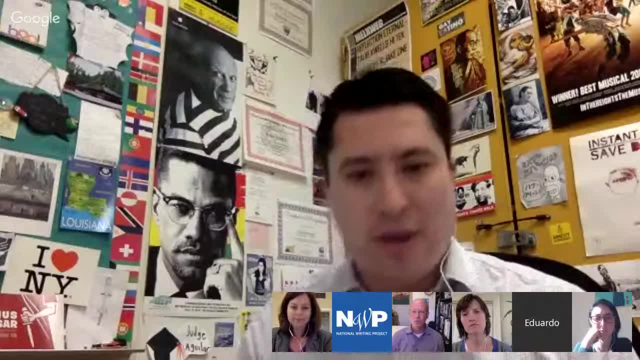 which is extremely powerful. And another partnership that I would say in terms of the community that we've created is working with the Social Justice Learning Institute. It's a nonprofit Headquartered out of Inglewood, California, A really good friend for a lot of us in the panel. 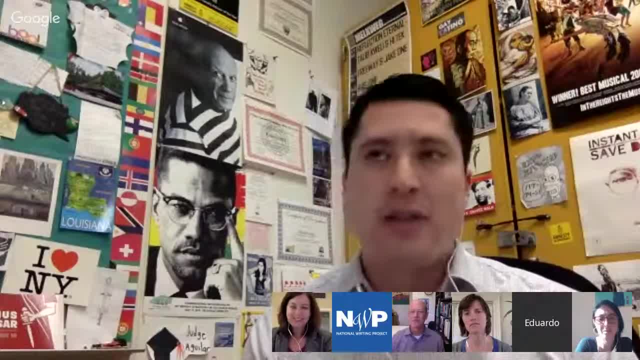 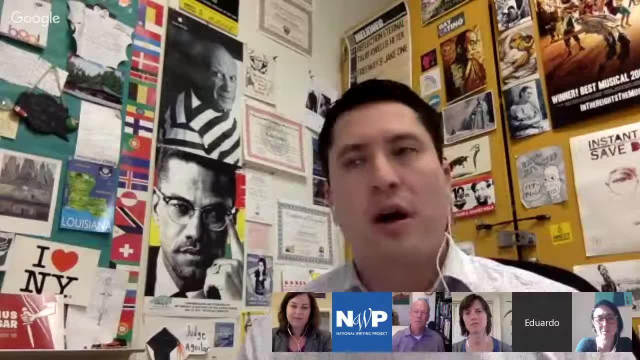 Dr D'Artagnan Scorza started this nonprofit and it started looking at young black males because of incarceration rates, recidivism, et cetera, et cetera, And so, working with him, we actually expanded and we get support. 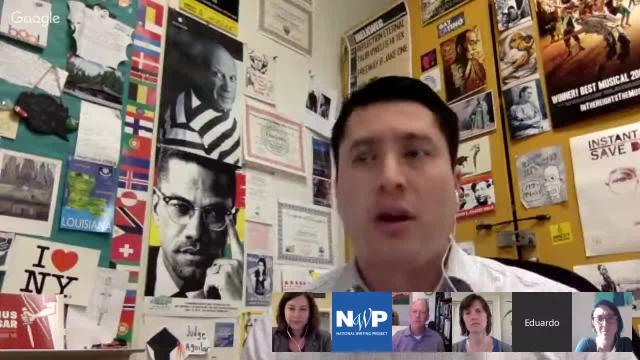 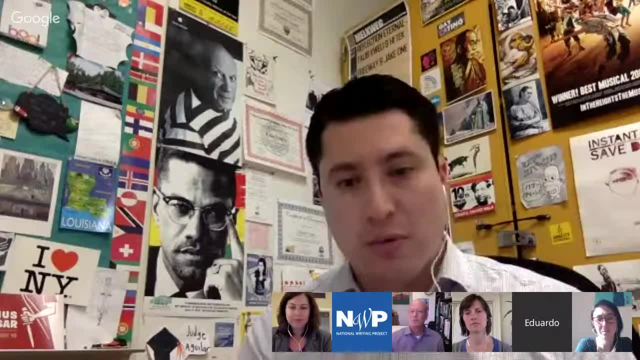 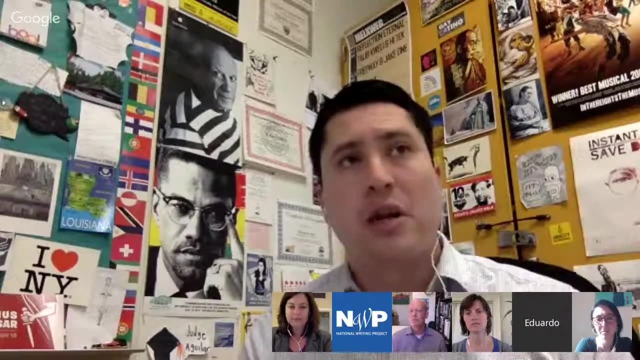 through the Social Justice Learning Institute with our young Latino males here at Roosevelt And that's allowed us a lot of additional support and ongoing support. where we have a college representative or a rep that they have in their office that will focus on making sure that our young men are not just graduating. 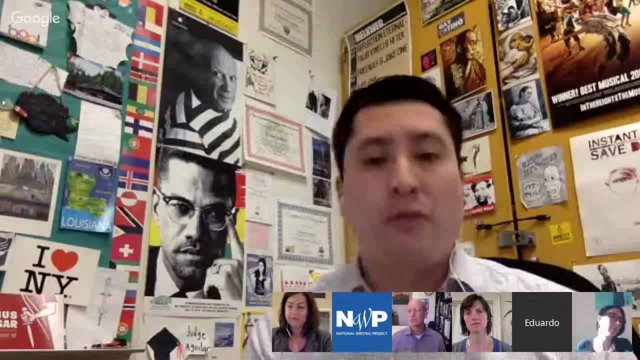 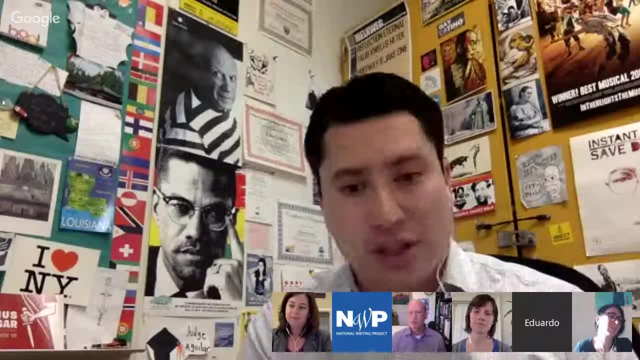 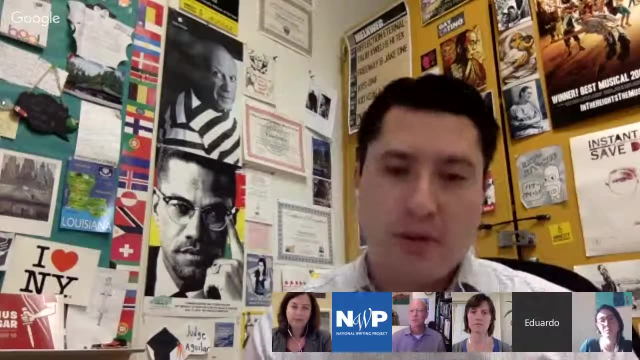 but going to college or getting ready for a vocational career, And so this is something that we plan every year, as far as including it in their budget. There are folks that provide us with retreats up to Big Bear to build community, And so these are the type of partnerships I think. 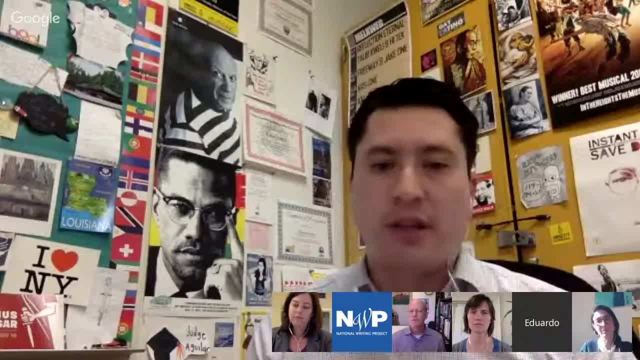 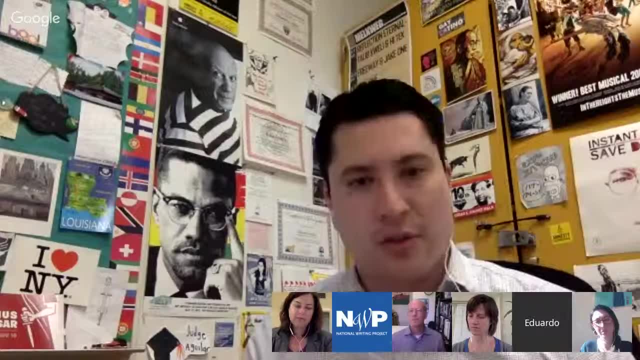 that I sought out But fortunately I've had folks respond to these invitations and it started really small and then it's continued to grow. And one last one that I'll make a plug in as far as another partnership because of the focus right. 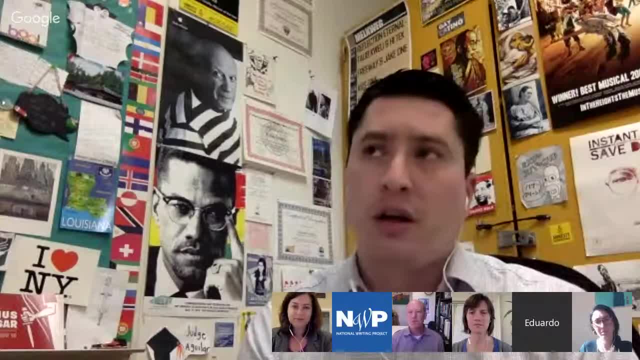 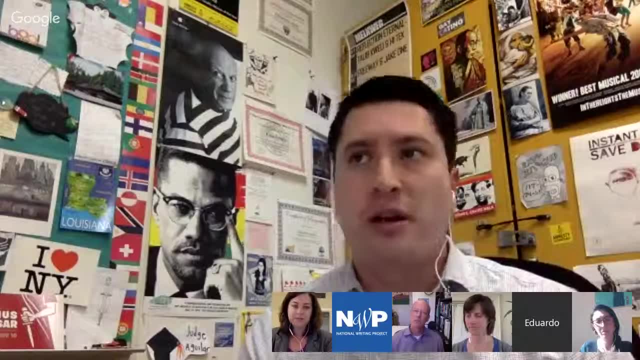 So one of our YPAR research project focus was on just the incarceration rate of Latino males specifically, and the high dropout rates and the association of, or the statistics that if you drop out, the probability that you'll end up in prison at one point or another in your life. 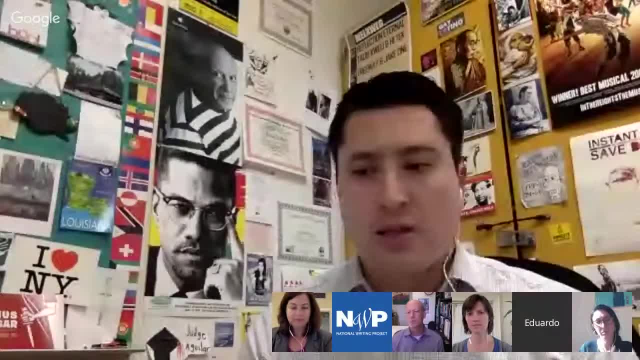 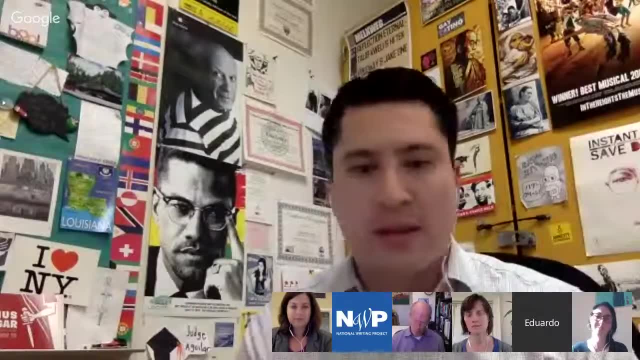 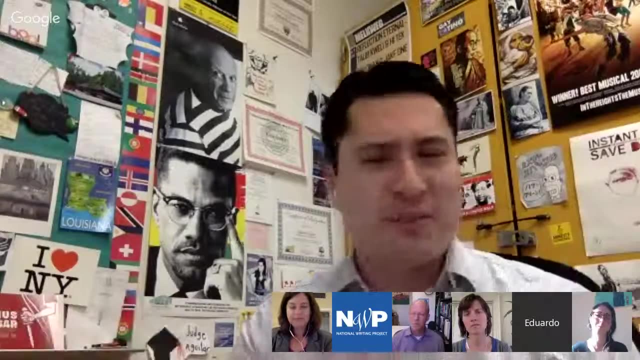 And so right over the bridge from where we're at is Homeboy Industry, which is the largest gang intervention rehabilitation, reentry program in the nation, And Father Greg Boyle has a strong connection to Boyle Heights. There's no connection in terms of the name. 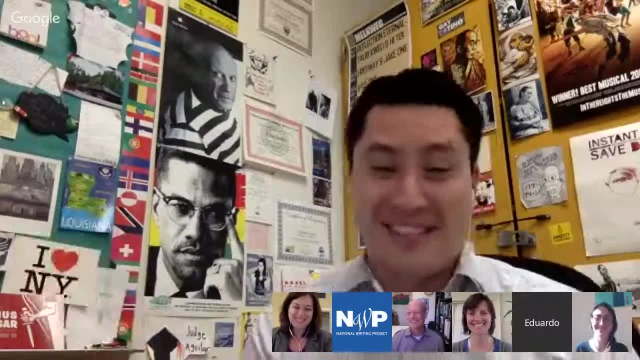 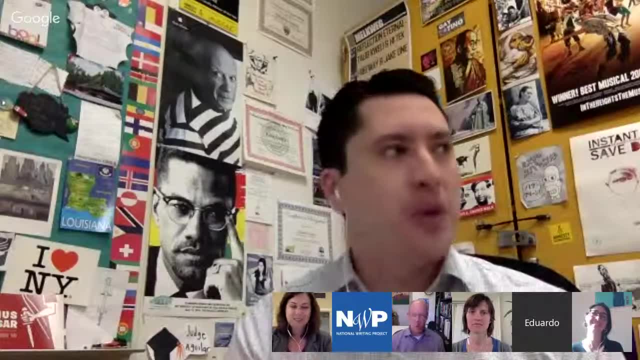 A lot of students think like: is that the reason why they call him that? It's like? no, that's his name, And so we've begun a partnership with Homeboy Industry. He's donated a class set of Tattoos on the Heart. 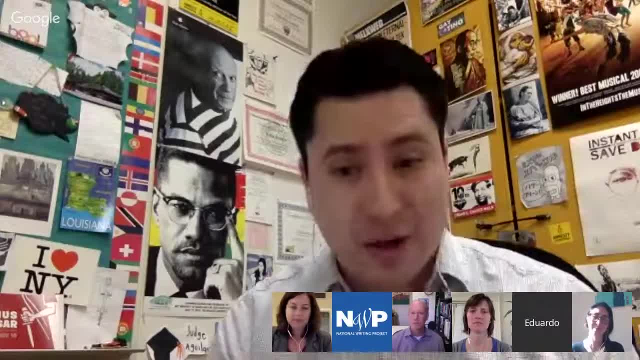 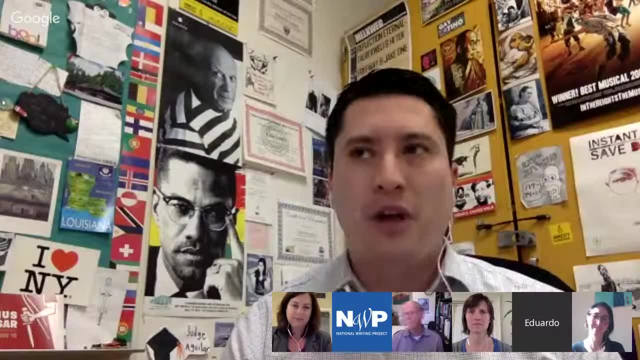 which is a great book that he wrote. So we embedded that in the curriculum And this all started with just going on a field trip out there, And so I think it starts really small And as long as you approach them, as far as I know, with Perry right. 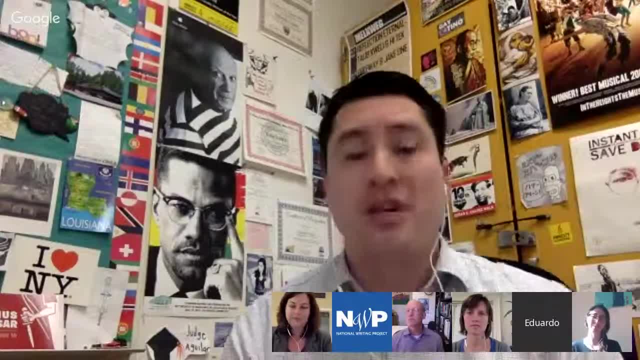 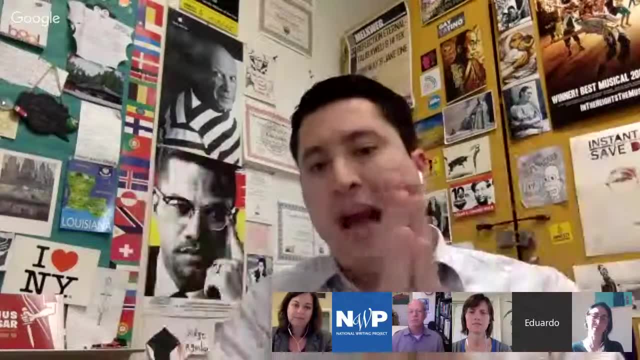 with the work that you do. I can imagine, right that there's organizations just wanting to help you out, right, Like they're in a sense like willing, but it also has to be, you know, we meet halfway where you know. 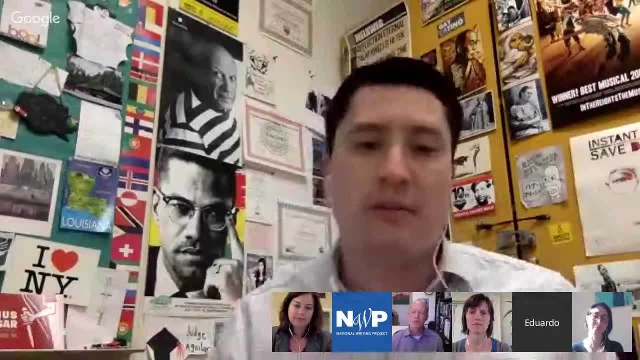 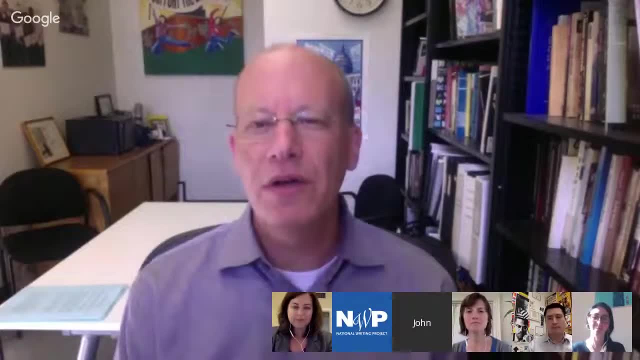 we're coming out to them and showing interest as much as they're going to put in with us. Can I just ask a quick follow-up question to Eddie? I'm curious, given the distance between East LA and Inglewood, have you used social media? 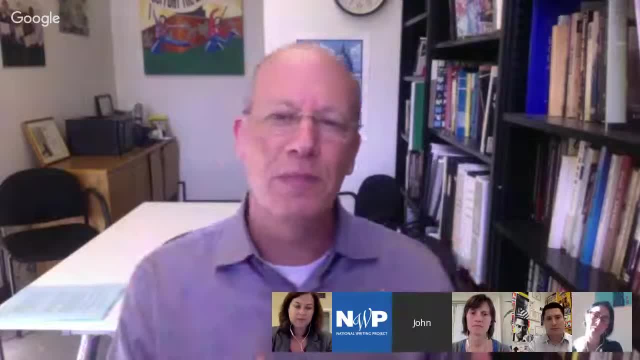 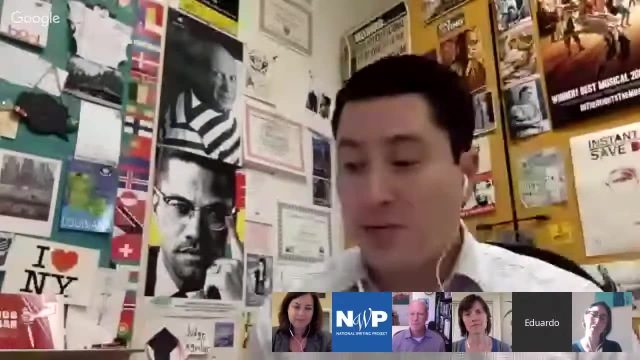 as a way to connect the young people you're working with with the young people that Dr Scorse is working with in Inglewood. Yes, that's what we're actually moving towards now. right, We're getting to kind of the level where Perry's at. 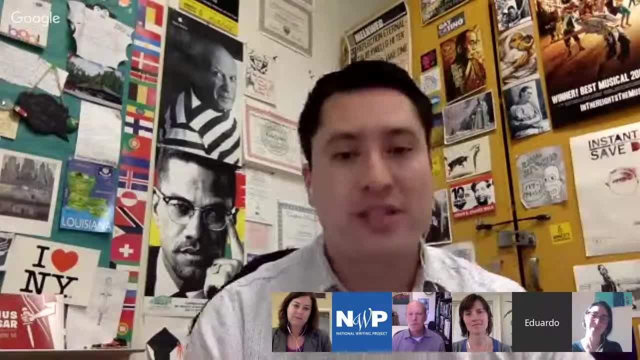 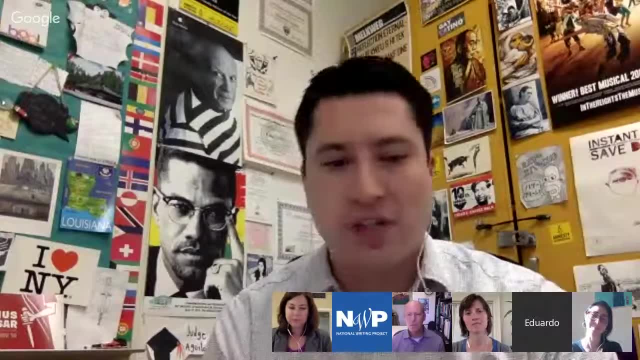 where we're actually blogging on the Social Justice Learning Institute website. So now they've started not only a Facebook page, which again you know we have to have those conversations every so often as far as you know what folks are posting, right. 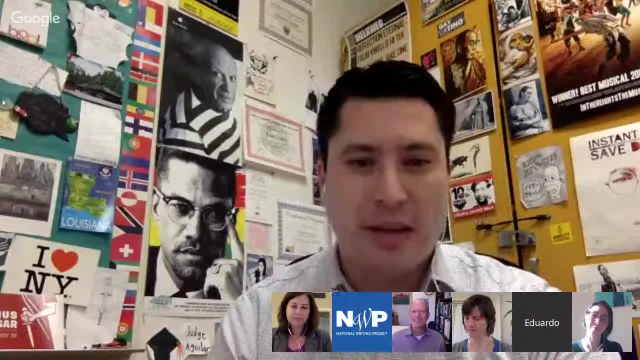 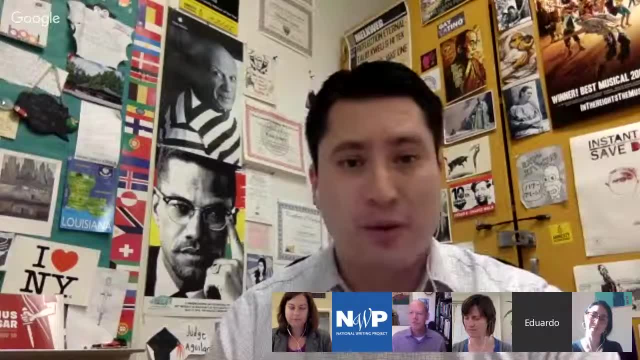 and how appropriate you know the things that they might be saying in that public forum. But we also are now finding ourselves in Google Hangouts, just like what we're doing right now, where we're trying to bring you know folks together during our class periods. 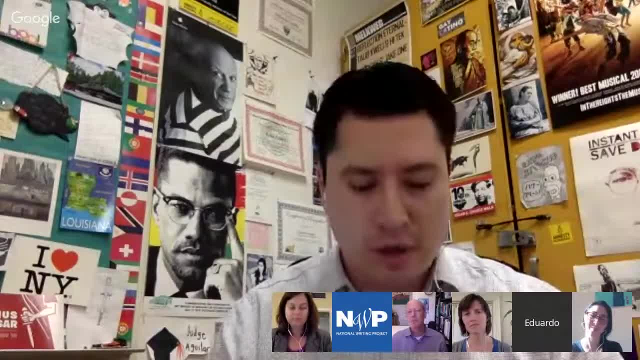 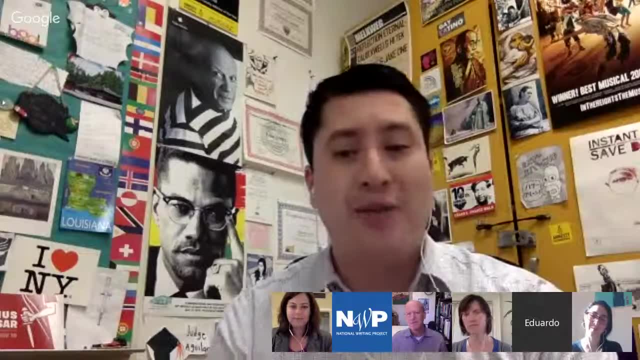 or after school, to continue. you know some conversations that we've had when we've been brought together Because, as you mentioned, going from East Los Angeles to Inglewood is about an hour traffic, And so it's not too often that we get the opportunity. 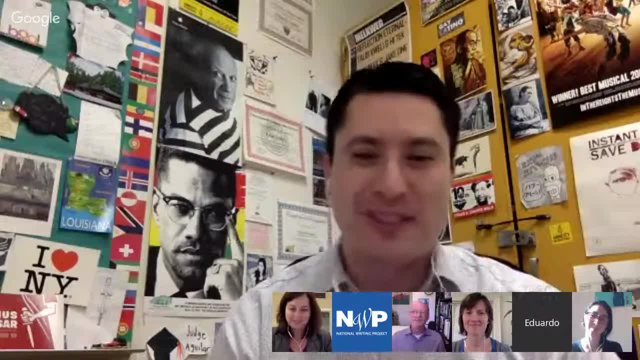 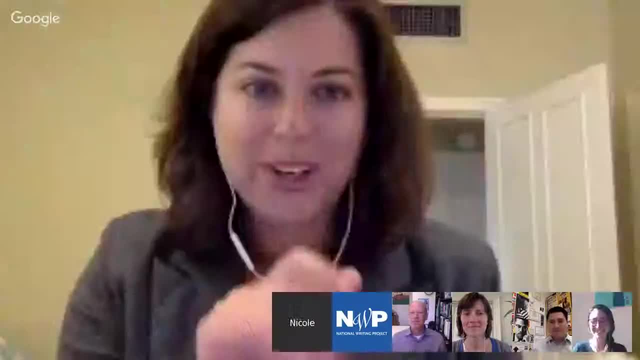 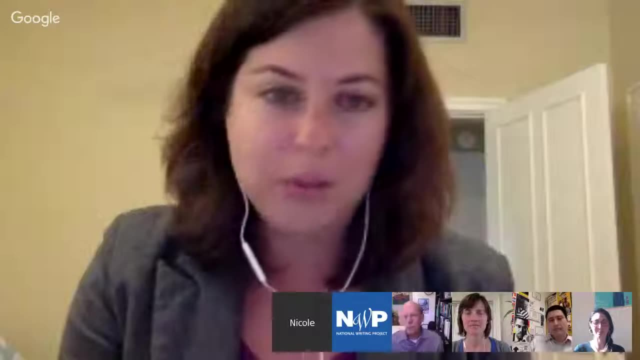 to go out there and mingle with the folks. I'm also- Oh sorry, go ahead, Perry. I was going to ask you and Eddie a follow-up as well- about you know, teachers that might think that this is work that's above and beyond. 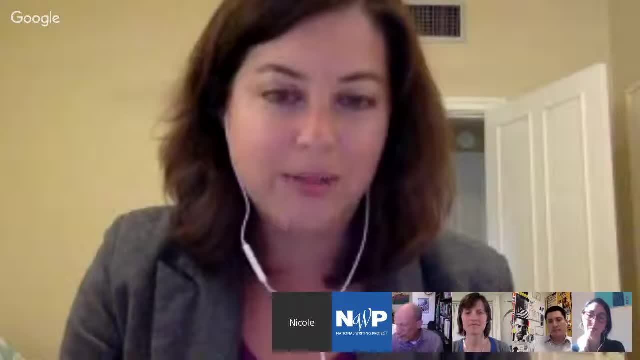 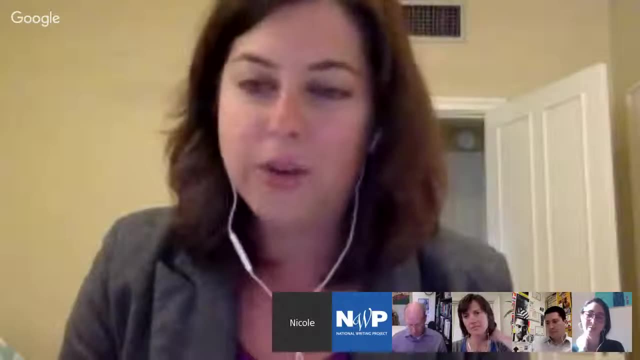 the work of academic teaching and how overwhelming it can feel if you're a new teacher or if you don't have the networks that you two both clearly have in your communities And just kind of how you would, And also one thing that goes along with that. 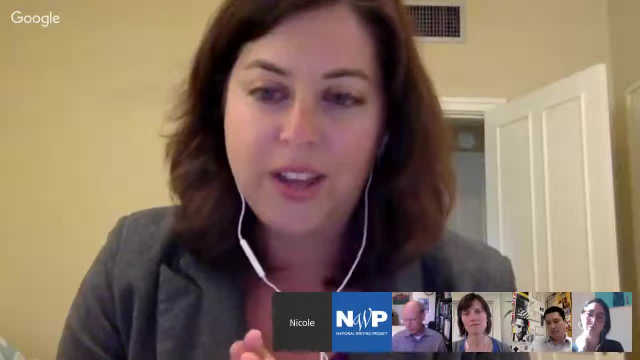 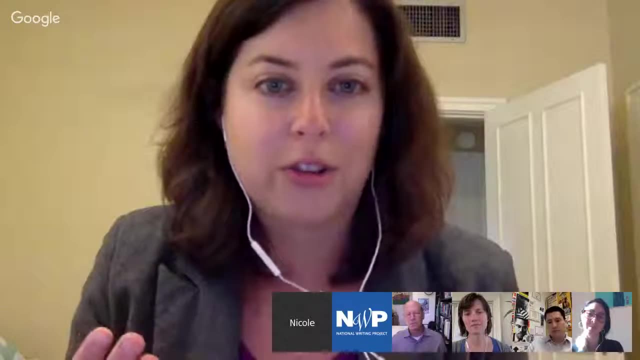 is the fear sometimes that I hear from teachers about, if they acknowledge that they are civic beings that have opinions and belong to different organizations, that somehow that means they can't be objective, They can't be positive teachers or they're going to be proselytizing to their students. 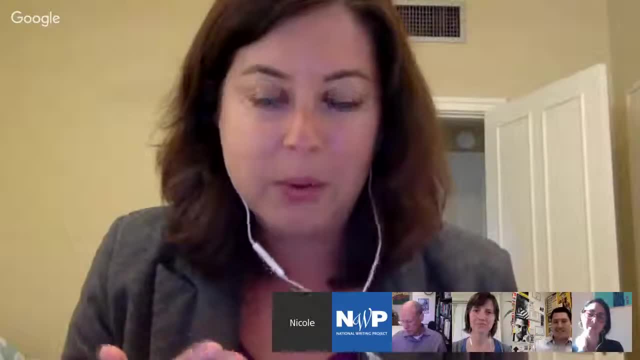 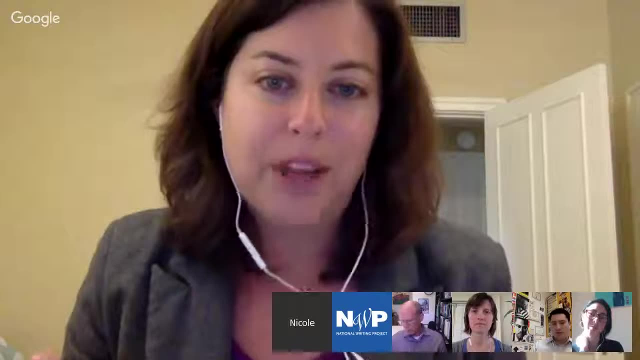 the stuff that people get worried about. So how do you, number one, counsel a teacher who maybe isn't sure how to start getting involved in these partnerships? And, number two, how to not be afraid to even talk about controversial issues when it can seem like you're trying to bias students. 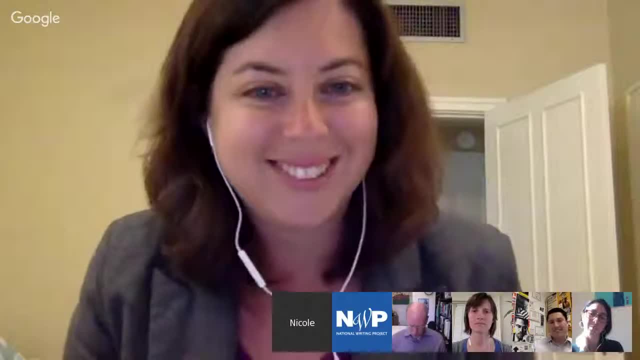 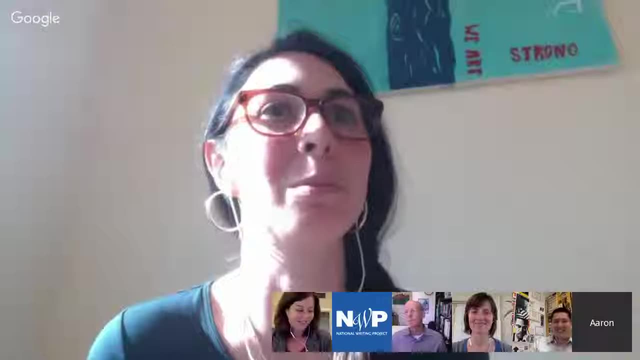 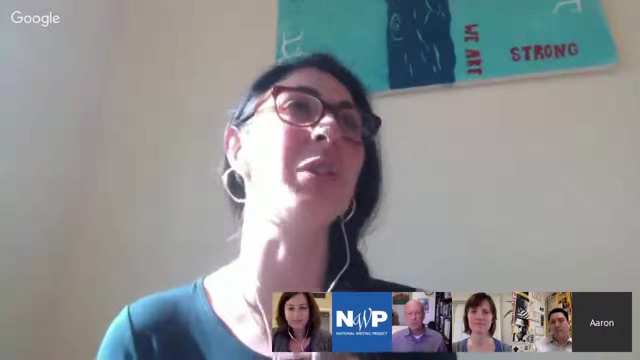 even though you're not and you're just being a human being. That's a big question, I mean. I think that my most basic response to that is that it is really challenging messy work. There's not. I don't feel like. it's like. 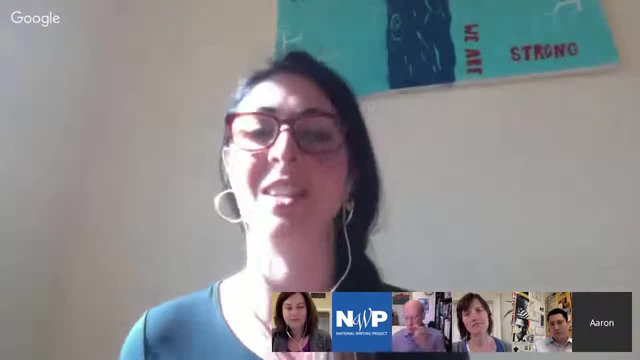 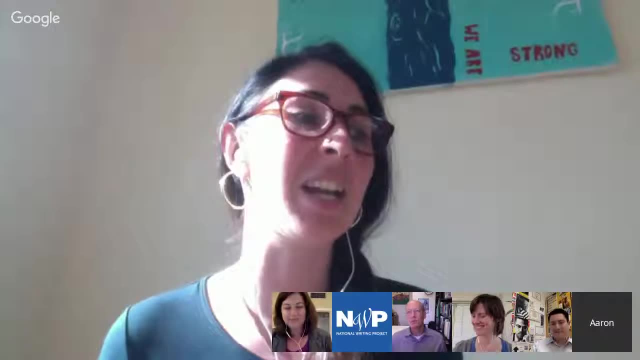 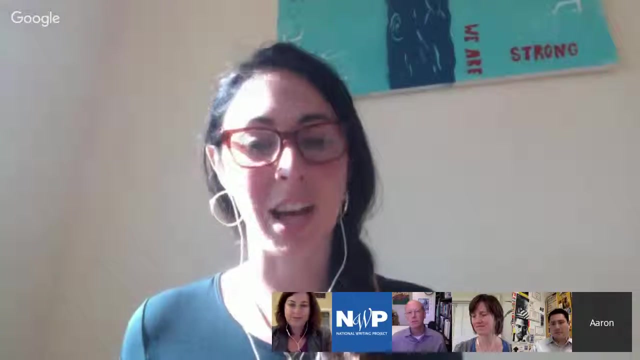 oh yeah, totally you should do this. This is the easier way to teach, It's not, It's the most fulfilling. I mean it's deeply fulfilling And there's, And it's not just Students are bought into classrooms. 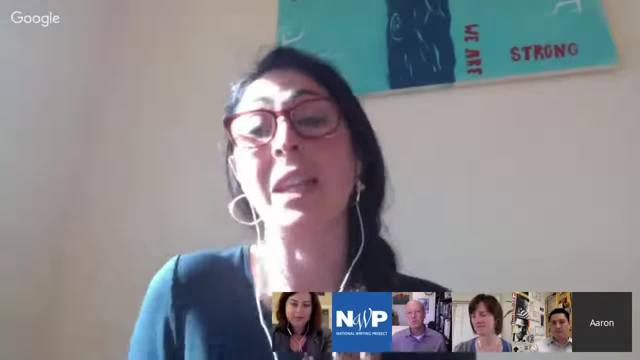 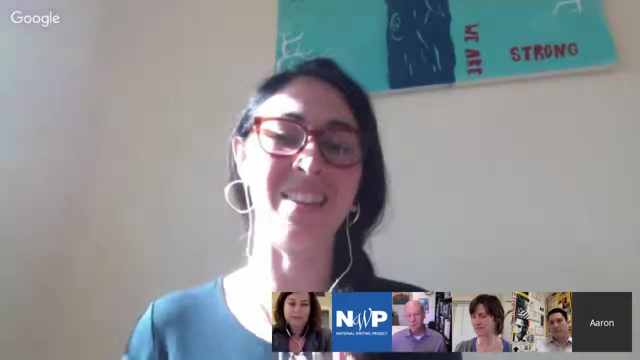 and academic experiences when they really get why And when it is meaningful to them and relates to their own lives, and that gets like. I feel so blessed to be able to teach content and teach in a way that You know. there are things that I struggle with. 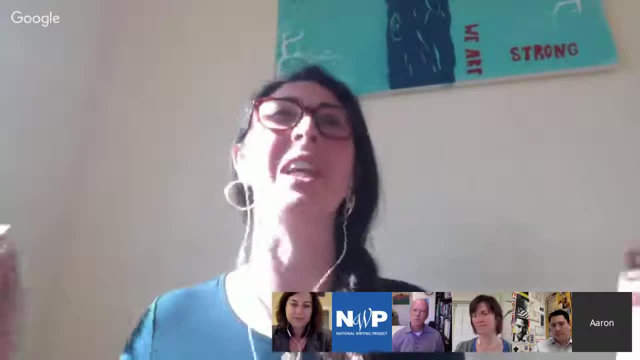 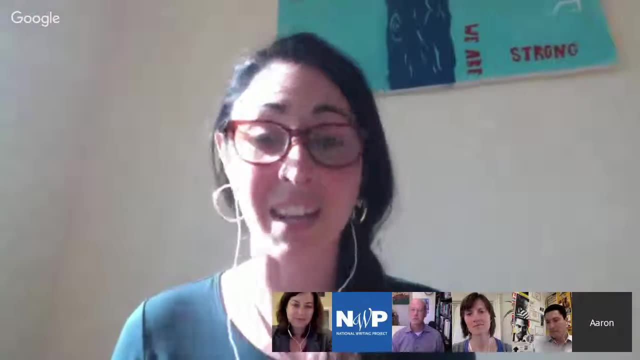 in the classroom and can always grow as a teacher. but the I don't hear from students: why does this matter? That's not, That's not a challenge. They get it. They get why it matters. and when someone asks: why does this matter? 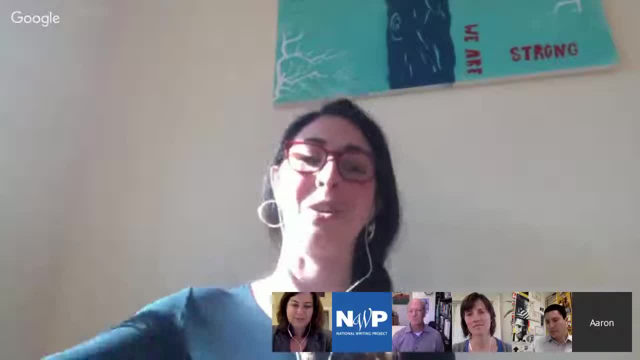 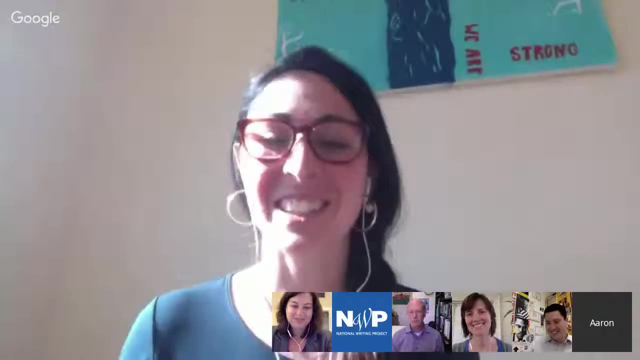 I never have to answer because there's like an, There's this outrage from some of the students in the class that are like: what do you mean? why does this matter? Like this is, I'm gonna, like you know, share with you. 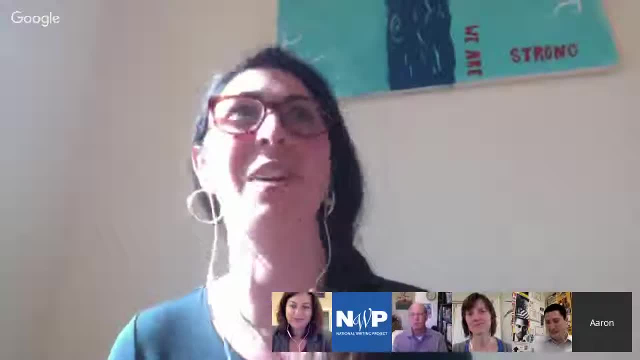 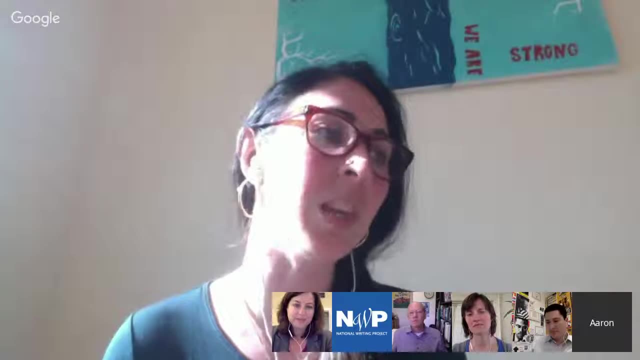 how this affects our family, remind you how this affects your brother that I know, whatever. So they kind of hold each other accountable to the content. The piece about community partnerships, I think, is some of the richest work and the most challenging. 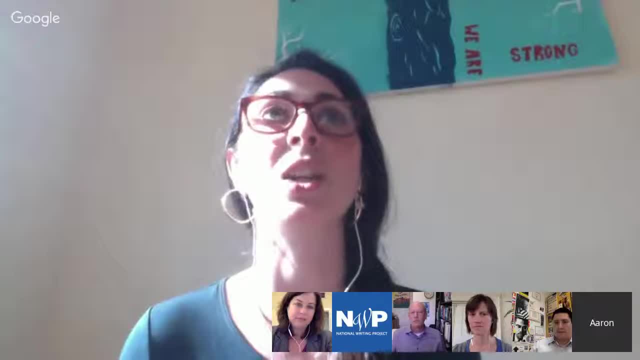 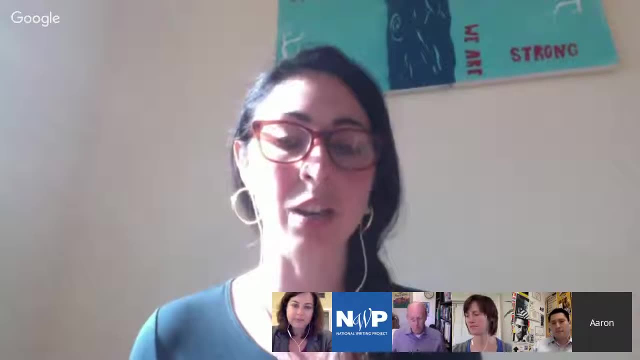 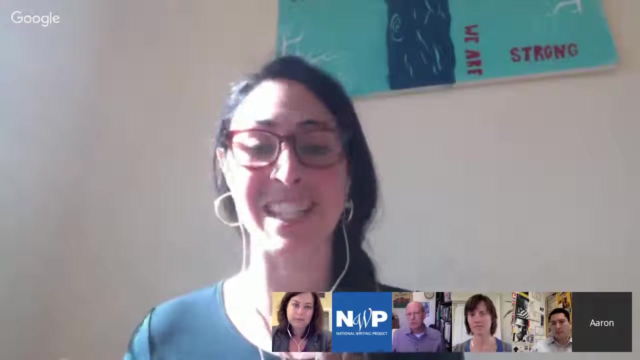 It is. You know, I think, even for many organizations that have a deep interest and belief in youth leadership. as we know, as educators, it is very different to believe in youth leadership on an abstract level and to facilitate it in the concrete. Young people are ever-changing. 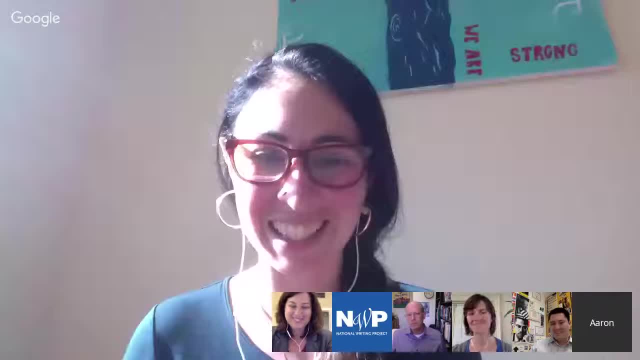 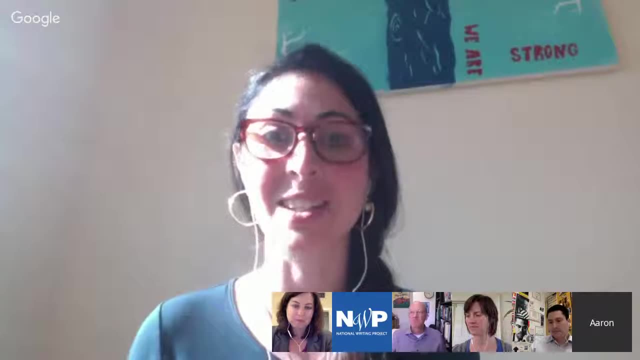 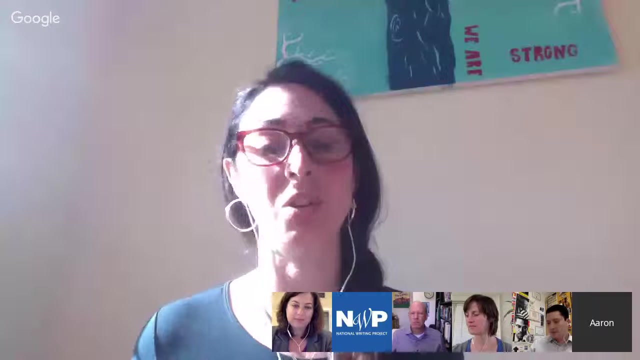 super moody and in many ways way more militant and confrontational than adults, And so organizations need to be ready to really embrace the voice that young people bring if they want to engage in an authentic way, And I think those are the partnerships. 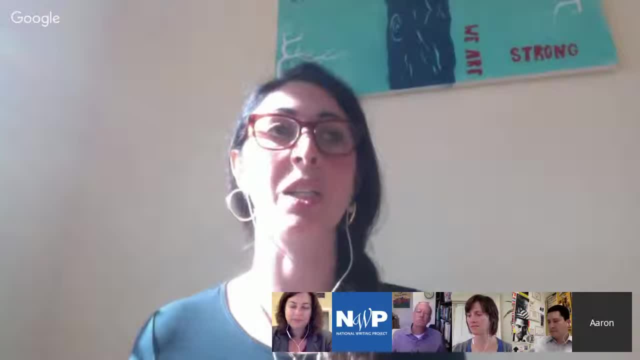 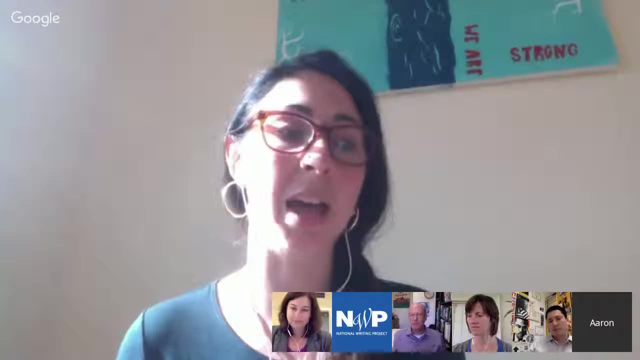 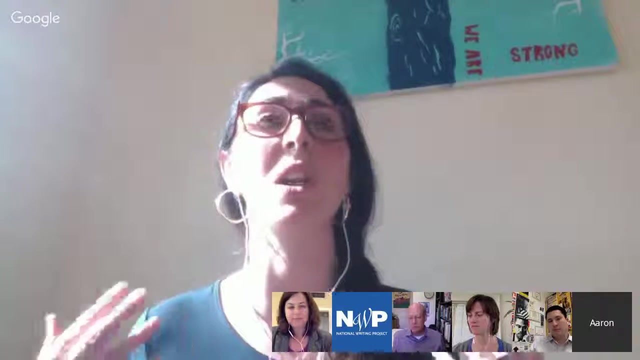 that are strongest and most important to build are with organizations that have a deep care and openness to youth leadership and have a long-term investment in the community. There's like a plethora. I think one of the things that can be overwhelming is, as you were saying. 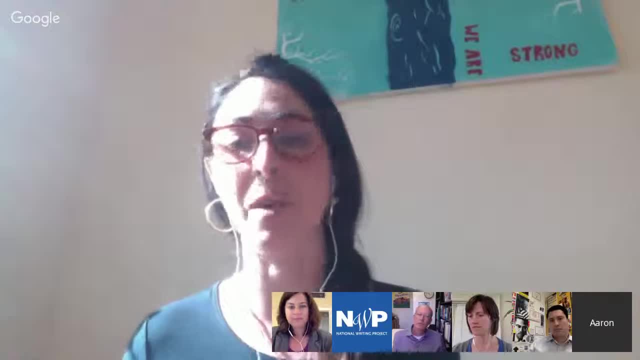 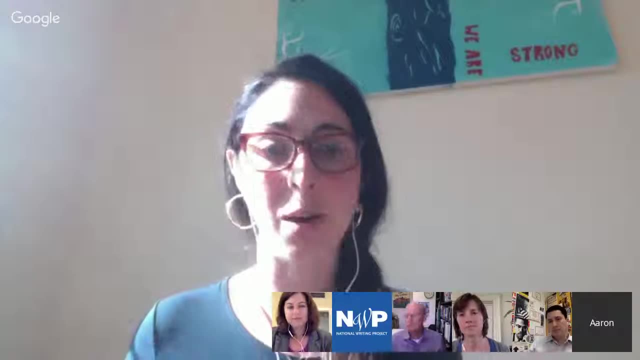 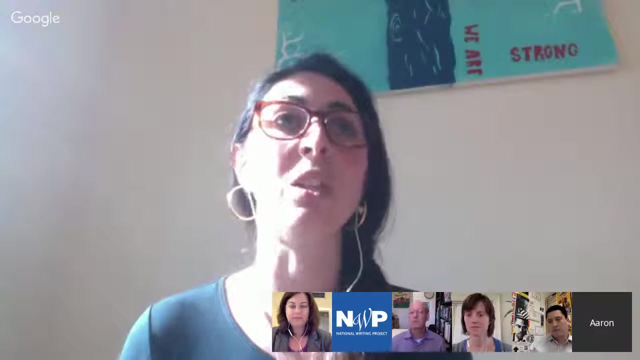 there are so many organizations at this point in time and so much grant money and different groups that are looking for these partnerships with schools, Particularly right now in California. that's a big theme, these industry partnerships, And so really sorting through and figuring out 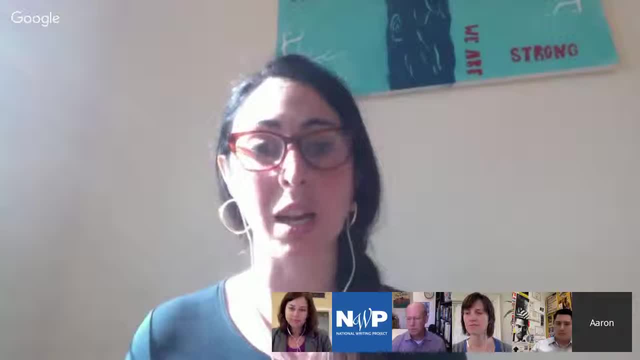 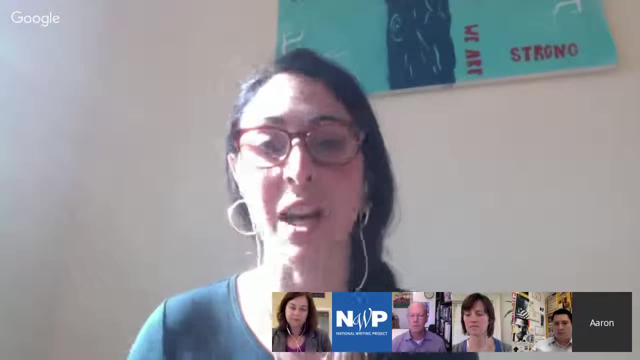 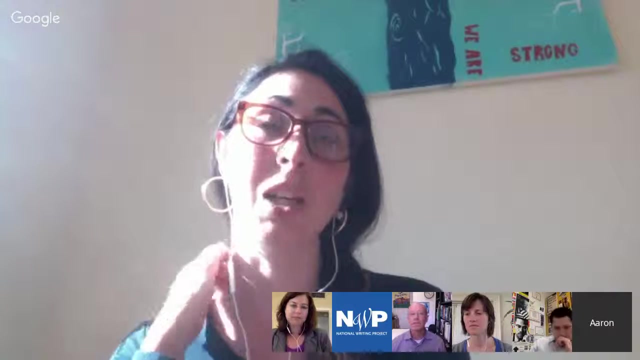 what organizations we can build with that's going to be sustainable in the long term. that's super essential work, because otherwise those partnerships fall off, you know, the next year. The other piece about it, though, and I think what does make the work easier: 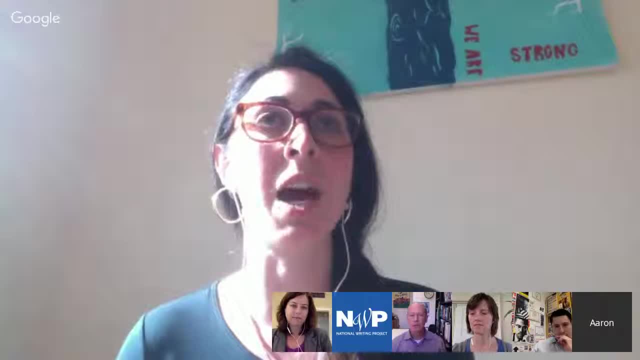 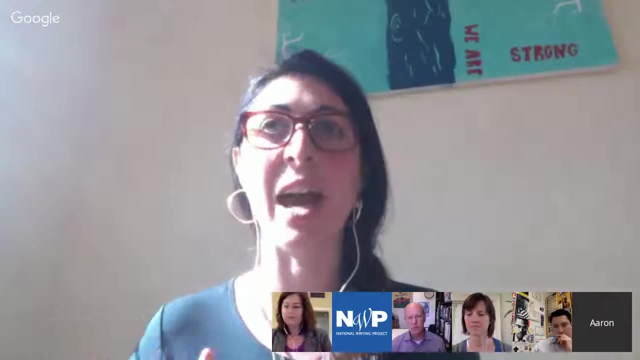 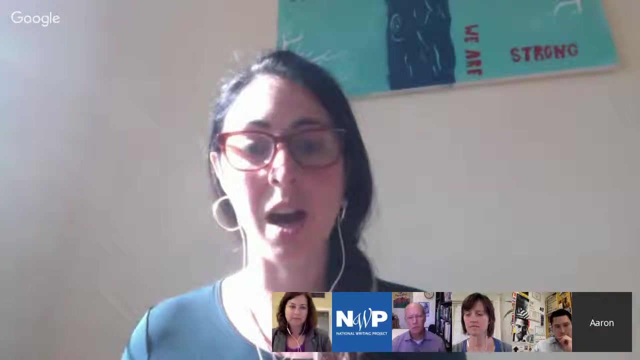 is. I think there's nine adults that work with my students on a weekly basis in some sort of mentorship role, So they have many people that they're having these conversations with because of the organizational partnerships. There are issues that I'm not equipped to deal with. 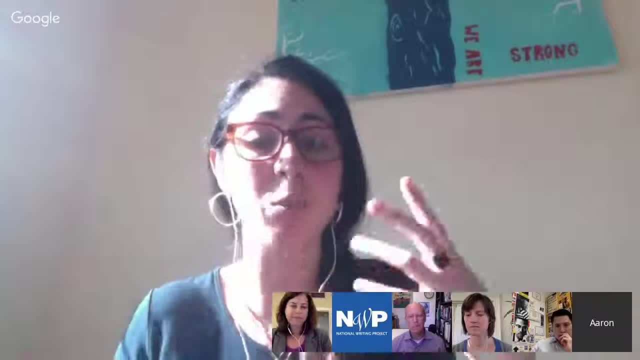 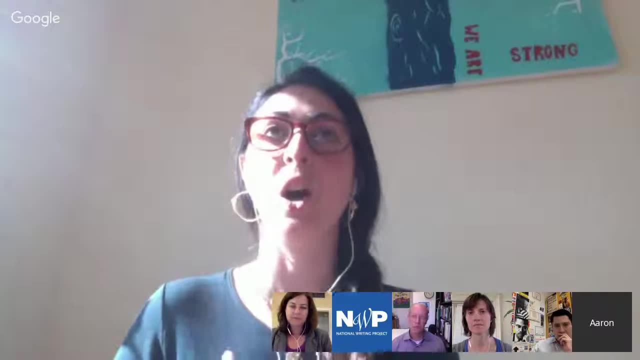 Times that students that I deeply connect with, students that I don't, but there are other people that are holding the work because of the partnerships that we've built, And so there is like an emotional level of labor that is part of civic engagement work. 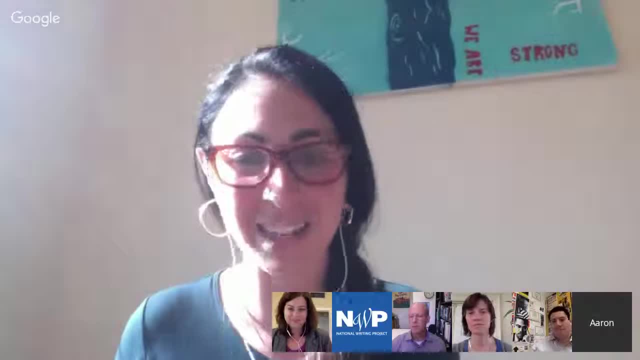 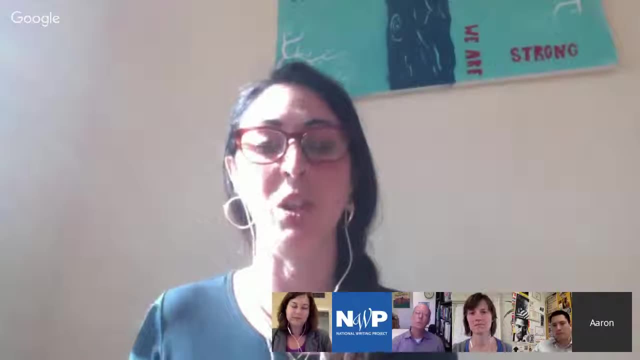 and should be, and if it's not part of the civic engagement work, then it's not being done right. But it doesn't need to be held alone and when we're doing this in a deep way, in a network with other community groups. 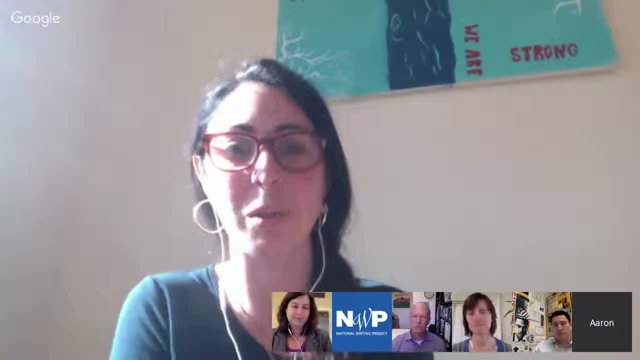 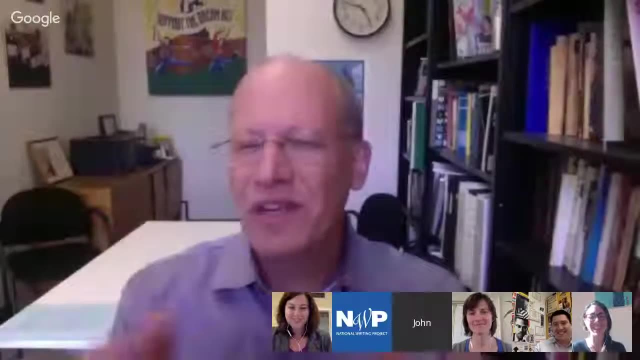 and we're not isolated in our own classroom and there are other people to be really building this vision with. What would you say, John, I was just going to? Oh, Eddie, I just wanted to build on one thing that Perry said. 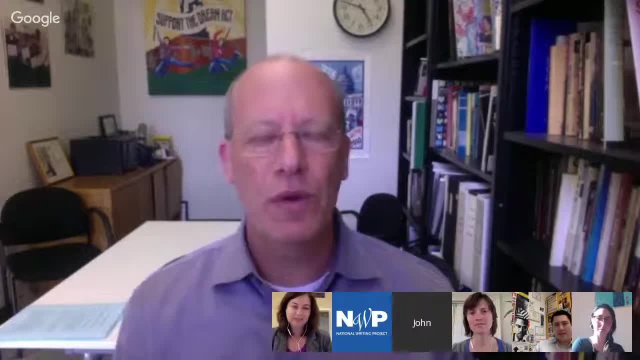 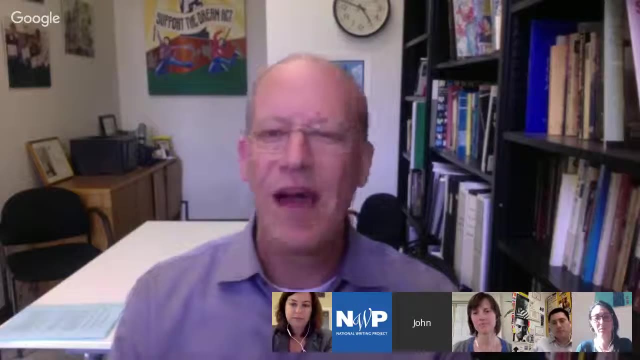 In my experience of working with youth organizing groups and youth development groups, there is this dance of sorts in the sense that if an organization is only focused on young people's learning and not at all focused on any real politics, then it seems inauthentic. 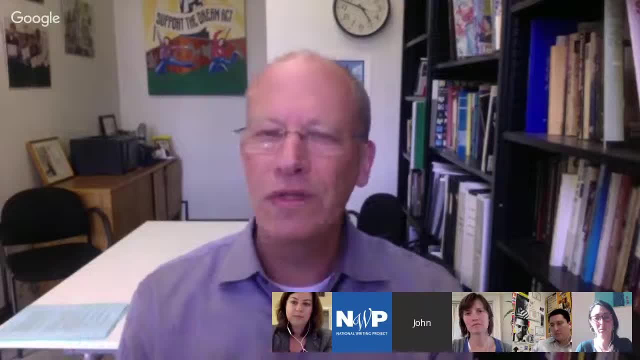 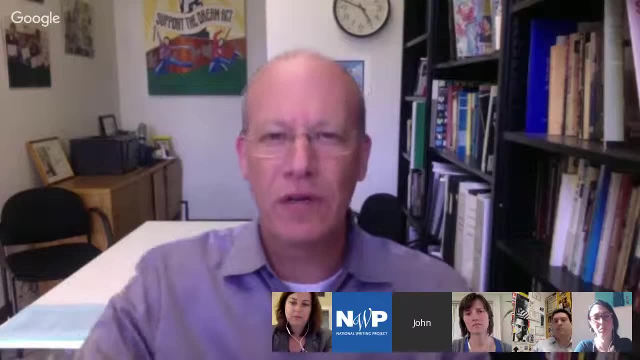 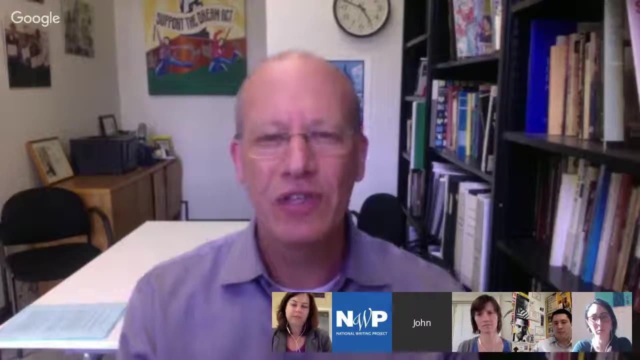 On the other hand, if the organization only looks to young people as, in effect, young people that they can use to win a political game, and doesn't care at all about the young person's development and learning, then that's really problematic, And so the organizations that I think. 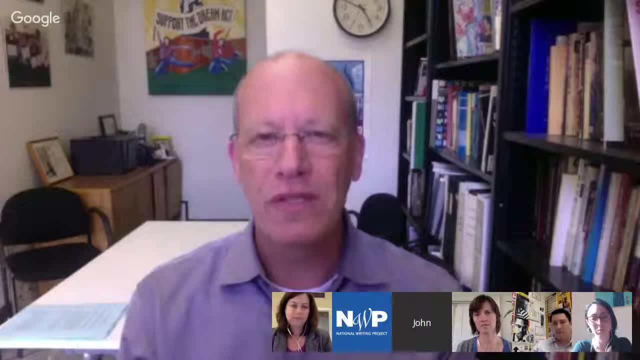 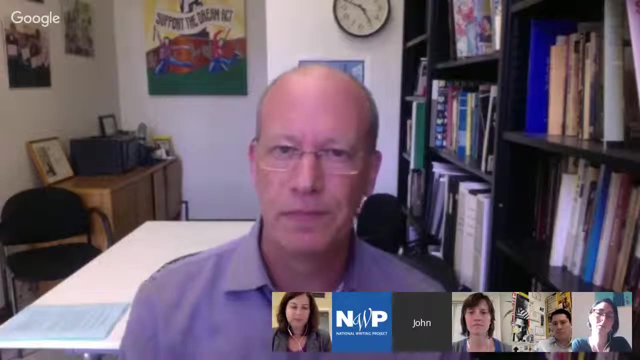 are most vital to partner with are ones that are holding both of those goals simultaneously and thinking about both of them, And I think that educators can really play a powerful role in helping organizations, as partners, think about these two roles simultaneously. I have one more question, but, Eddie. 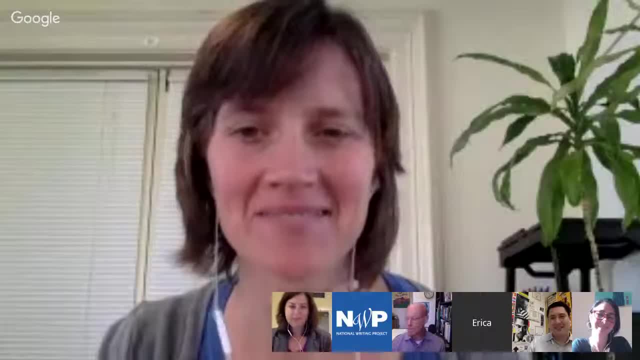 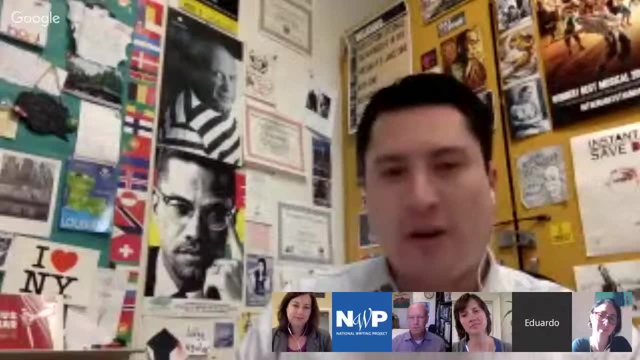 I want to give you a chance to jump in on that. if you wanted to add, Sure, Yeah, because I'm just thinking of the question, right, as far as those teachers that you know, how do I even fit this in my schedule, right? 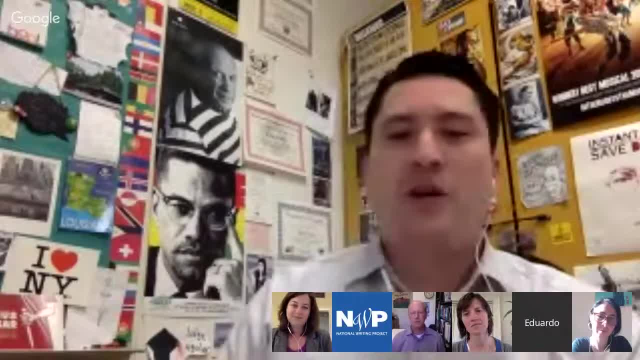 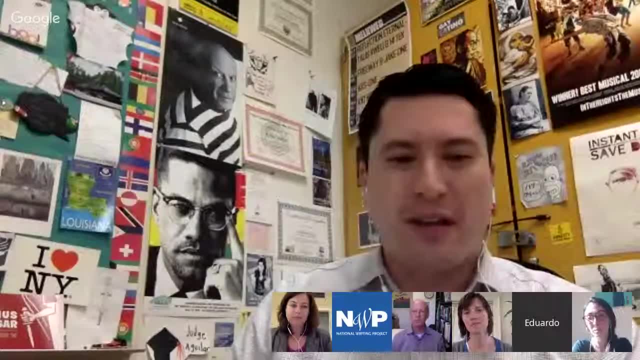 Common core standards, standardized testing. where can I possibly right if they're stuck on a pacing plan? right, at what point would I be able to do anything like this right? So when thinking about like schools, I think of that group of teachers. 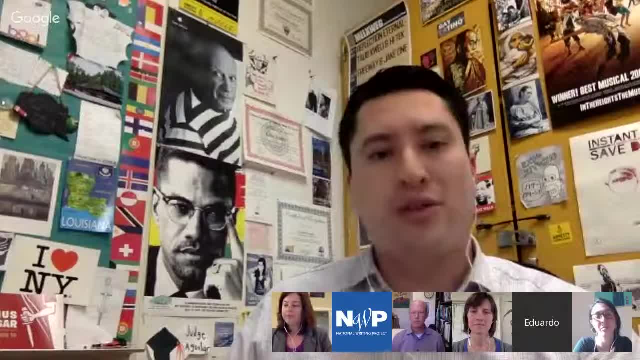 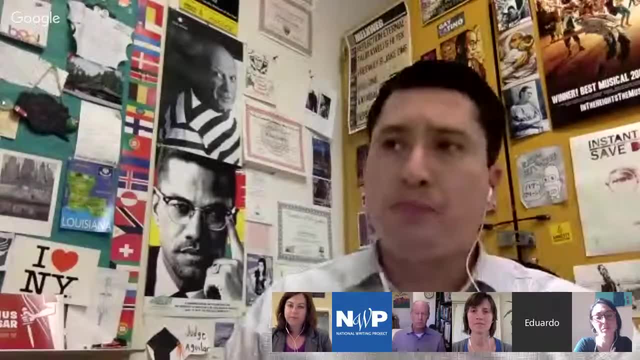 and then those teachers that want to do this. but where do I turn to to get that support to be able to, you know, kind of roll this out, right? So for those individuals, right, that are just more concerned, going back to what John was saying, 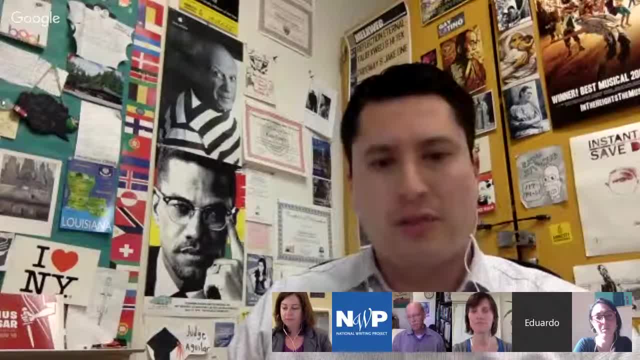 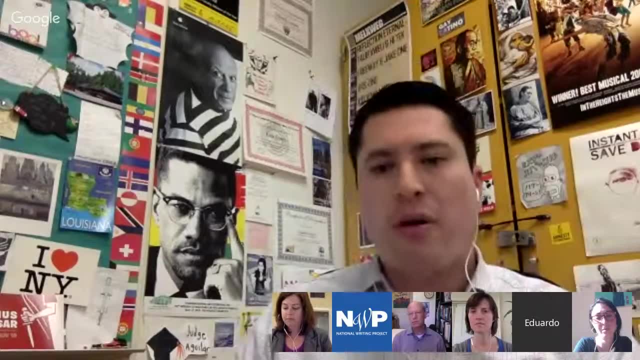 you know it doesn't have to be one or the other right just like he was mentioning. I think you know what I've done early on, after having been trained in YPAR practices, I would for all my 11th grade students. 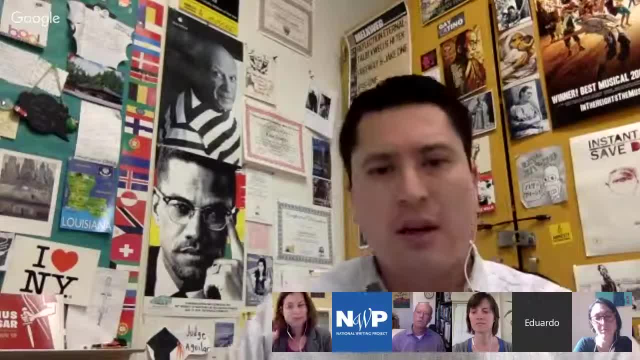 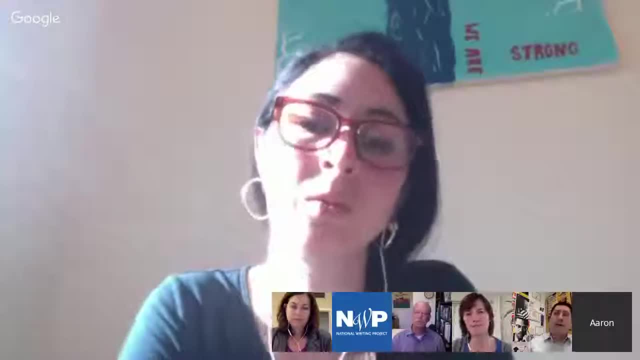 so I have like about 120 students right in a year at the end of the state testing, which usually was, you know, early May or so I believe it was for a solid month- then I would do YPAR right with all my 11th graders. 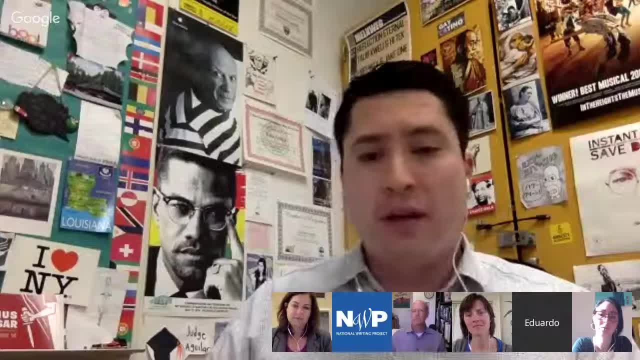 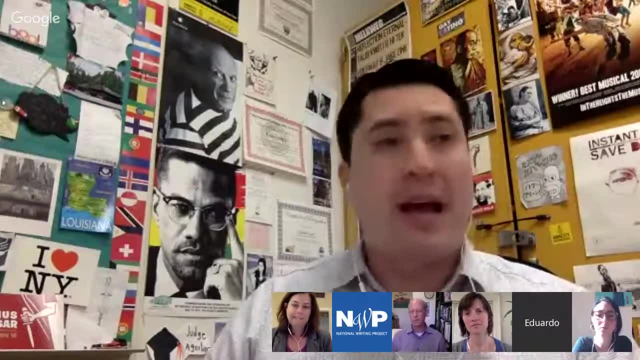 And at my school and in the state of California high school students are supposed to meet a service learning requirement and at my high school that would happen in every US history class in 11th grade. So it just kind of fell together in that, you know. 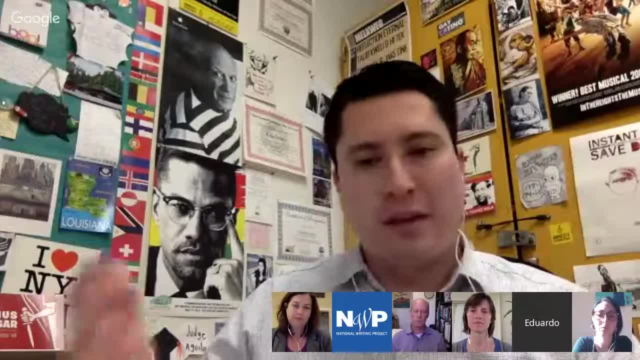 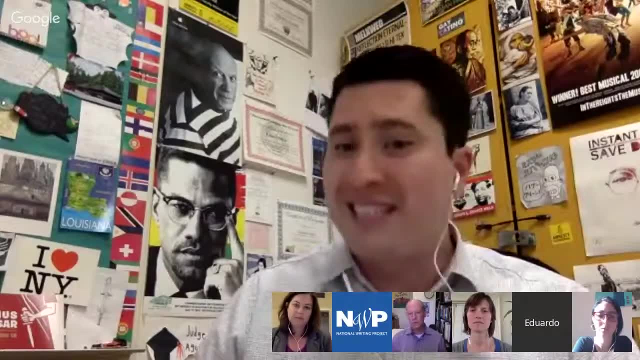 I was able to address, you know, all of that in one project and at least it gave them a taste. And so what Nicole was referring to in the beginning of a five-week intensive, every day at UCLA doing this work, I would try to do that within a month's span, right? 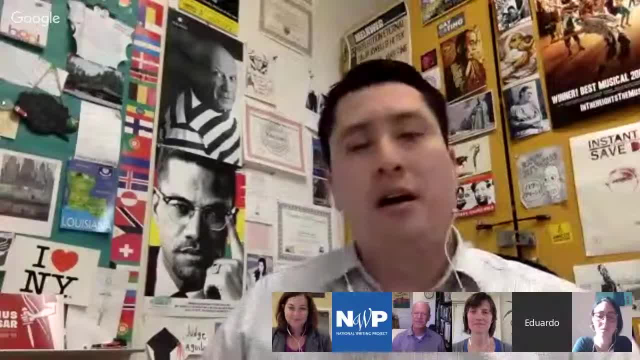 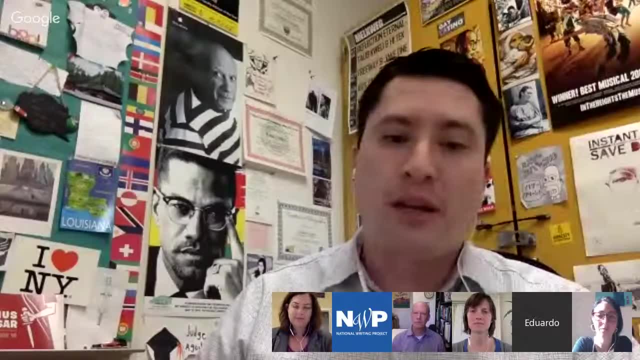 every day in the classroom. But luckily, because I had, I was in the Humanitas team doing interdisciplinary work with an English teacher, which is very helpful if folks are working in that type of system. But my colleague, my English teacher, they were getting double the amount of time. 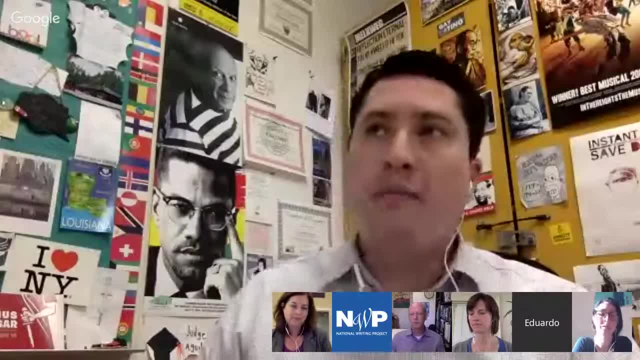 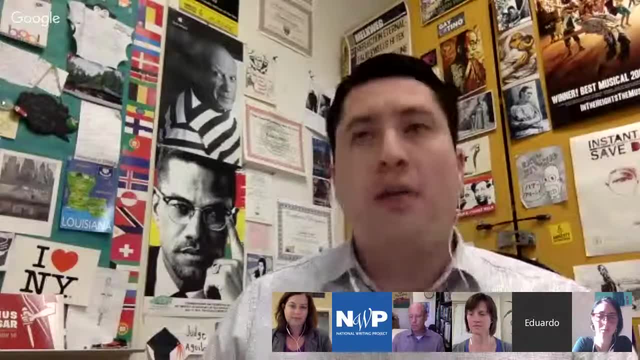 in the school day to do this work. So, while in my classroom we were developing, you know their research topic, and it ranged from community issues to school issues, and so we would break up groups into fours and then, as they were doing that, 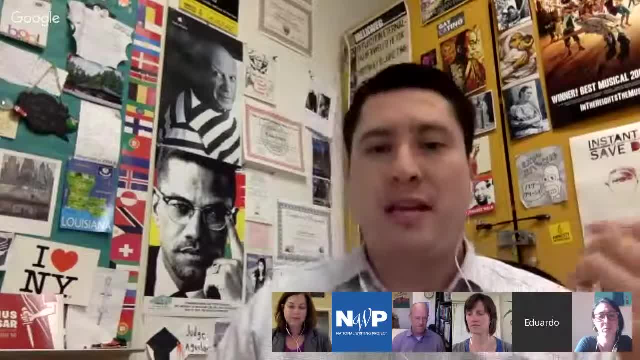 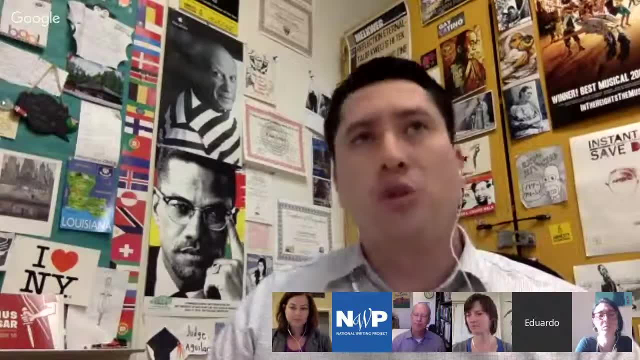 and as eventually as they were creating their survey statements and interview questions in their English class, they were getting a lot of the theory right. They were getting, you know, they were getting Yoso. they were getting Noguera Andrade. 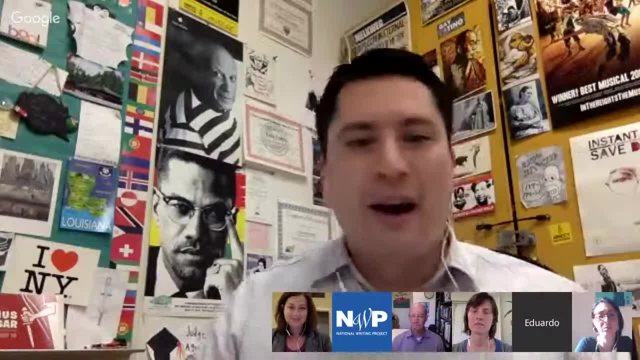 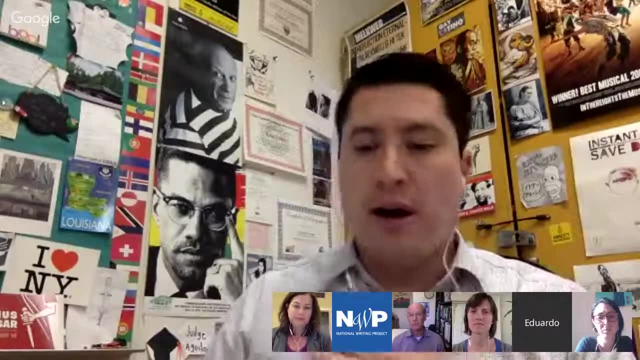 you know, and the list goes on and on right, And so it was a happy marriage in that we were getting that or I was getting that support. So that allowed my students to really feel you know being civically engaged because you know the whole year. 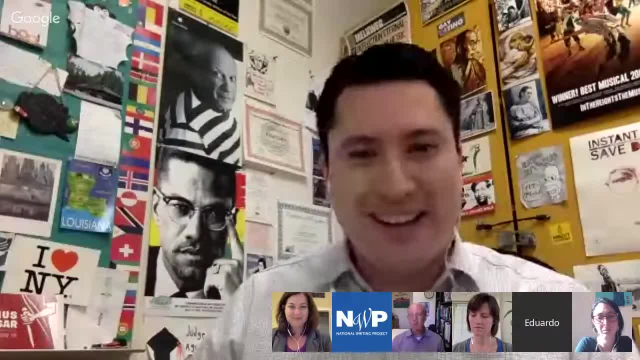 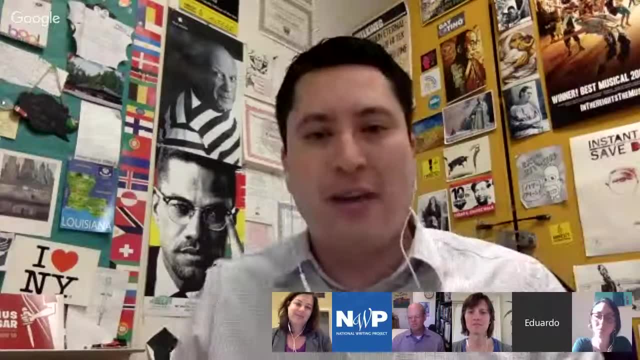 I think that I anger my students a lot, right with what we cover, and so I don't want them feeling, you know, empowered. but then what do I do with this? How can I even move forward? How can I propose policy? 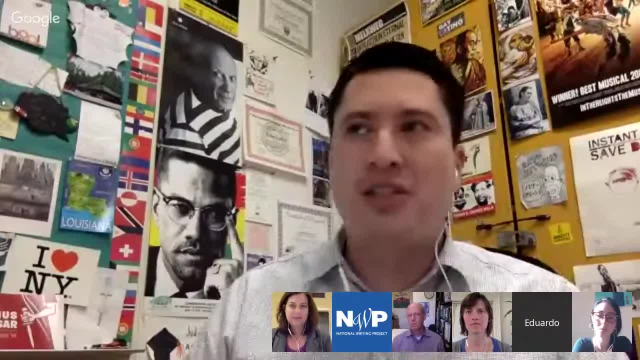 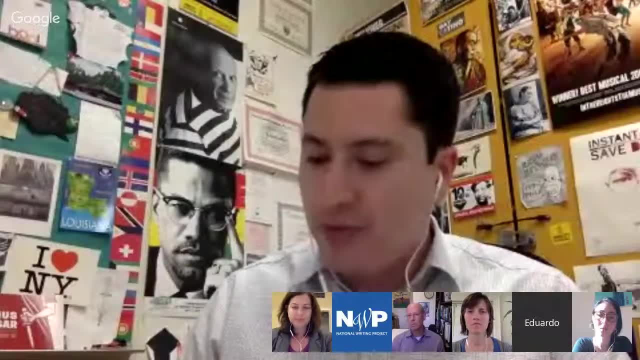 or how can I give people marching orders that this is not just on us, but you have a role in this, and I'm going to tell you exactly what that is right, And so that's how I was able to use that time. 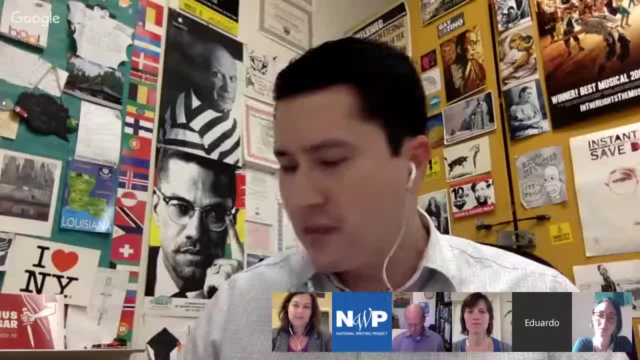 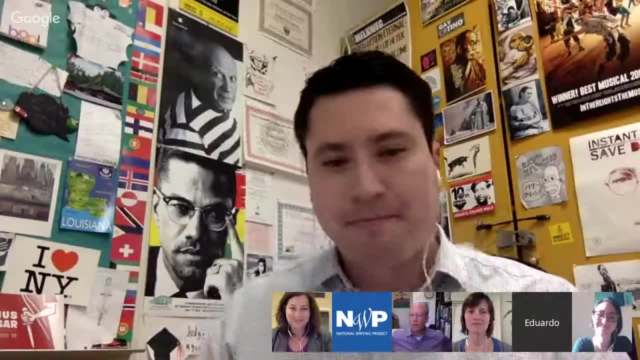 but now it's a little different because of the way the format of my school has changed a bit, so I'm able to do you know YPAR earlier on in the year. That's great. Thank you all. So I just have one last question. 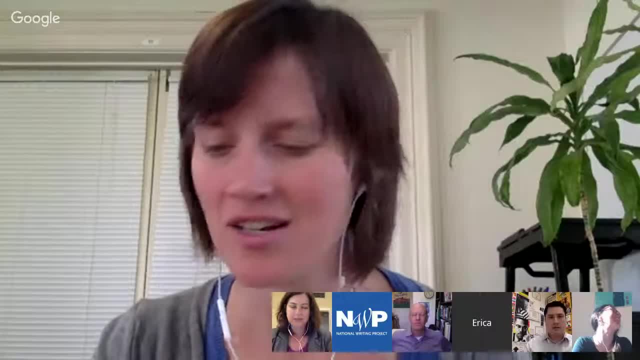 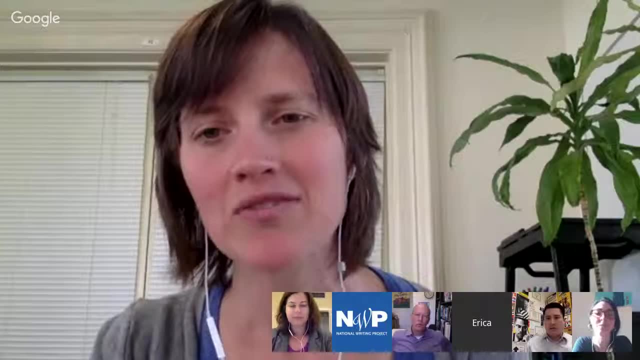 and we only have a few more minutes so maybe people can sort of share brief final thoughts and the question that I'm thinking and you all have touched on this, but would love to just kind of highlight the unique opportunity that we have to talk about doing this work in schools. 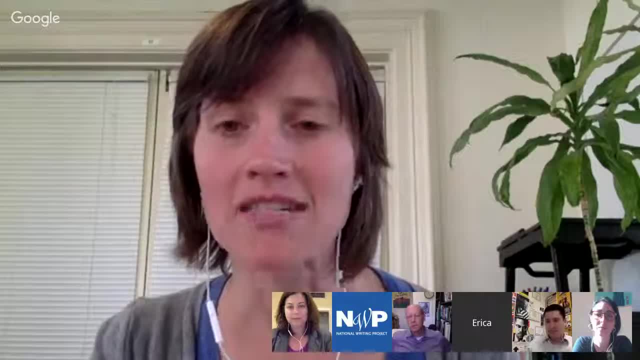 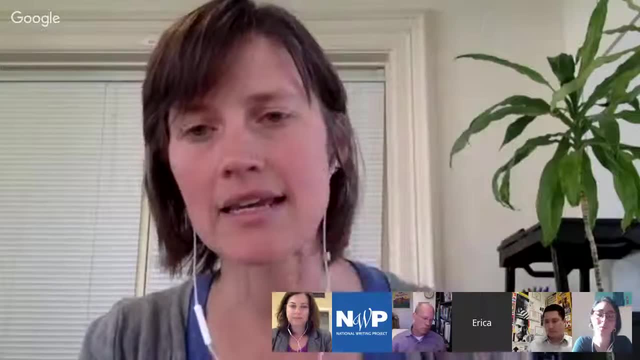 because I think you know, civic engagement work often happens in many settings and sometimes you know it's after school or in more informal learning settings. and I think you know, Eddie and Perry, you both are you know. 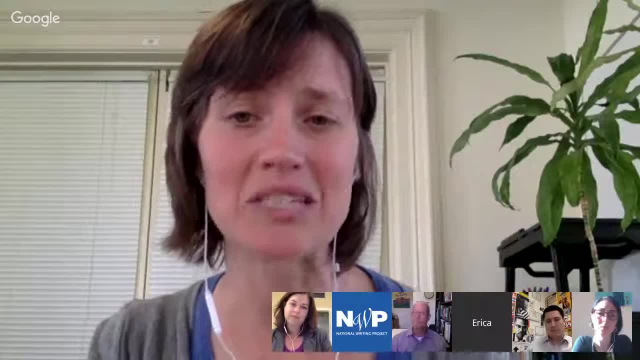 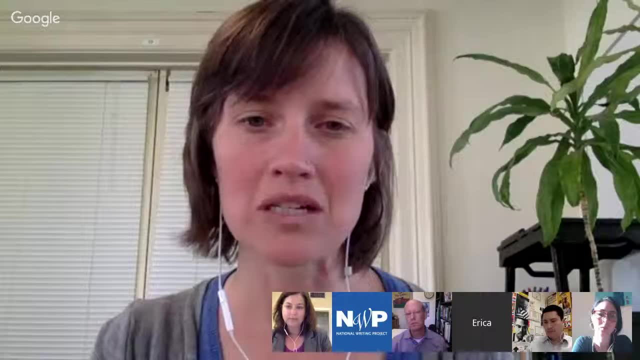 doing the hard work of integrating this into a school district and into the school day. and I think, you know, I think one of the things that we, especially in the work that we've been doing in Oakland with Perry and other amazing teachers, is really, you know, 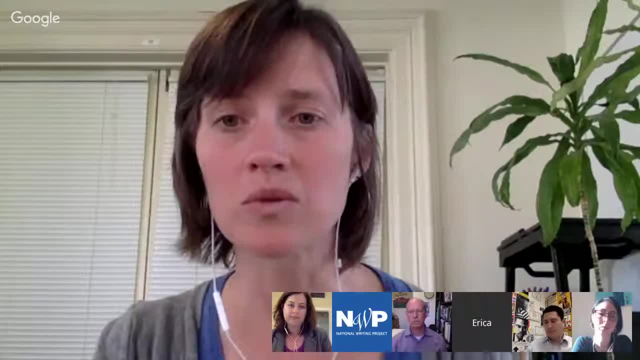 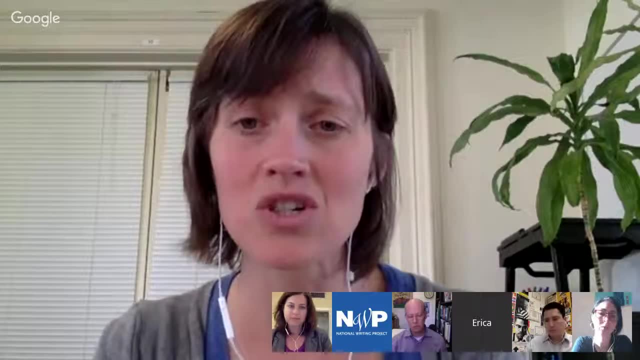 making the effort to really work with the district because we really believe that schools are powerful places to access youth and to really ensure that this sort of civic engagement, youth work is equitable, that we're not just reaching the students who are able to. you know, 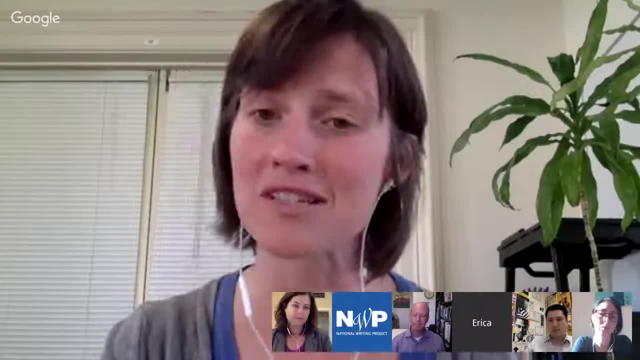 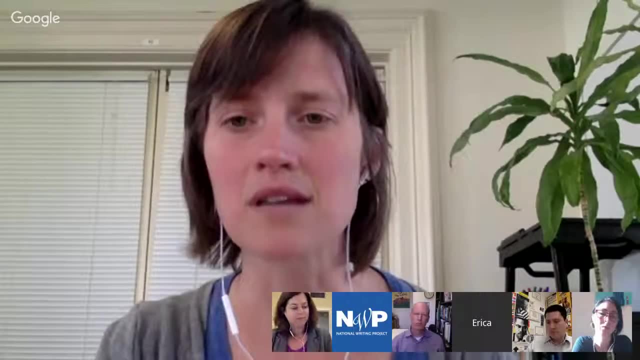 show up after school or who are volunteering or who are part of this club. but really, you know, how do we really think about serving all young people to really develop their civic and political selves and to really have the tools, I think, especially in the digital age? 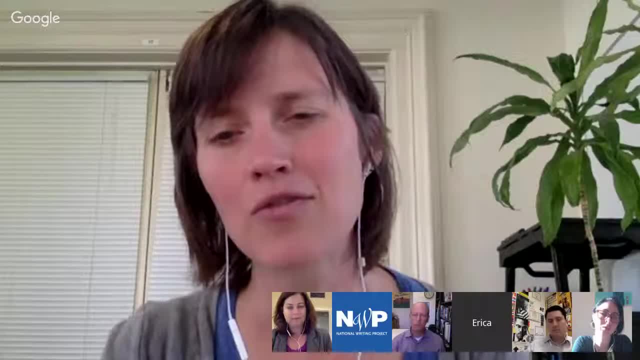 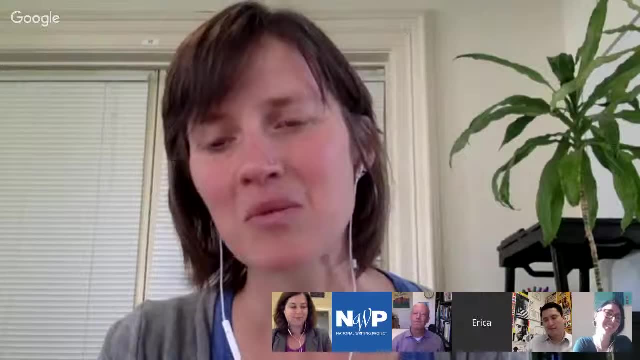 to get their voices out there and make change and so I wonder if folks want to share as final thoughts. but you can tack on other things if you don't want to attempt to this question, but I just think it would be wonderful to hear. 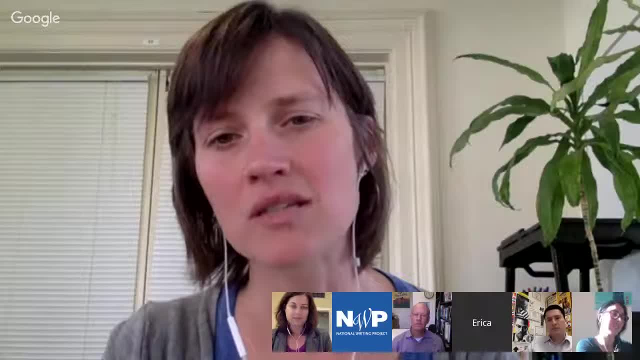 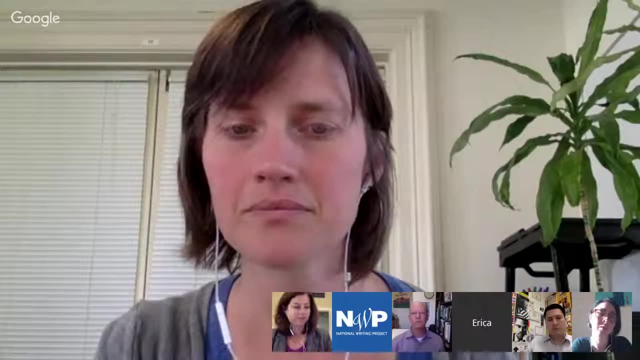 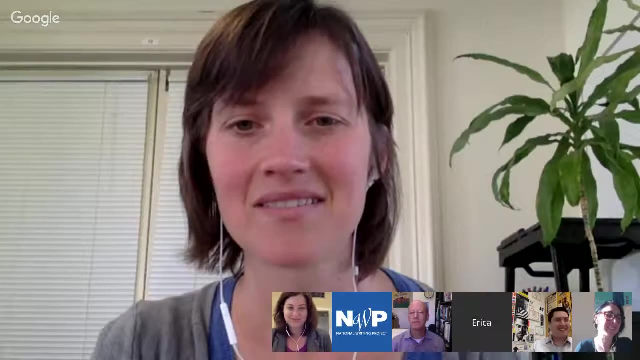 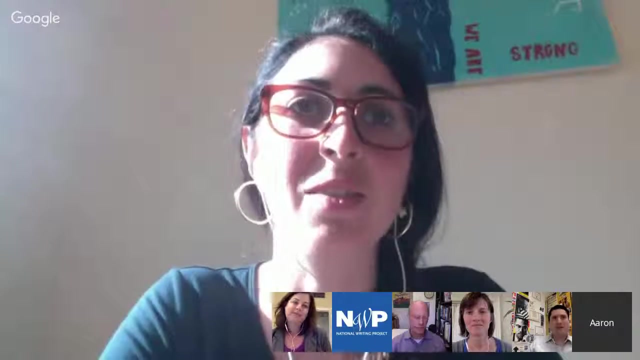 you know, what advice or strategies do you have for doing this work in schools and really making sure it's equitable and reaching all youth? Anyone can jump in, so I guess I think this is starting to be touched on. I feel like the first thing. 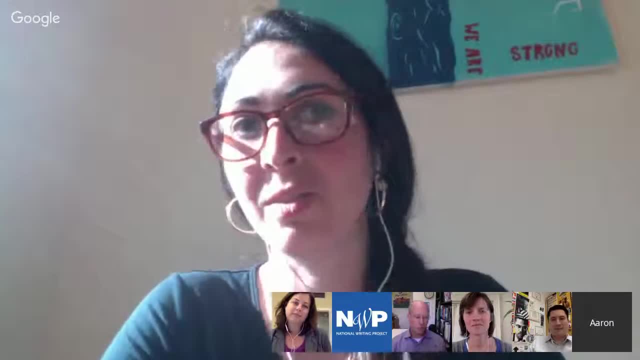 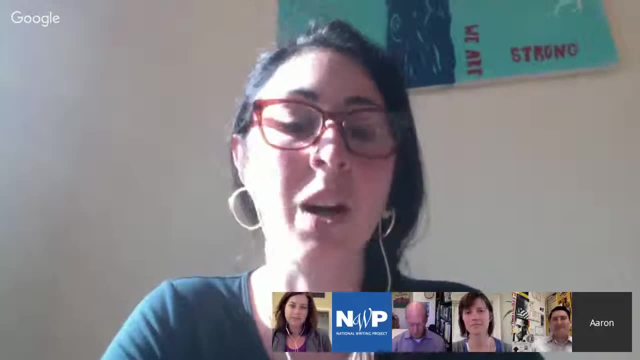 that we, you know, need to do is fight for this type of work to be structured into the curriculum: civic engagement work, ethnic studies, frameworks, that we need to rethink how we teach. We can't just add in civic engagement into the enormity. 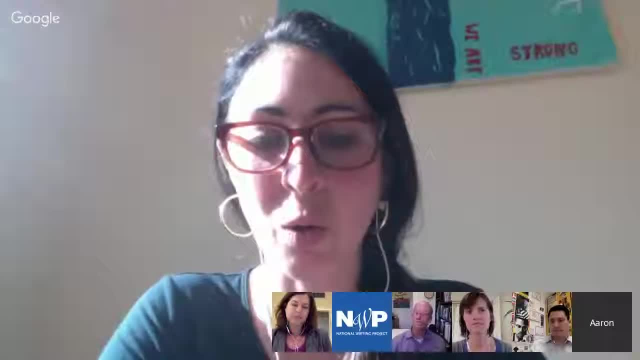 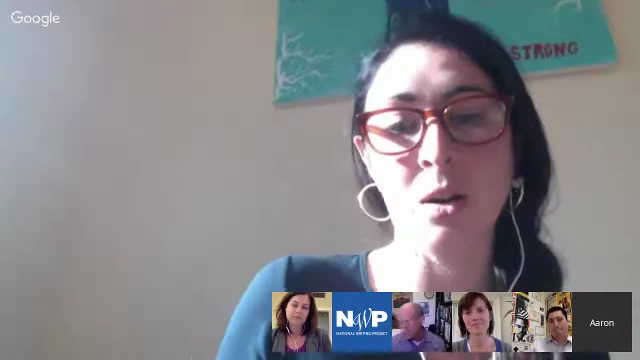 of the standards that we have right now, and so there, I think, does have to be more of a kind of transformative process on a district level and in a school where there is a deep dedication to it and where you know there is a need. 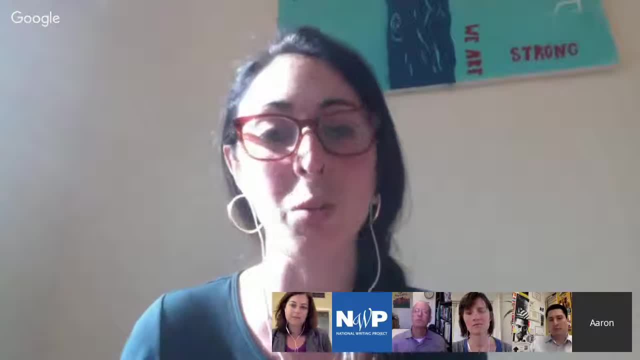 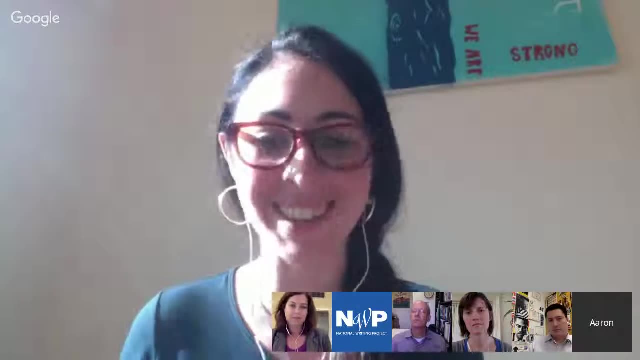 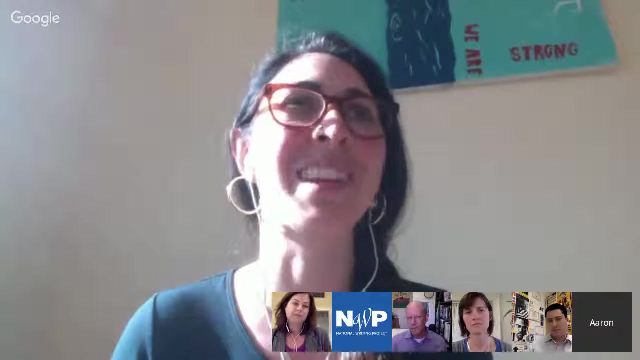 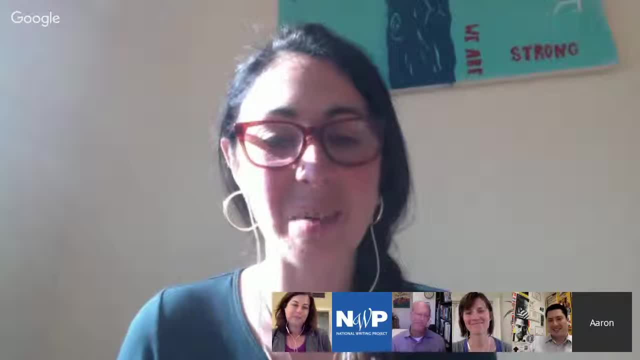 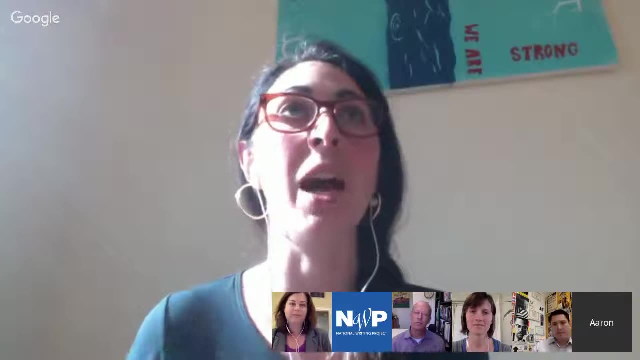 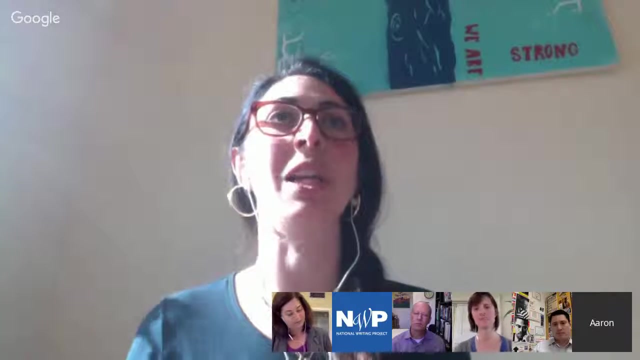 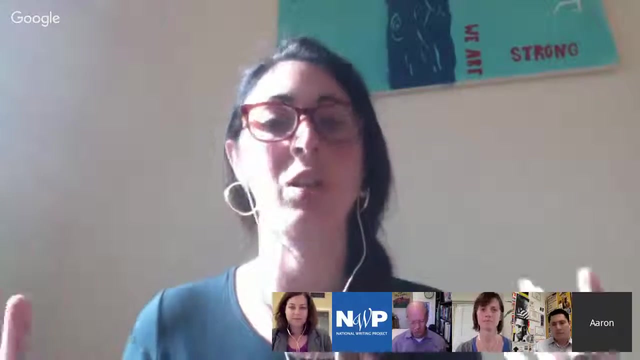 That being said, more concretely and immediately, I think like some of the pieces that have really helped bring this work into other parts of our school are the ways that we've created events and peer education projects that tie in other teachers and spread and engage other teachers. 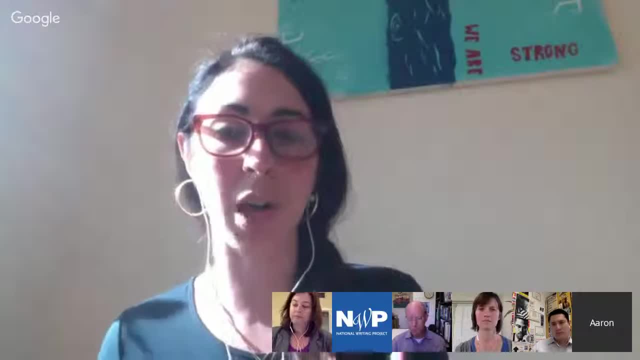 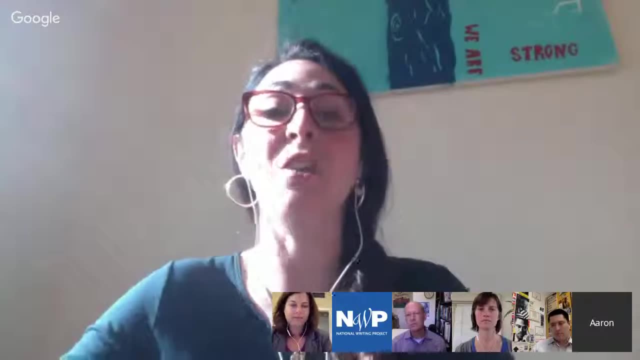 So, for I have students who developed workshops, peer education workshops that they then went into other classrooms to do, and so then they were participating and other teachers were able to see: oh, this is what this work looks like. right, they're seeing my students take. 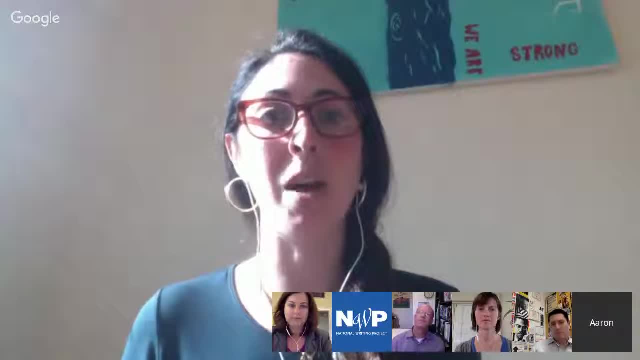 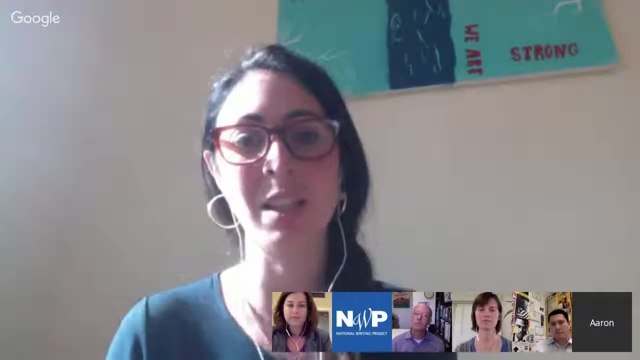 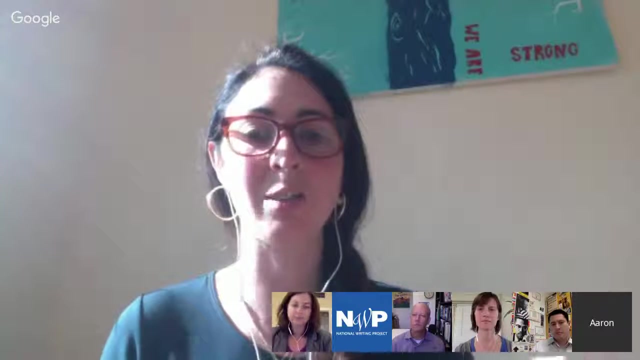 on this leadership. they're seeing what they're capable of and what kind of civic engagement it might mean. and from there I'm getting interest: and how do we incorporate this more? So I think there's also this slow process of like how, within a school itself, do we engage? 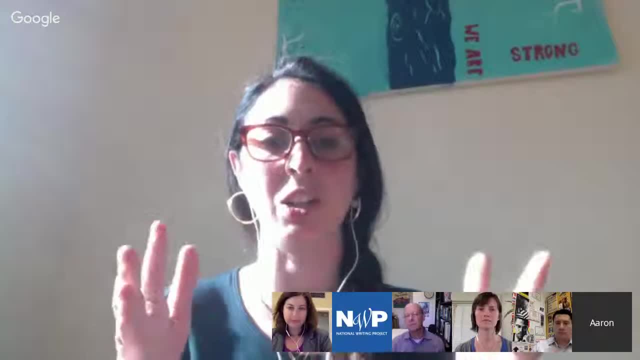 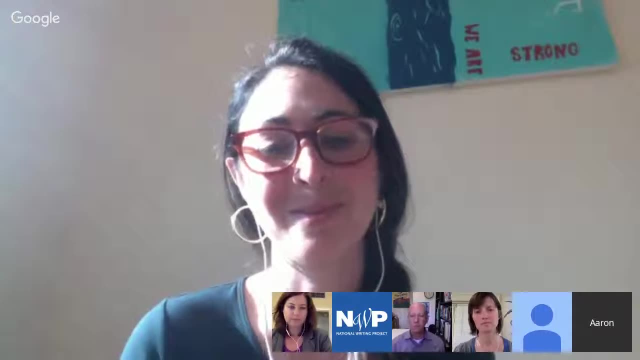 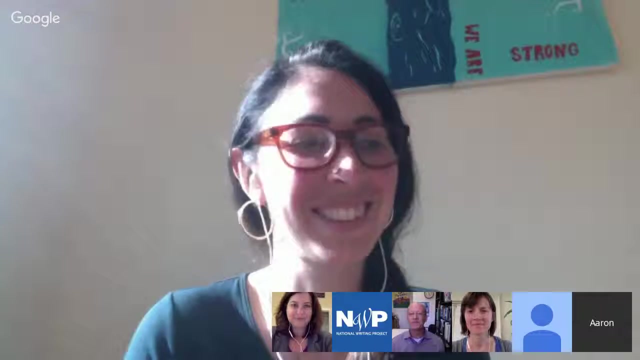 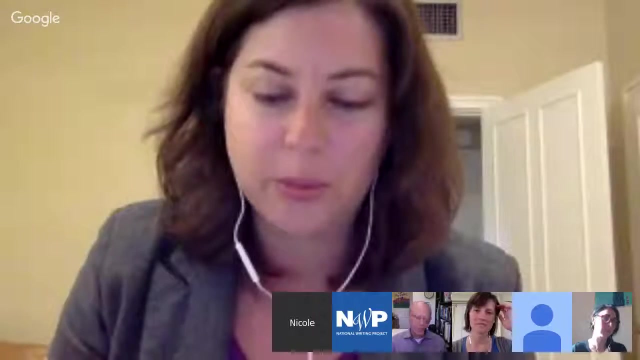 with our colleagues and support our colleagues to plug in, so that these projects don't live isolated in one classroom or one school. Eddie, as you're speaking about your experience doing this in the classroom, I'm really curious about- and I know that you were. we have this symbiotic relationship between classroom practice. 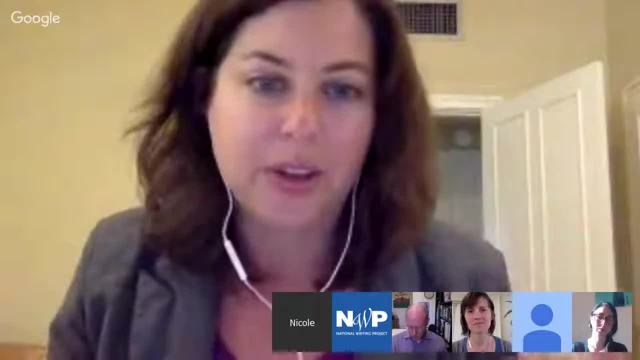 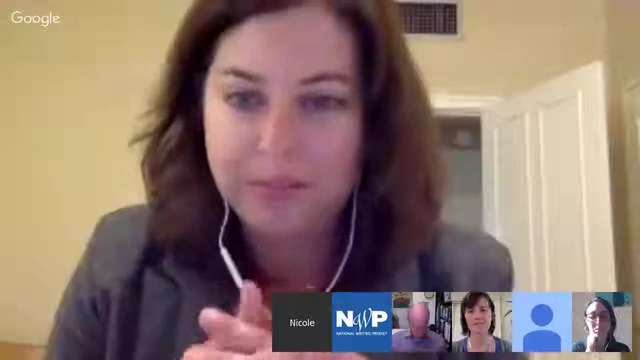 and out of school spaces with the council and how you think in school and out of school time could actually work together and maybe hit different competencies but be a kind of symbiotic relationship. So I'm wondering kind of how you thought about that with YPAR coming into the classroom. 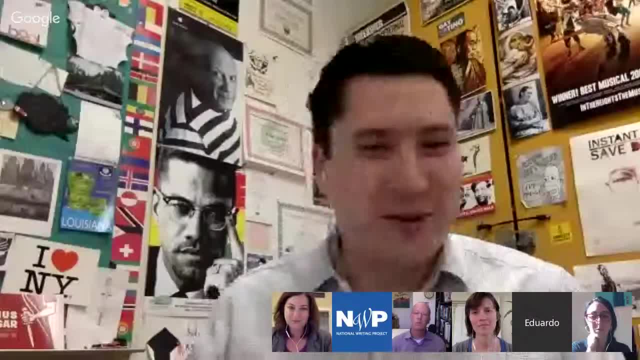 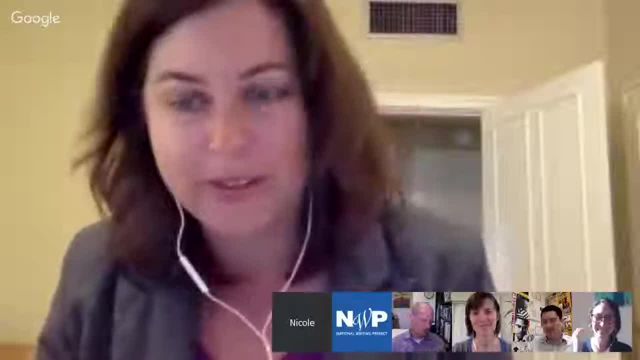 Yeah, All right, hold on. I just it just froze on me. was that question towards me, Nicole? Yes, it was. I was just about like the out of school space of the council and then bringing it into the classroom and doing classroom civic engagement with more constraints. 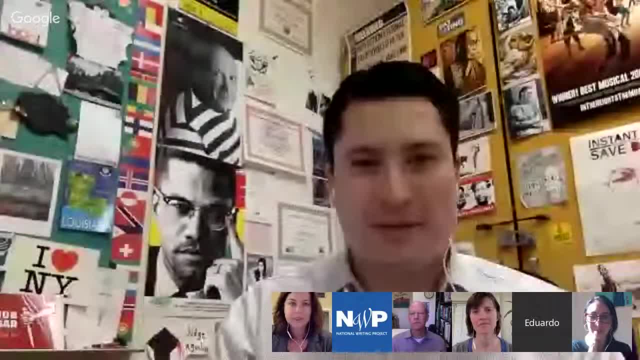 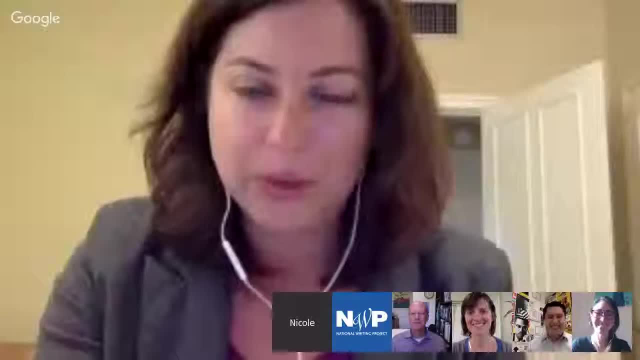 Okay, Nicole. Yeah, did you hear me? Sorry? no, no, I just kind of froze so I didn't hear the question at all. No, no problem, We're just as we're doing our final thoughts. we're thinking about this kind of classroom. 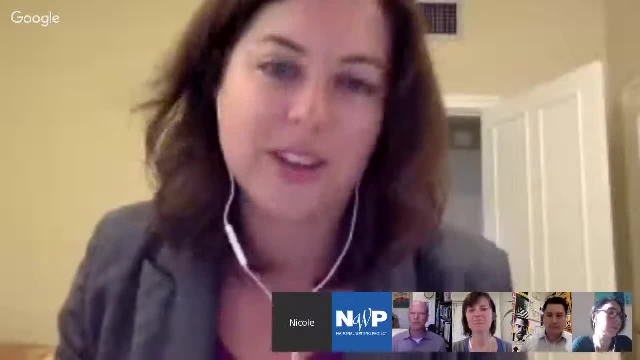 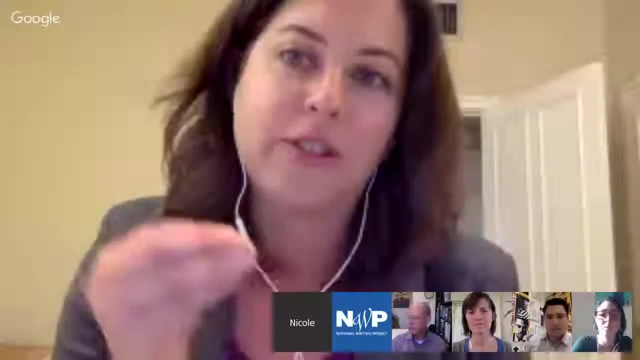 time, Gotcha And out of school civic learning spaces like the council is one thing, but then it's. you know you're dealing with different constraints in the classroom and how you feel why you feel it's important to not just do it outside of the classroom, why it needs to be in the 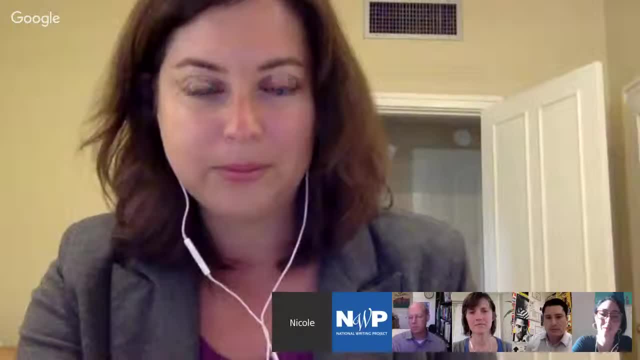 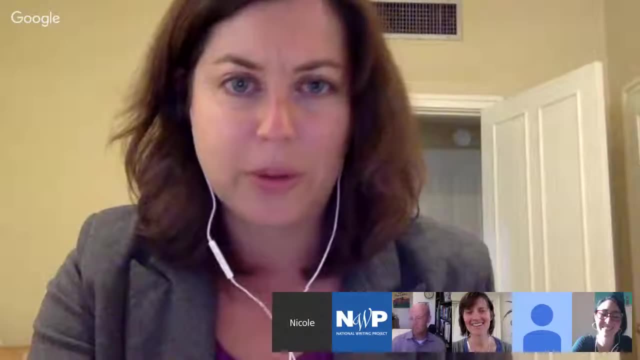 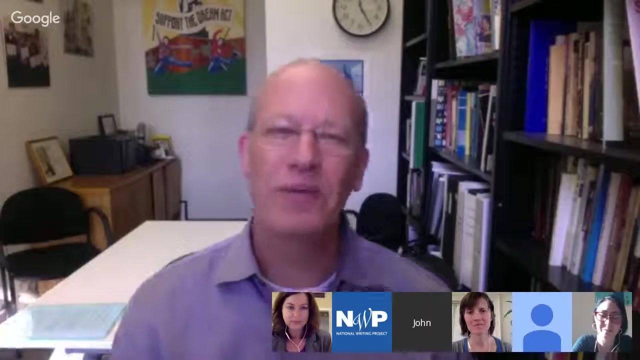 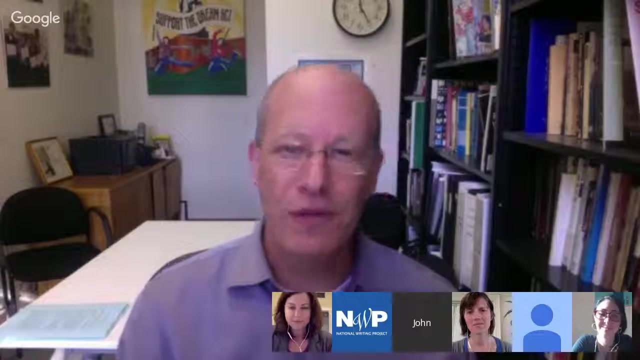 school day, I think Eddie froze. John, do you want to jump in while Eddie's coming back? just about kind of what you hear from this conversation. Sure, Let me pick up on one thing that Perry was saying. Okay, Yeah, I was suggesting that in order to advance and expand the work of civic education in 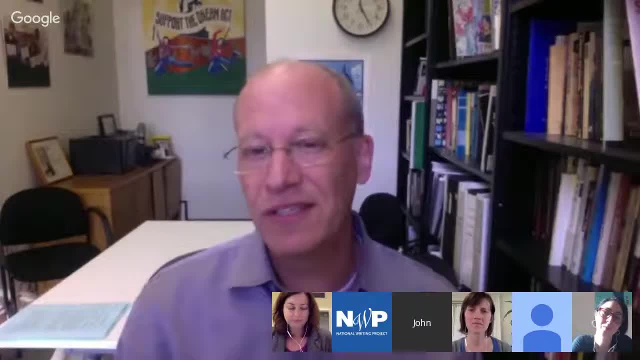 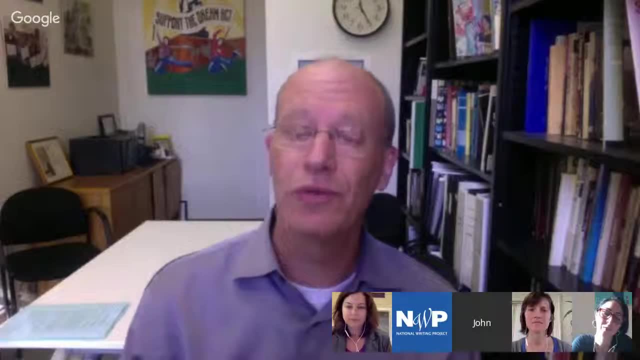 schools. teachers need to push on the system, whether it be at the district level or at the state level or the federal level, to ensure that the conditions are in place in their schools: time, other supports that allow for civic education to occur. 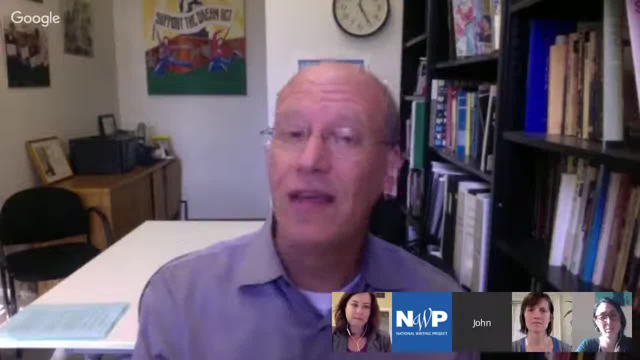 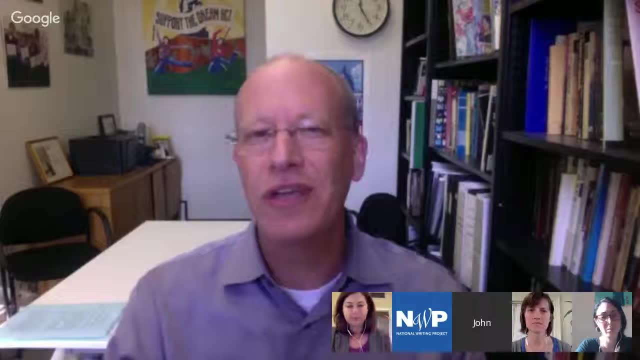 And I would suggest that that's exactly right and that in the process of engaging in the civic process of transforming public education, teachers develop a set of skills around civics. They develop practice in the civic domain. that is really important for them as they then go back and work with young people around civics. 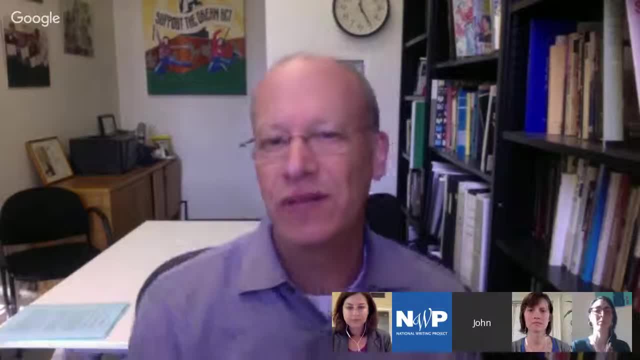 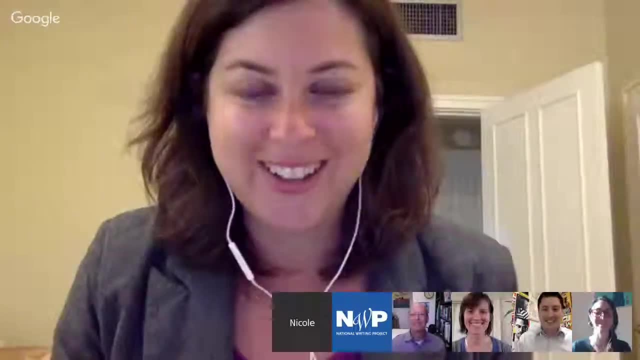 The teachers that are practiced in civics are better at teaching civics. Looks like Eddie was jumping in and out. Are you back with us, Eddie? Yes, Yes, I am. I hope it's working now. Cool, All right. 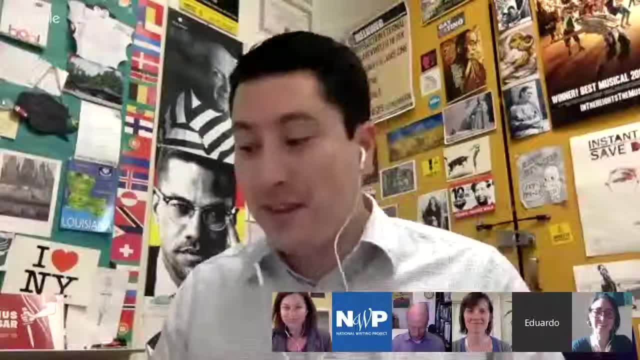 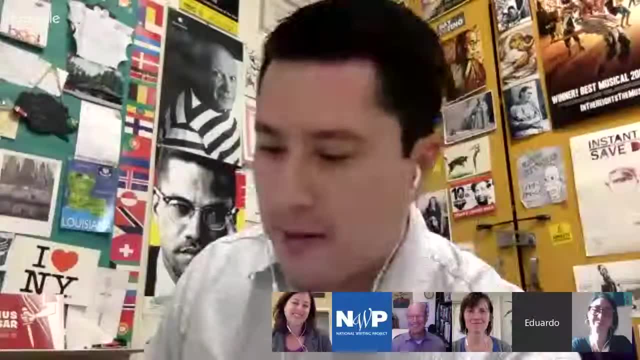 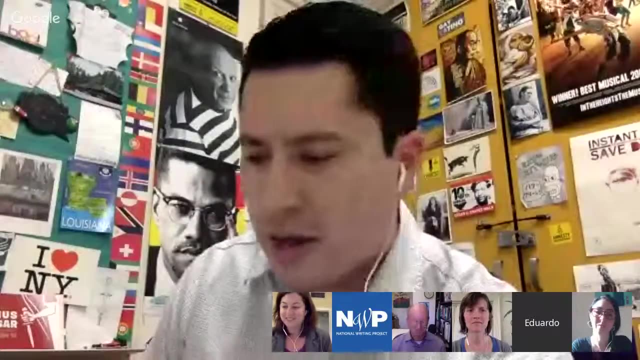 So just last thoughts about civic education in the classroom. Yeah, With what Perry was saying before it froze me out, I completely agree. I think it needs to start with, you know, it can't just be an end of the year project doing this type of you know, trying to civically engage our students. 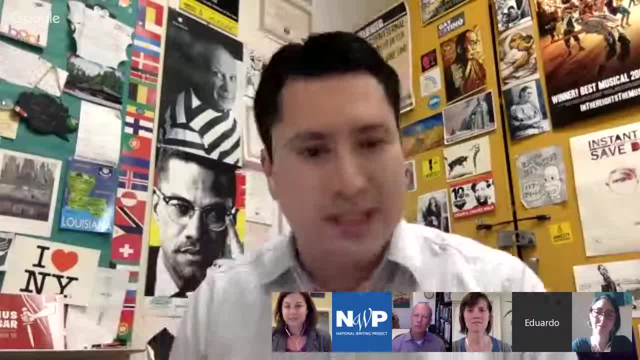 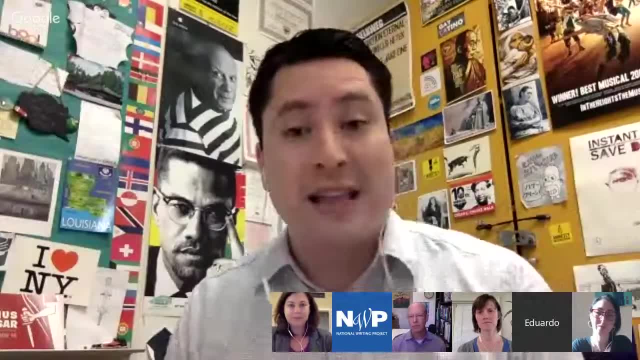 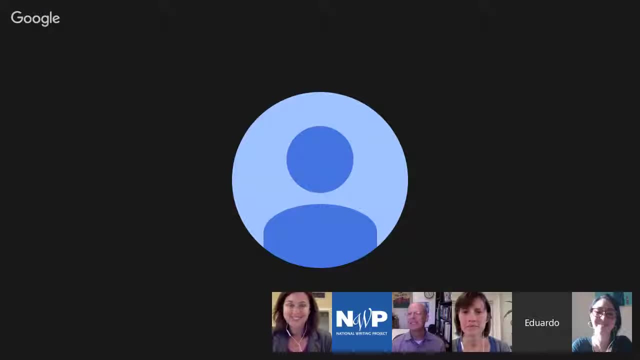 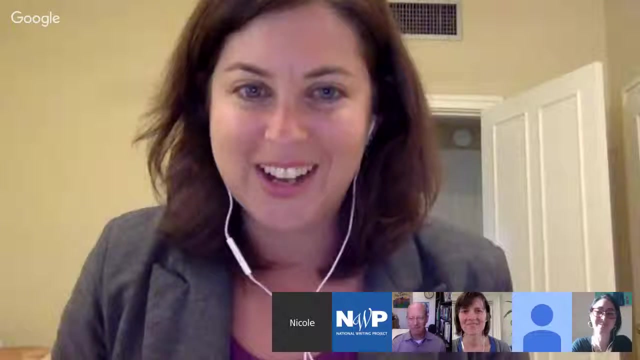 There has to be a huge paradigm shift and transformative way in which we teach. I think we definitely need culturally relevant curriculum. I think by doing that we provide that counter narrative. Looks like Eddie might be a little frozen again. I know that. I know one thing: that what he's saying makes me think about and what I've 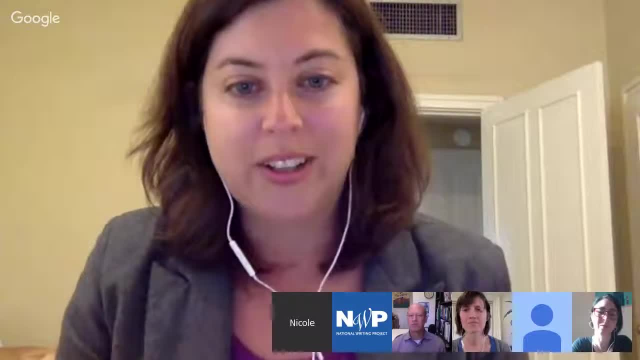 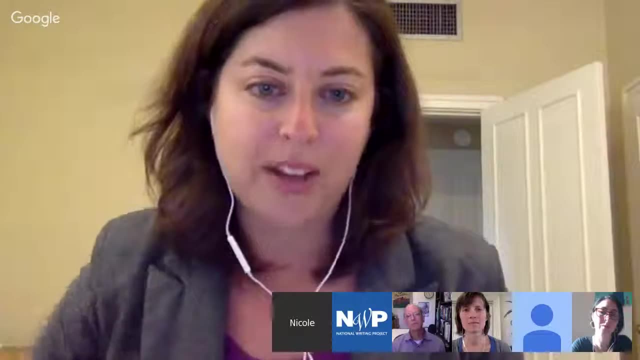 thought about a lot when it comes to the council, the council's work and the kind of education that it gave me in an informal space, that after I completed my doctorate and went back into classroom teaching, It definitely changed who I was as a teacher. 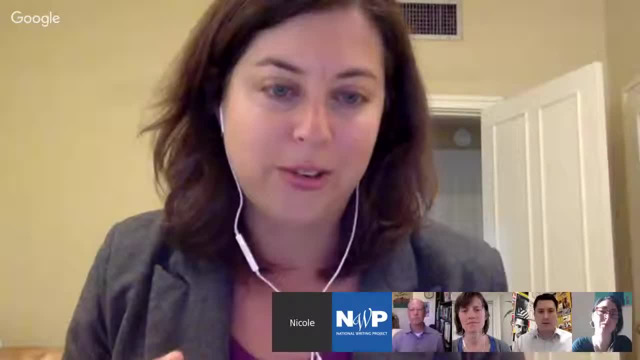 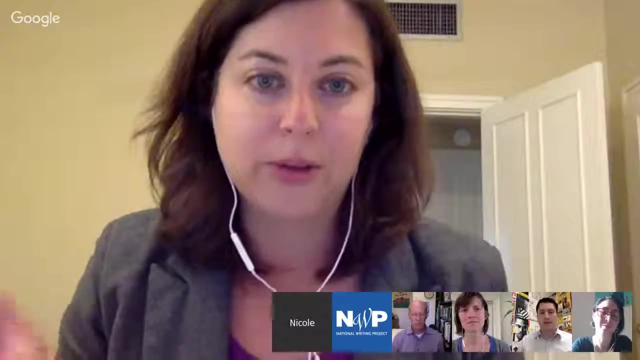 And it challenged me to bring the informal practice of YPAR into a formal classroom space. So I feel like the it can be done, like Eddie's saying, like having those experiences can then lead you back into the classroom in a powerful way.